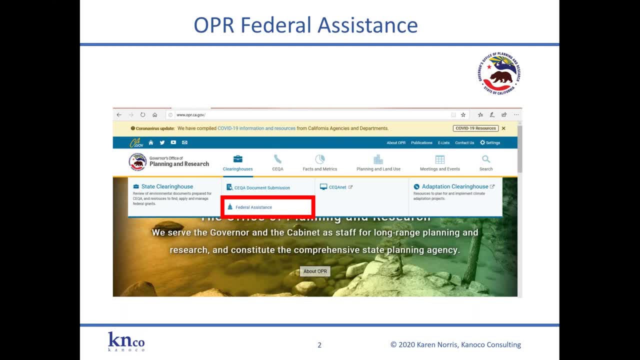 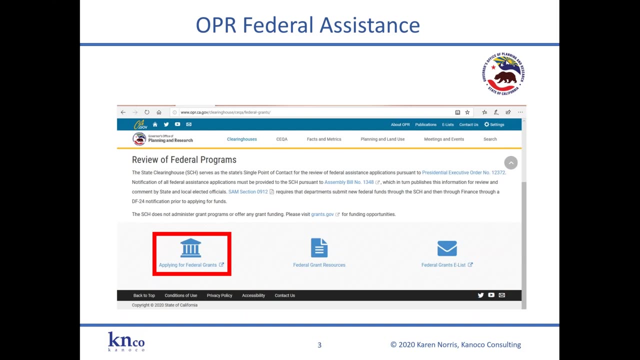 point of contact for the intergovernmental review of federal grant applications. You can find all of our resources for federal grants on the OPR homepage by hovering on clearinghouses and selecting federal assistance. The Applying for Federal Grants link is where you'll go when you're applying for a federal 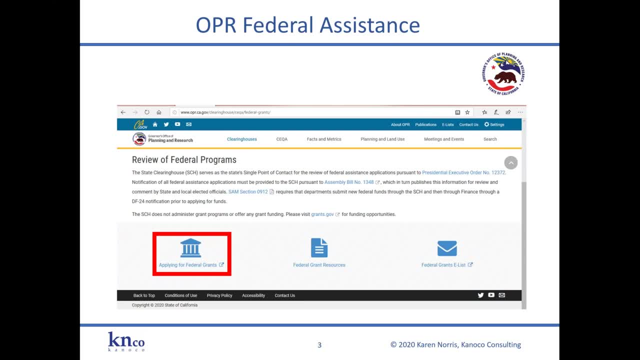 grant and need to submit notice of your application to comply with the Executive Order on Intergovernmental Review. All notices can be viewed on this page under the Submissions tab. The Federal Grants Resources link will take you to a library of resources to help you. 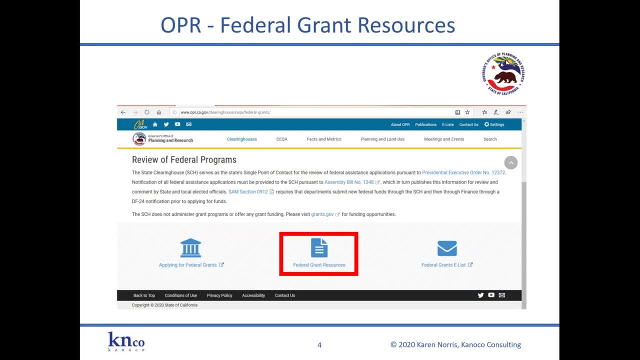 learn more about applying for and managing grants, and includes links to the grants pages of every federal agency. Last is our Federal Grants eList, which hopefully most of you already receive, but if not, you can sign up for it here. This weekly email provides updates on federal grant opportunities, news and trainings. 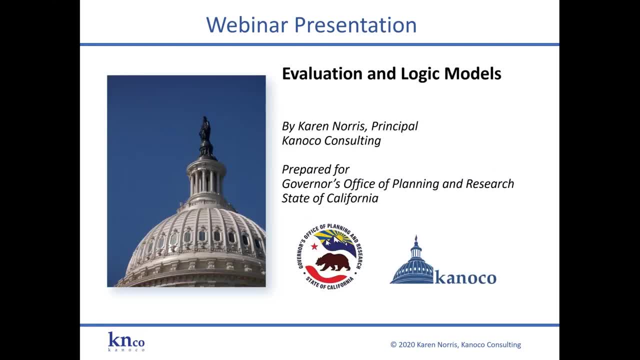 and events. And with that I'll turn things over to our presenter, Karen Norris. Karen is a nationally recognized expert in the grants community, based in the Washington DC area. She regularly presents at state and national conferences and has provided expert testimony to the Maryland. 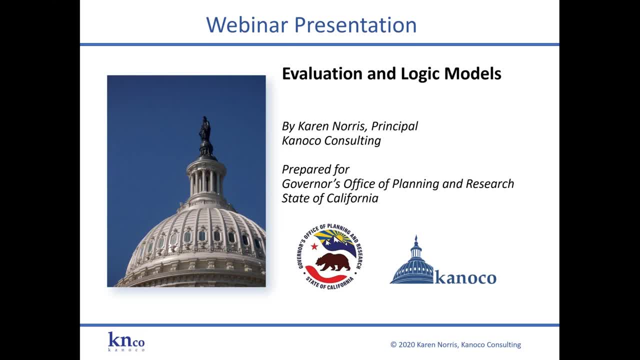 General Assembly. We're going to start a conversation with Karen. Thank you, Karen. Thank you, Amy, So I'm excited to be here with you this morning. My name is Karen Norris. I'm from the National Center for Finance and the United States Senate. 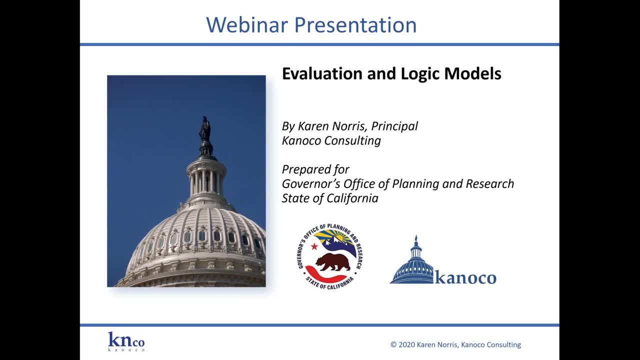 Subcommittee on Federal Financial Management About Grants And we're very pleased to have her here with us today. So thank you, Karen, Thanks Aimee, Appreciate that And good morning everyone. Welcome to Evaluation and Logic Models. I'm really glad you have some time in your schedules today to spend with us. 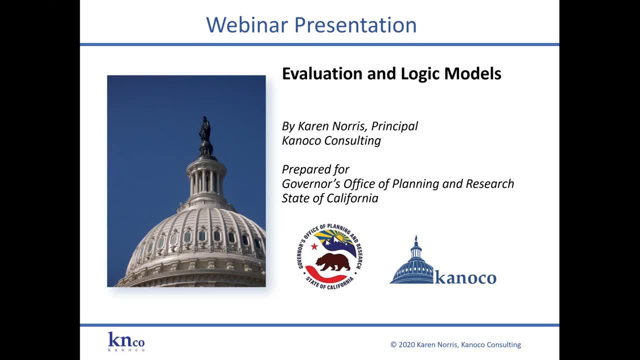 And I hope that the presentation is meaningful to you. Good morning. It seems in today's environment that more and more focus is being placed on performance and results, And the logic model is an interesting little tool that can be easily applied into the grants environment to help grant managers articulate performance and results and outcomes. 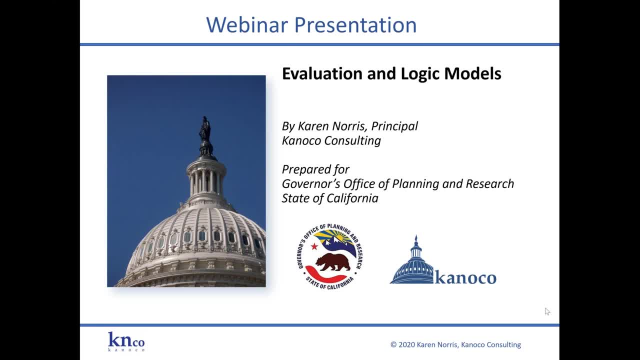 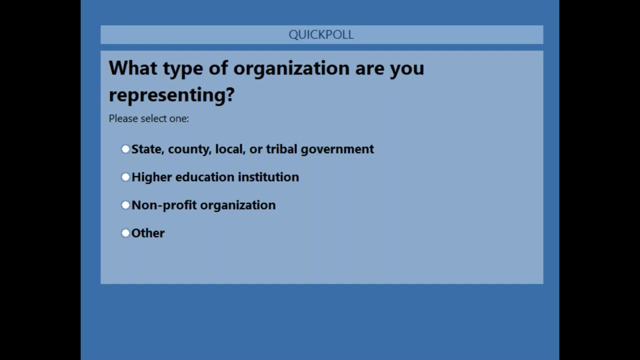 So let's get started Now. sometimes there's a little lag when I forward the slides, So let's see, Here we go. So, right before we start our presentation, go ahead and do us the kind favor and fill out the poll and let us know what type of organization you're representing. 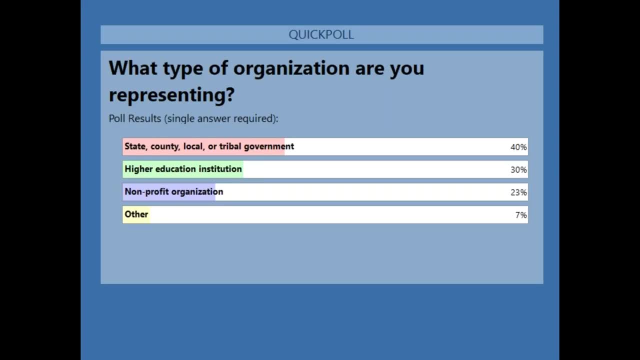 So great. So this is important: 40% of you are from state, county, local or tribal governments, which is wonderful. 30% from higher education, And higher education typically has not only program grants but research grants as well. 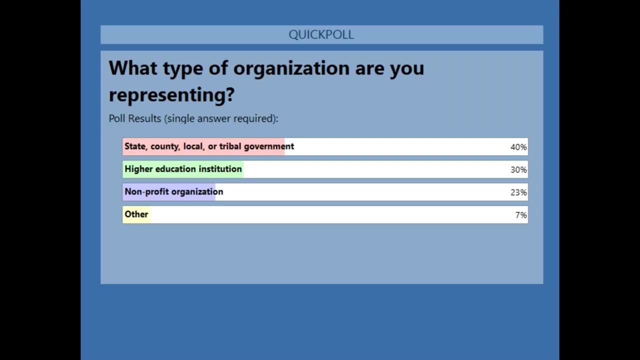 And the logic model will work with both types of programs. And 23% nonprofit organizations. And 70% of you are from state, county, local or tribal governments- So great. So this is important: 40% of you are from state, county, local or tribal governments, which is wonderful. 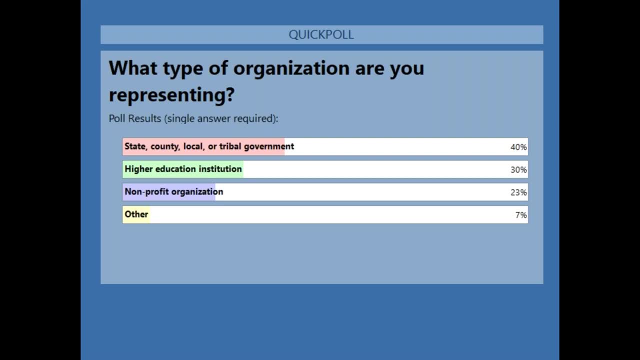 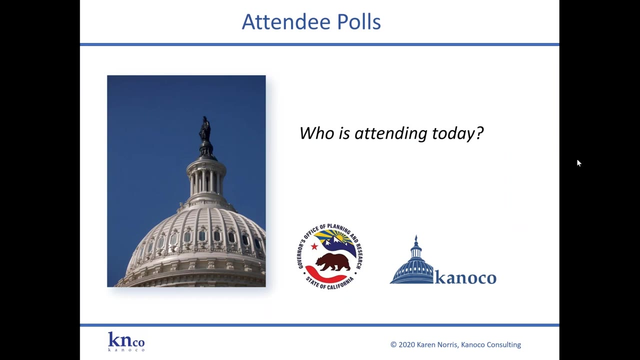 And 27% others. So you may be consultants, or you may be grant writers, or you may be policy folks or CPAs- It's everyone Welcome. We hope the webinar is helpful to all of you. Great, Now my next question is: how long have you worked with grants? 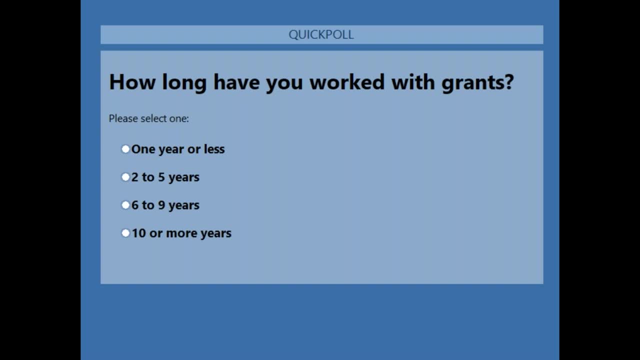 Great. Now my next question is: how long have you worked with grants? So, 13%, one year or less, That's a lot. Well, welcome. Welcome to the grant world. And I, you know I fell into grants by accident. I've yet to meet anyone, And I've been doing this for 30 years. 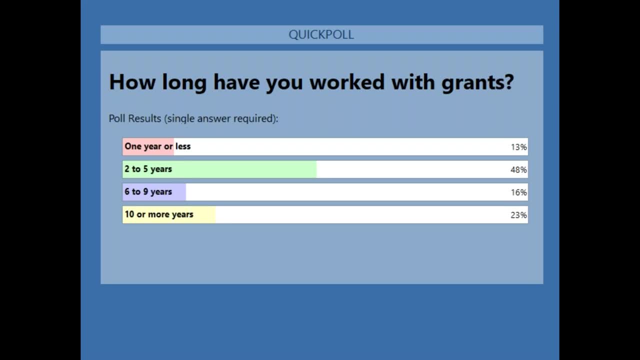 I'm an old person. I've yet to meet anyone who kind of started off in their career saying: I know what I want to do when I grow up. I want to be a grants person. So I just fell in love with the whole concept that the federal government makes money available to local communities, state local governments, nonprofits- so that they can go out and do good works in their communities. 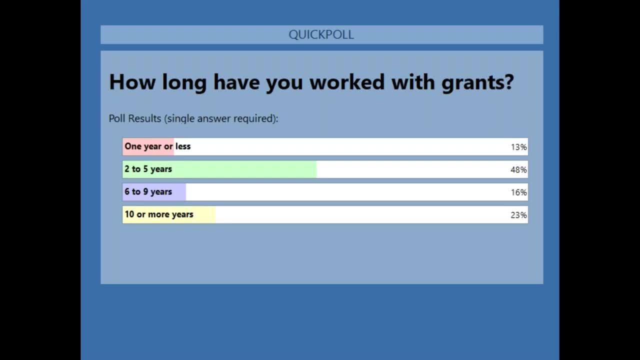 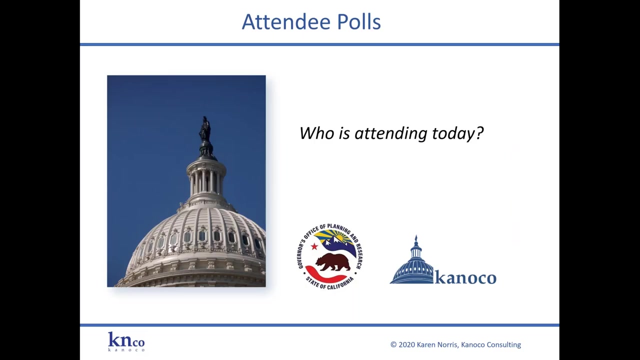 And I just think it's wonderful. So welcome to my new people. And two to five years- about half of us, Very good. Six to nine, And then 10 or more. Bravo for you guys for for hanging in there. So the reason I wanted to know how long you've been in grants is that we're currently operating under a set of guidelines called the uniform guidance. 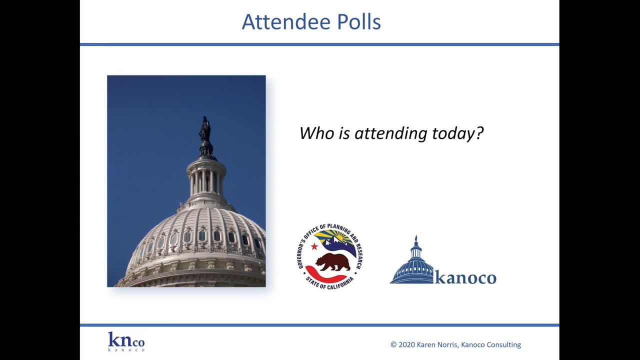 And this current set of guidelines became effective December 26. In 2014,. so if you've been working in grants for five years or less, you only know the uniform guidance. You don't know what was used prior to that. And that's not such a bad thing, because you didn't have to unlearn bad habits. 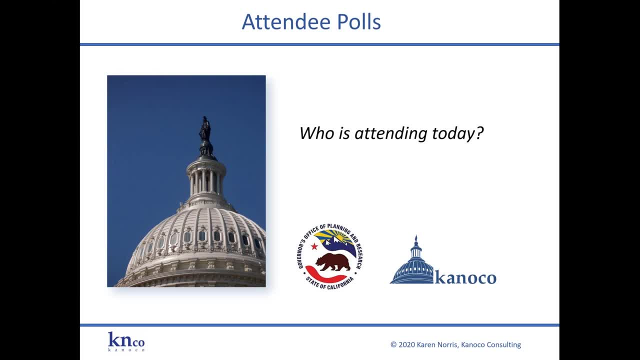 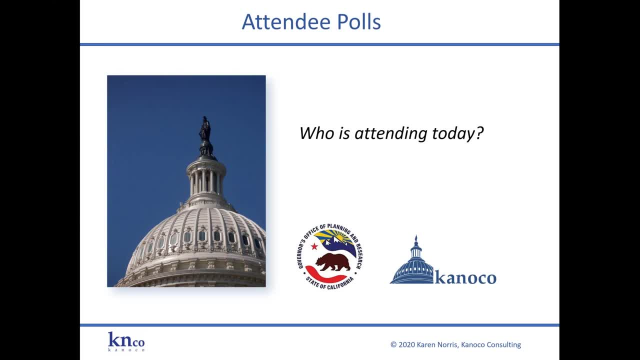 And when the uniform guidance went live, it sounded the same. You know, a lot of the words were the same: pre award, post award, audit. you know, indirect costs: the word sounded the same but it's written very differently And the uniform guidance is very much focused on performance. 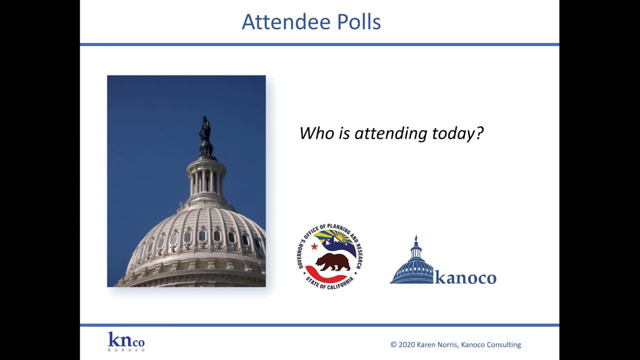 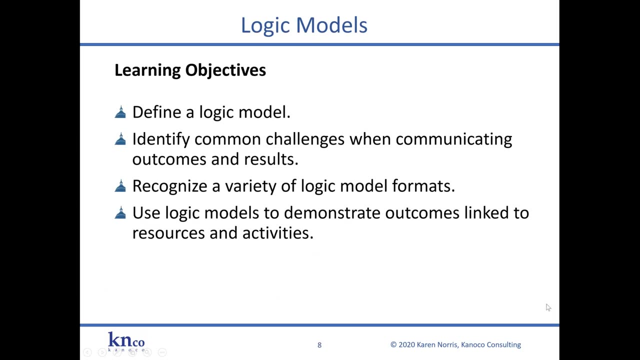 And whether or not you want to get funded or not, the individual, the non-federal entities who receive the funding, whether or not they're, they're not only complying, but they're also performing so great. so I'm trying to advance the slide, so it's ah, here we go. 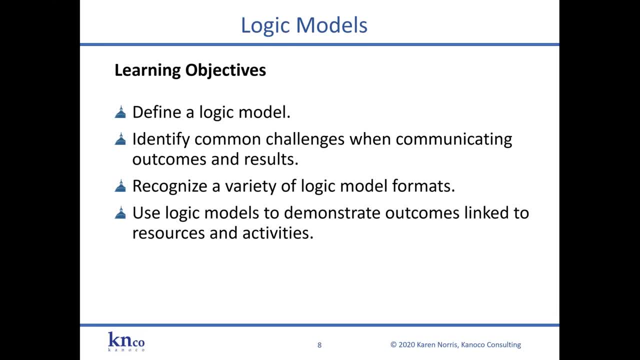 Bravo, the slide moved. so our learning objectives: first of all, we're going to define what this logic model is, and then, for the second learning objective, we're going to just talk in general about: well, what are some of the challenges when we need to communicate outcomes and results? what is it that that is important to say? 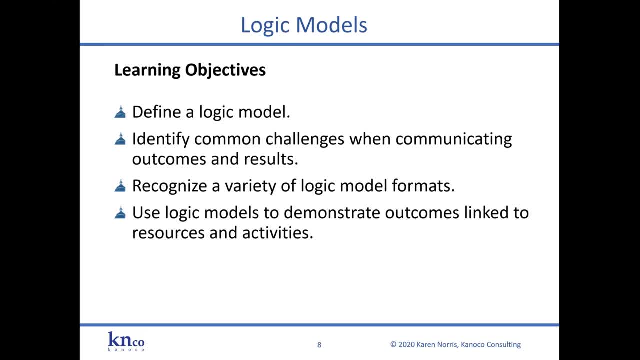 or not important to say, or what is it that gives some, you know, gives us some difficulty. so we'll talk philosophically about some, just the the best way to communicate outcomes and results, and then we're going to start to get into using logic models. so the third learning objective will be: well, there's a variety of 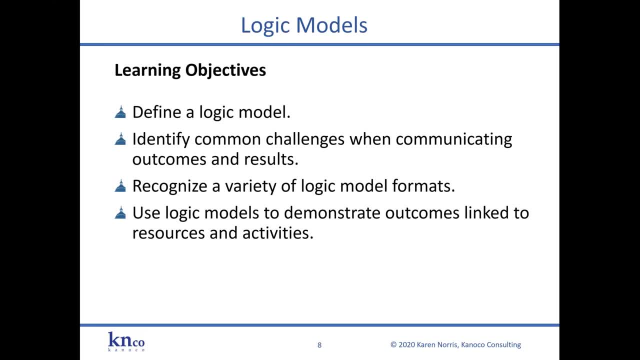 different formats and one format might be a little bit better than than another one for your particular organization or your particular program. and then it also, you know, lets you know that well, you can kind of modify and make up your own logic model format, as long as it includes some basic, some basic concepts. so we'll talk. 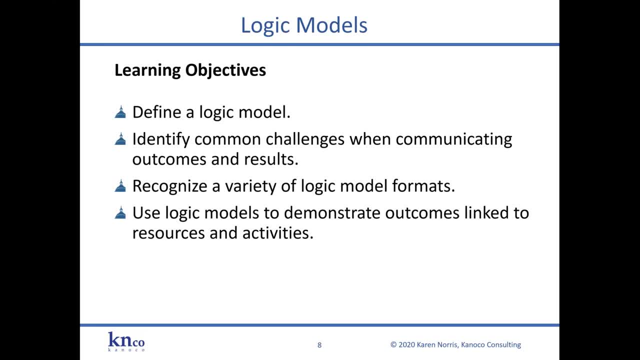 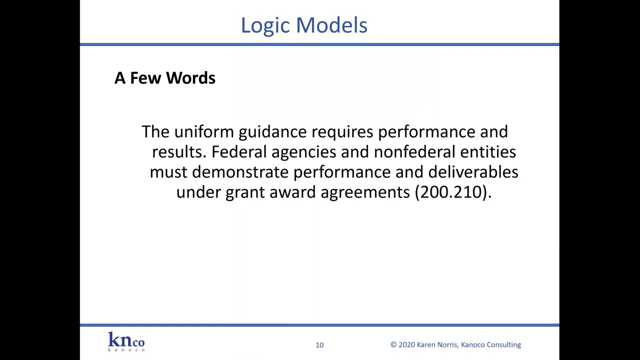 about that. and then the last bullet: we're actually going to give you some samples of objectives, excuse me, and how we use them, and and logic models, so hopefully that that will make it seem a little bit more real. so a few words. the uniform guidance requires performance and results as a matter of 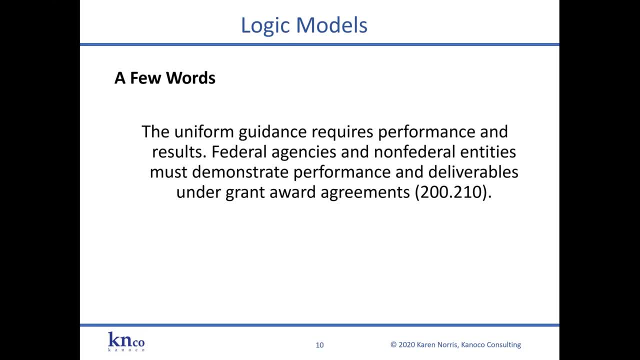 fact, the president's management agenda has about a dozen what they call cap goals, CAP cross-agency priority goals. there about about a dozen of them, and goal number eight is is specific to the grants community and it's based on results oriented outcomes for for grants and 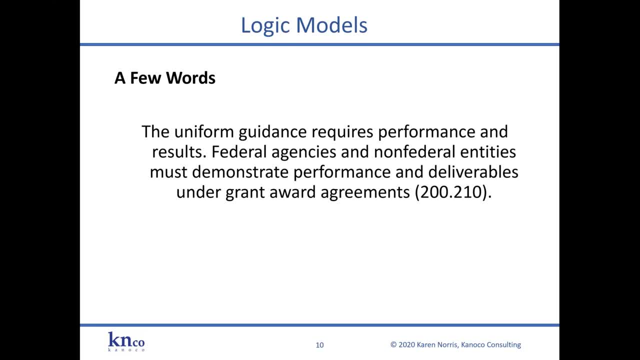 the president's management agenda issues progress reports every quarter and the most recent progress report, which was released in April and is posted on wwwperformancegov, is exactly about this topic. it's about grants and it's about results and managing grants for outcomes and results. so I've gone ahead and gotten a copy of that report and 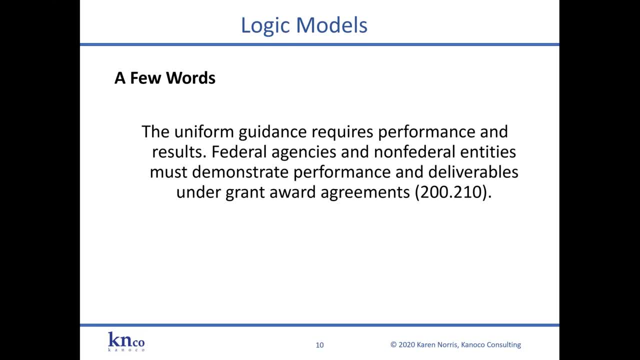 shared it with Amy and she's posting it to the governor's office website so everyone can have access to that report, which, which is really quite remarkable that you know just a sense of timing. so federal agencies and non-federal entities must demonstrate performance and deliverables under grant award agreements. 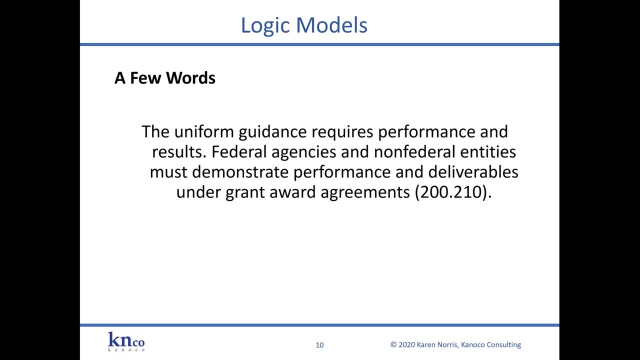 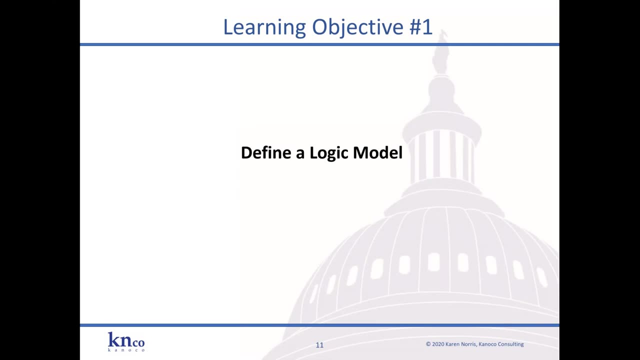 and that citation number is from the uniform guidance. two hundred point two ten, and that is the provision number that explains what must be included, what information must be included in an award document. so let's start learning objective number one and we're going to define the logic model and, in general, 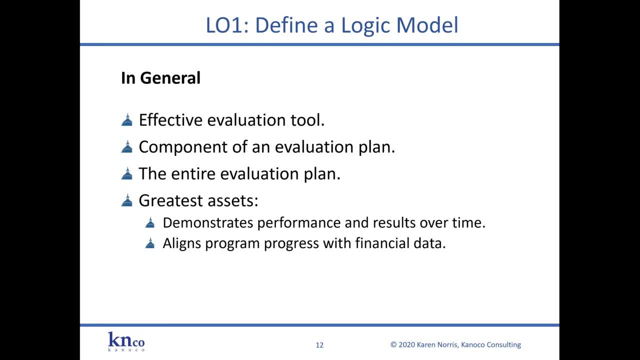 it's. it's a very effective evaluation tool. now it can be a component of an evaluation plan or just an evaluation kind of evaluation plan, but we definitely have to assess theravel for the groups and then we determine which whole data group can be a part of the evaluation plan, for example, if either communities have a significant number and industry accommodation. Eastern Jonah gap- wonderful, ever. so. it talks about that in the Tangent원 response book: zero population 합니다. loış kurešlettÁ- 991 beráćaa kureśte. råan circuit, Oak Wake, собак bomby og lea 2020. 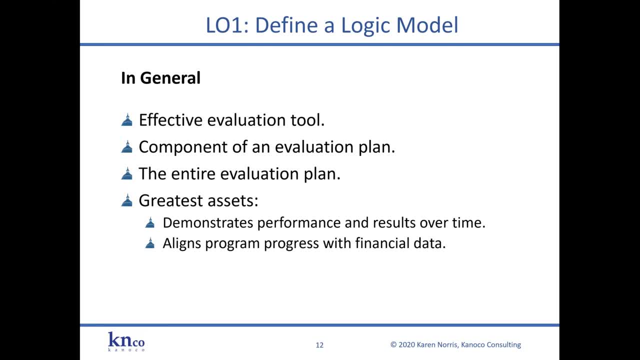 could be. the entire evaluation plan could be built around this logic model format. the greatest assets of this plan is that it demonstrates performance and results over time, and it also aligns program progress with the financial data and under the uniform guidance that's. another requirement is that grant. 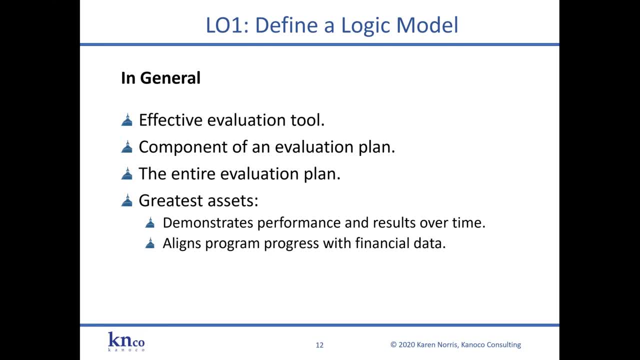 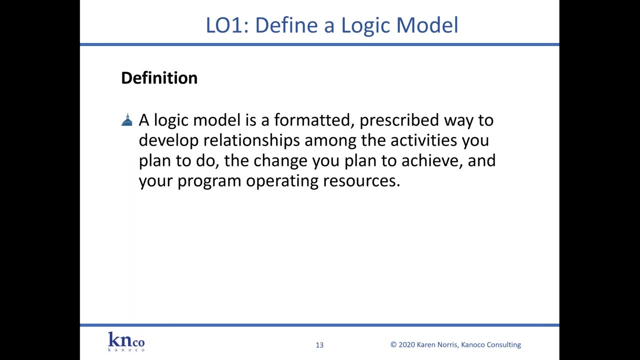 managers must be able to tie their resources, the funding that they use, to the activities that they're they're performing under their program. so a logic model is a formatted, prescribed way to develop relationships among the activities you plan to do, the change you plan to achieve and your program. 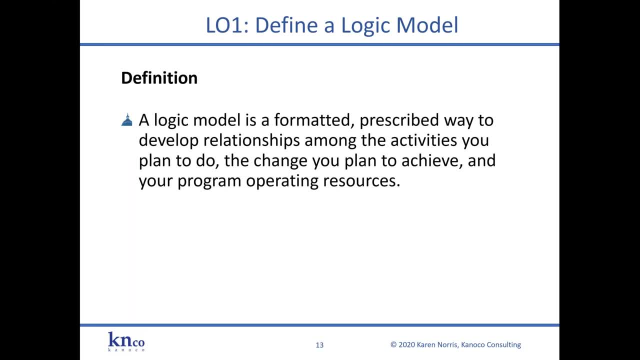 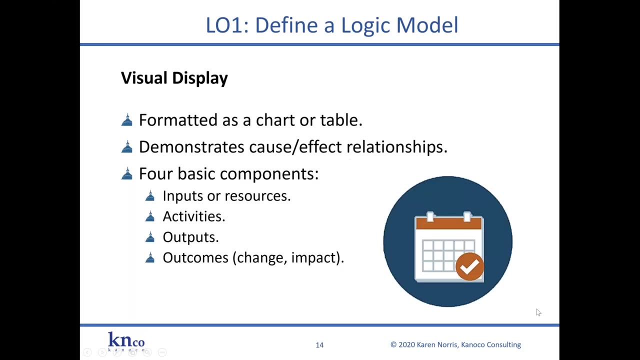 operating resources. so it's very important to be able to tie their resources to the program. so the logic model is a formatted and it it shows causal data, causal relationships. if I receive this money, what will I have to show for it? so the format is usually in a chart or a table and my preference is 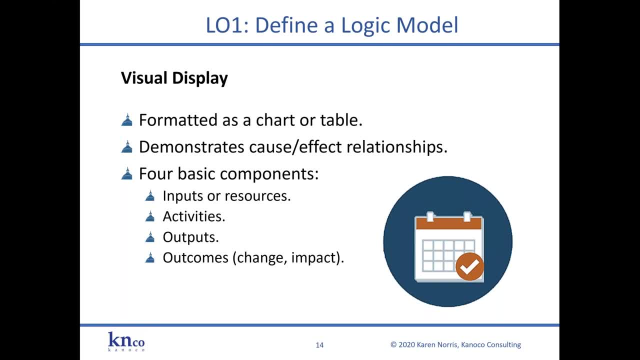 to use the table format, column a, columns tables with columns rates, cause-effect relationships. and here are the four basic components. no matter what kind of a visual display you use, the, you need to include your inputs or your resources, like like the award amount, the funding that you receive from. 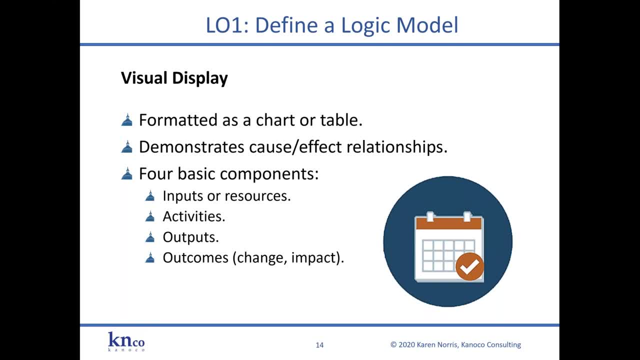 your award, then with that funding, what activities are you going to do under the grant program? and then we have outputs and outcomes, and those are the two that are the most difficult to explain. the difference- I mean the money, the resource- is kind of obvious. the activities that you're doing, that's kind. 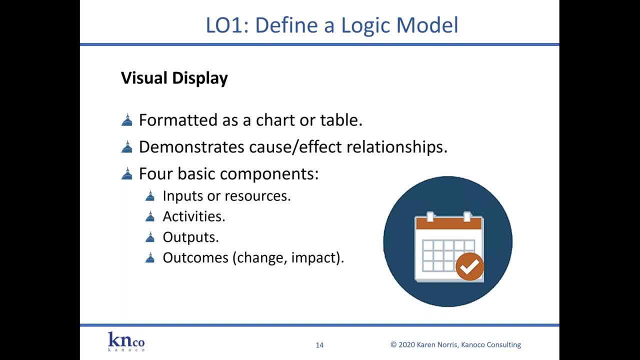 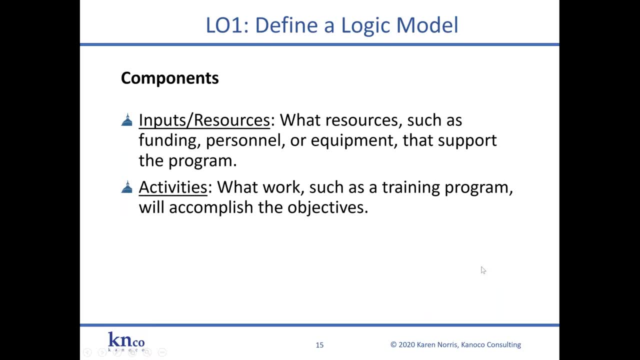 of obvious. but just what? what is an output and how is it different from an outcome? so we'll talk about that. so your endpoints are: your resources are exactly what? what funding percent, personnel, equipment, what you know, are you using? do you have a computer lab, internet connectivity? whatever it is that you're using in order to implement? 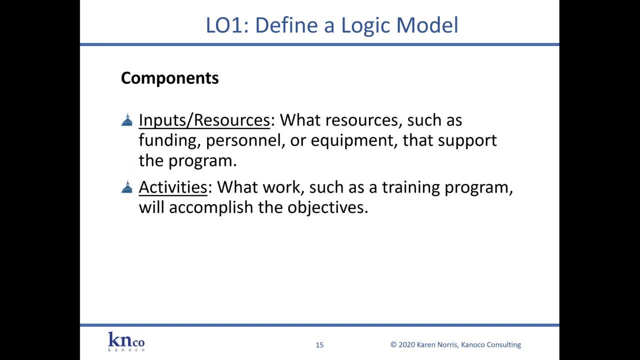 the program that would go into the inputs or resources column. and then your activities will. what works, such as a training program that you might be delivering. what will accomplish the objectives? and again, in your proposal you will have had objectives or you would have made promises. if we receive the federal funding or federal 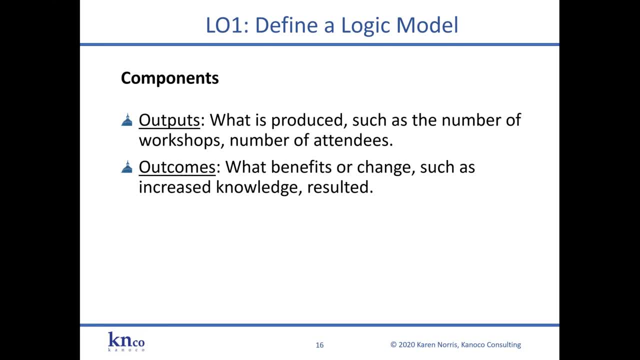 the estate funding. this is what we promised these. this is what we plan to do with the money and what we hope to achieve. so now, an output is a number, it's something. its productivity, it's something that's produced, such as the number of your workshops, or the number of attendees, or the number of hours spent. 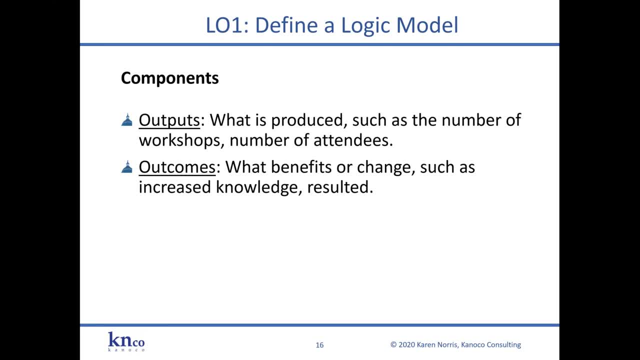 volunteering. it's a number of hours that you're spending as a volunteer on a certain project. it outputs are generally productivity data and then outcomes- is what the benefit or the changes, such as increased knowledge or results? so let's say you're driving down the road in a car, in your car, and you and you stop at a traffic. 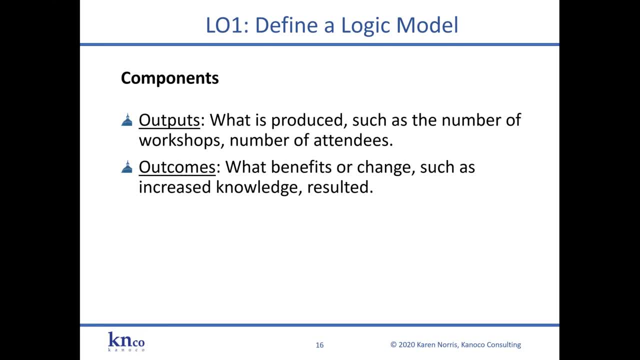 light and your car. you know, all of a sudden you press on the brake and you hear this squeaking and you go: oh, my brakes are making a noise, maybe they're wearing out, maybe I need new brakes. I better take the car in to the shop before it gets worse, because I don't want the brakes to wear down and then. 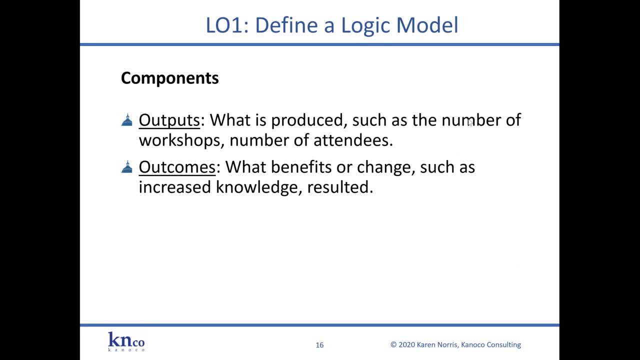 I've got a problem with my brake drum and that's going to be even more expensive. so it's does sound like I'm talking from experience. so here you take your car into the and you're speaking to the mechanic and say, yeah, my group, you know, I hear a. 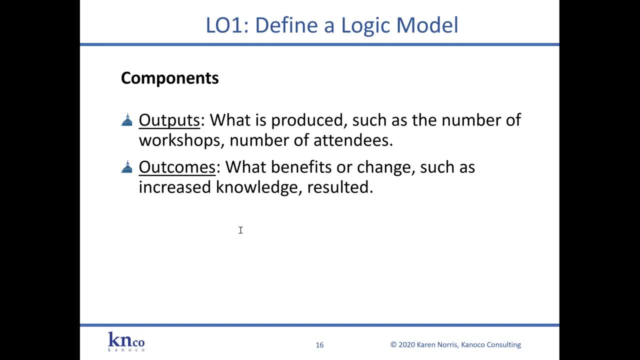 noise when I press on the brakes. I think my brakes might be. oh, maybe I need new brakes, and so the mechanic goes: no problem, we'll take a look at it, and it's gonna cost you four hundred and fifty dollars, or whatever it is, and you sign. 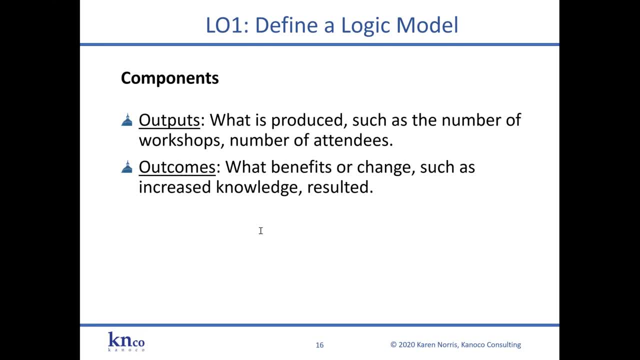 you know, on the estimate, okay, I promise to pay, kind of thing, and you drop off the car and you come back and and here it is and you pay for it and you get in the car and it's it's squeaky again. it's still making that. 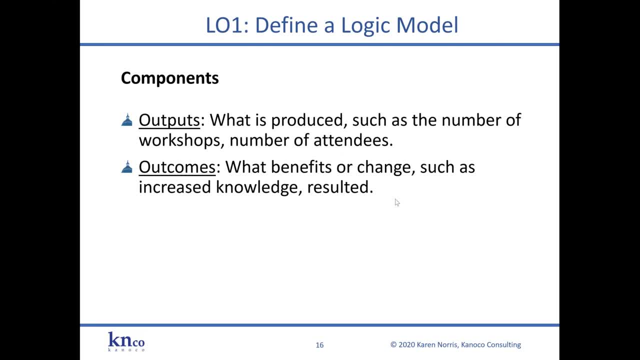 noise. so back into the mechanic. you know what happened. I expected to see a change, I expected to give you this money, I expected a benefit. my outcomes right. did you or didn't you fix the brakes and the guys go? well, we had two guys working on it and it's 50 a dollars an hour and they spent four hours, you know working. 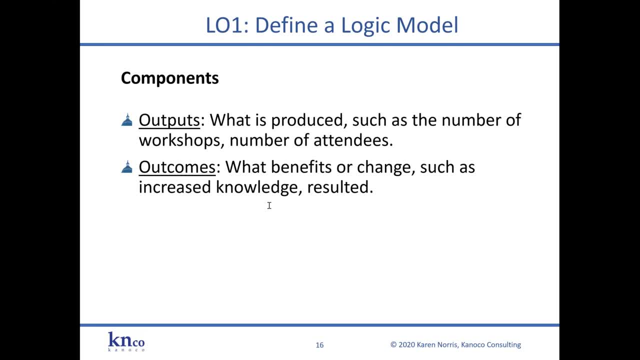 on the breaks and I said, yeah, but that's what you produce, That's the number of hours and the number of people working on it, and that's all fine and good and I'm glad that you know they were working on it, but I still have the same problem: I don't have change. so that's the. 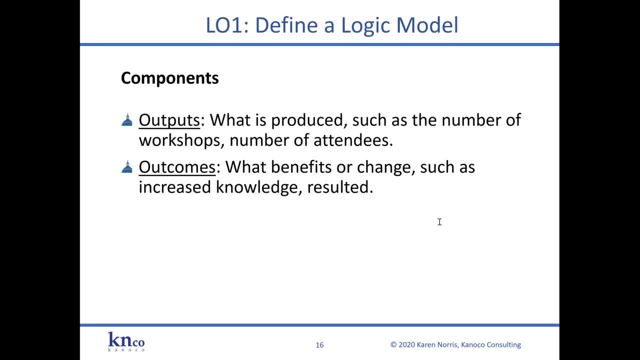 difference between an output and an outcome, and a lot of people think that output is what you the end result. We had so many numbers, so many workshops. We had five workshops and 30 people attended each workshop. so by the end of the program, by the end of the grant project, we were 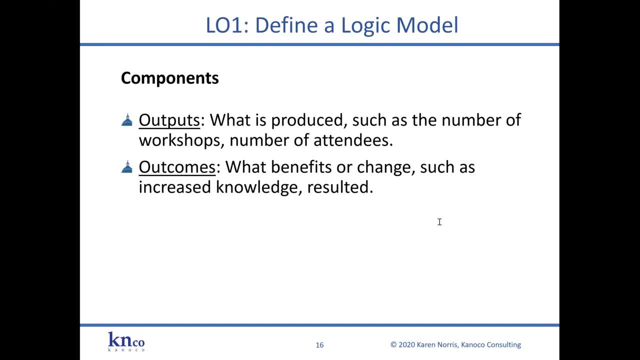 trained 150 people, and you know they think that that's the end point, but that is not. That's almost there, but not quite. That's the productivity that took place under the grant. but what was the result? What was the whole purpose? 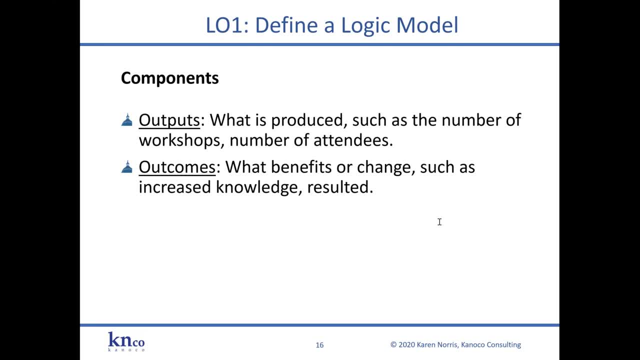 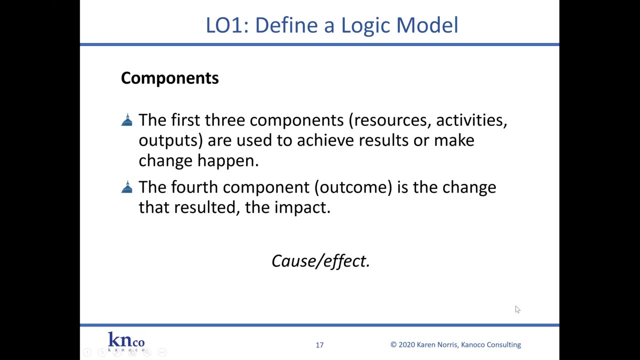 What was the purpose of training the people? What benefit did they receive as a result of taking that workshop? So big difference between outputs and outcomes? okay, We will have a question and answer period at the end of, in case you want a little bit. 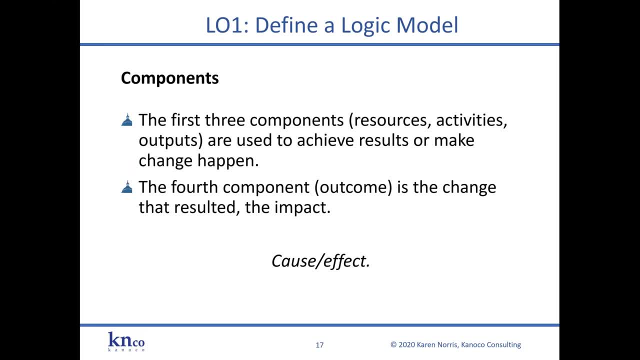 more clarification or you have a question. So the first three components of the logic model, your first three columns, you know if you're using the column view is you have resources, activities and outputs and these are used to achieve the results or to make change happen. 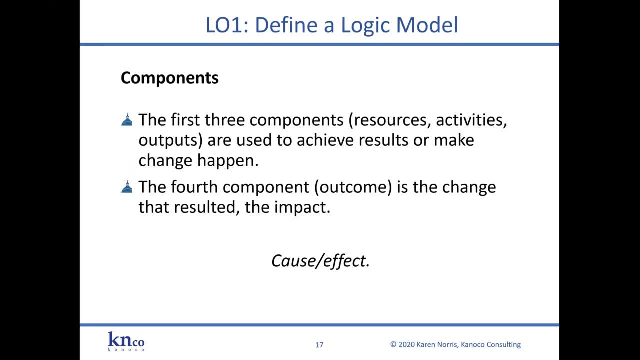 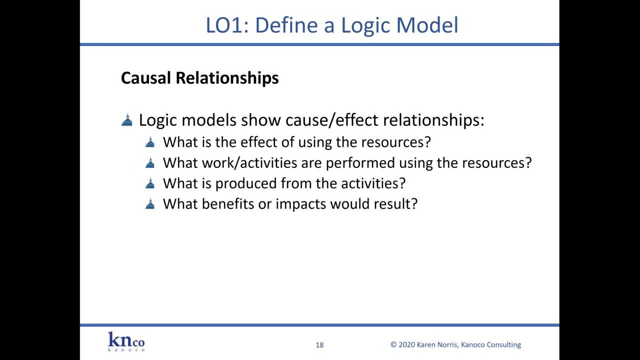 the outcomes. So the fourth component: the outcome is the change that resulted, the impact. and so there's your cause and effect. So here, cause and effect relationships are, you know, just the basic, the basic philosophy of using a logic model. So what is the effect of using the resources If we, if we make you? 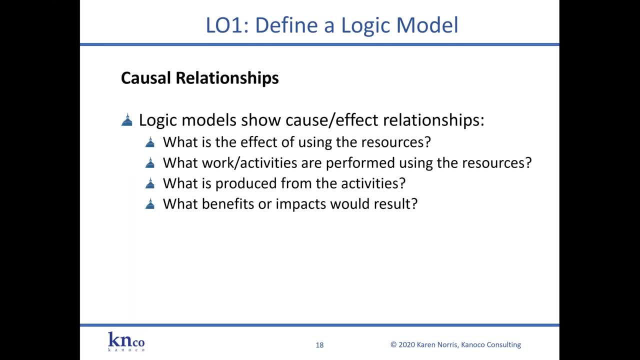 if the awarding agency says: okay, you've submitted a proposal, you've made some promises to perform. if we make you the award, if we give you the money, what is the effect? Are you, do you have the capacity to make sure that you achieve your promised results? And then, how are you going? 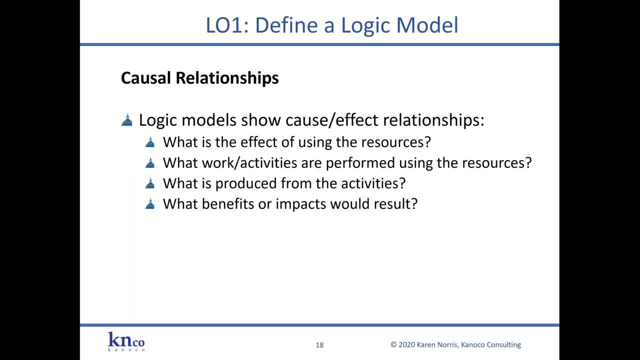 to do it? What work or what activities are you going to, are going to be performed using those resources? And after you do the work and you conduct your activities, what have you produced? There's your number, your productivity number, your outputs, And then, from all of that, 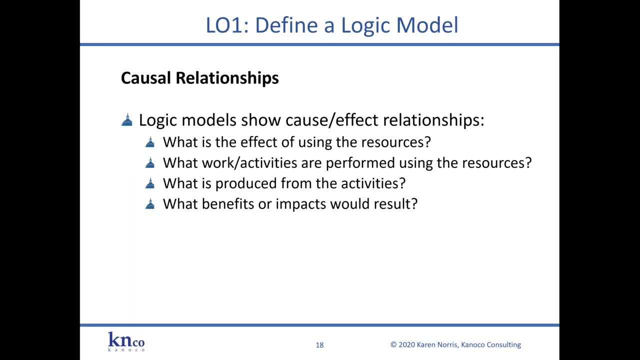 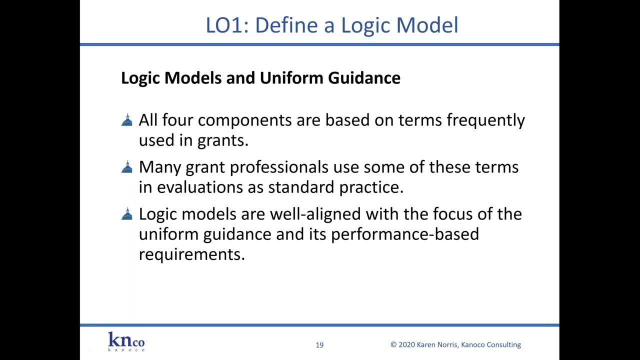 what's the lasting benefit, And it would be nice if the change would be lasting change, something that's sustainable. So there's your cause-effect relationships. So all four of these components are based on terms that are frequently used in grants, which is one of the reasons the logic model is is so practical when it's applied. 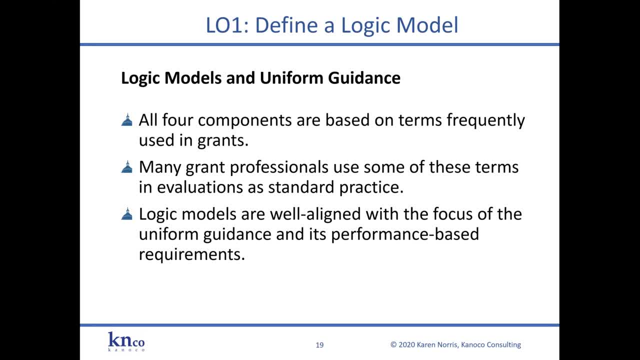 to a grant project. Many grant professionals use some of these terms in evaluations as a standard practice. Logic models are well aligned with the focus of the uniform guidance and its performance-based requirements. Without a doubt, it's one of the reasons I like this little tool so much. 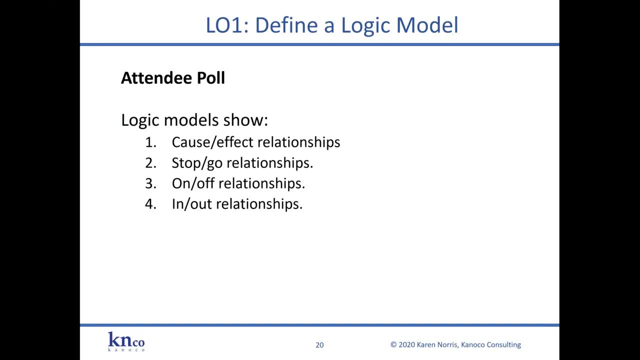 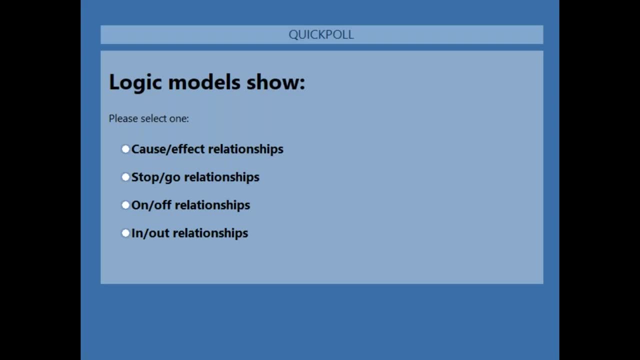 So here we have a poll. Amy, are you able to put the poll up on the screen? Yeah, I'm able to put it up. Yay, Amy. So please select one of the following Now click through. select something even if you're not sure. 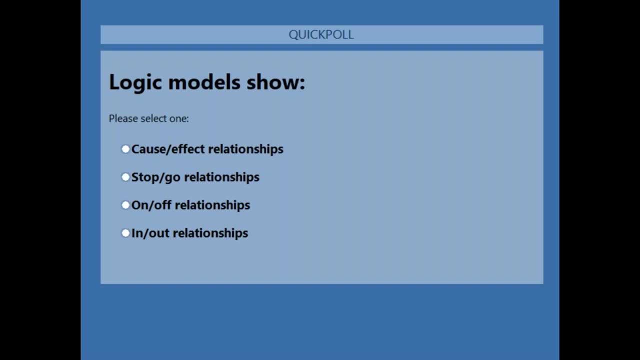 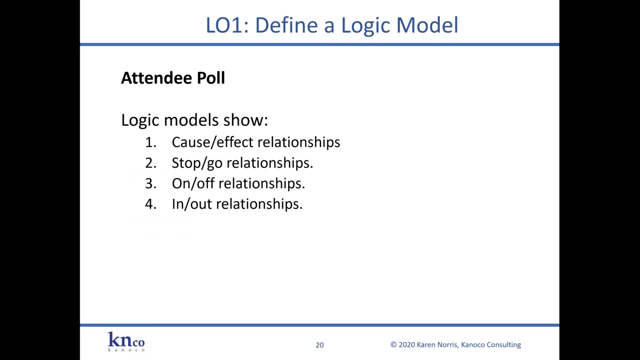 We want to see the click-throughs so that we know you're watching, And so would the logic model show cause-effect relationships, stop-go relationships, on-off. Well, look at you guys. brilliant, 100% of you get it. It's cause and effect Awesome. 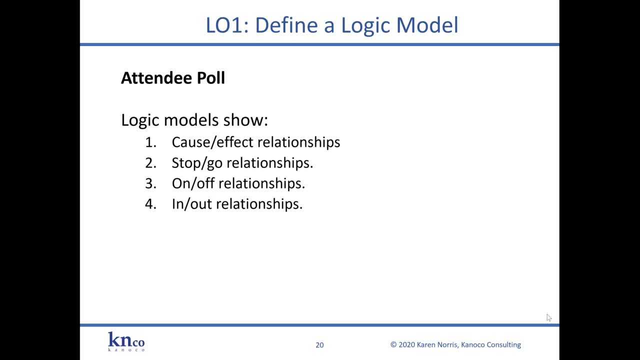 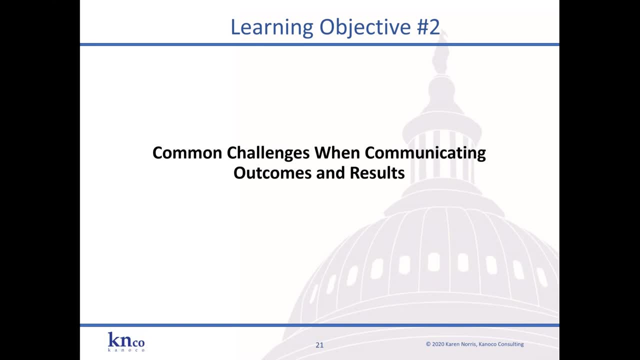 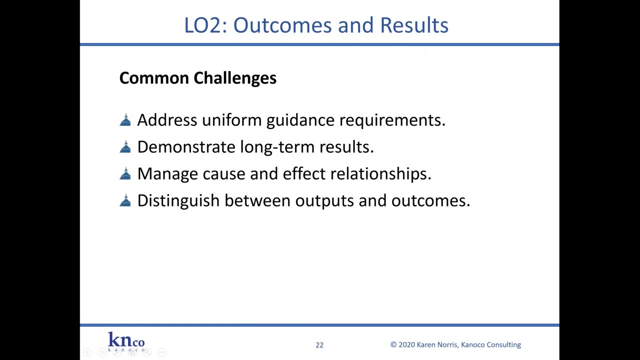 Yay. So what is the challenge? What are some of the difficulties that we have to cope with when we're trying to communicate outcomes and results? Well, first of all, we have to address the uniform guidance requirements, And the uniform guidance has an expectation that there will be. 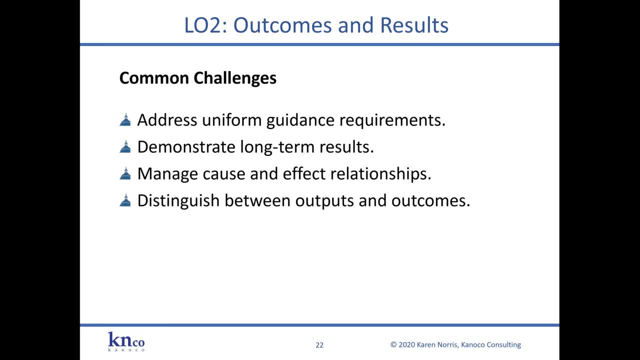 deliverables. there will be performance, there will be results, And so we have to address the results. You will have reduced risk. You'll provide good stewardship of federal funds. We have to address the uniform guidance requirements And the logic model really does that. 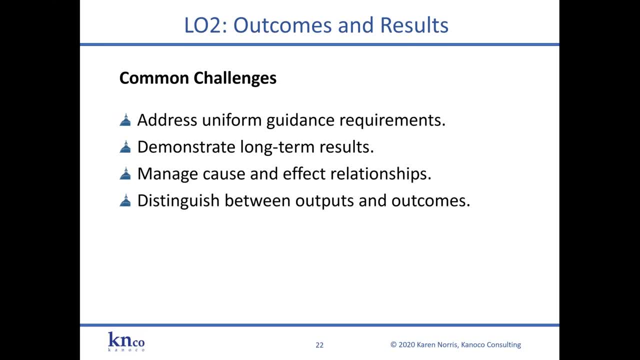 It's hard to demonstrate long-term results, particularly if you have a one-year grant program. You know 12 months and you're done And anything long-term is going to happen. but you're in a position that you really hope to finish this grant and then you get the 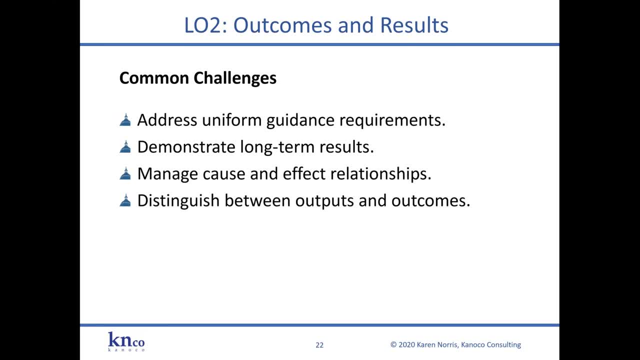 confirmation that the grants are complete And you really can't commit your organization to anything once that grant is over. So how can you reflect the possibility that there's some lasting change, not just short-term change? And the logic models can help lead you to that conclusion. 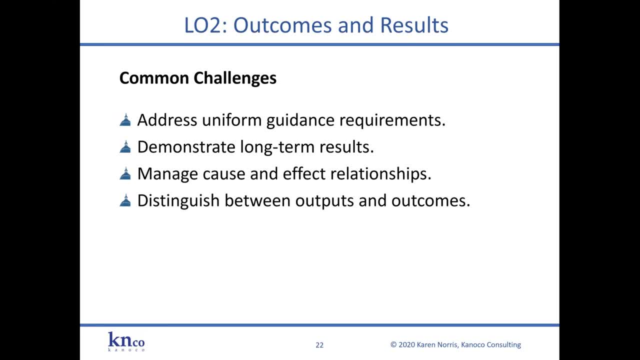 Managing cause-and-effect relationships. we have the funding, we did the activity. what's the result? Logic models can help you articulate that and then they can help you really articulate between outputs and outcomes, which I think sets your evaluation, your evaluation report, a step above anyone else. 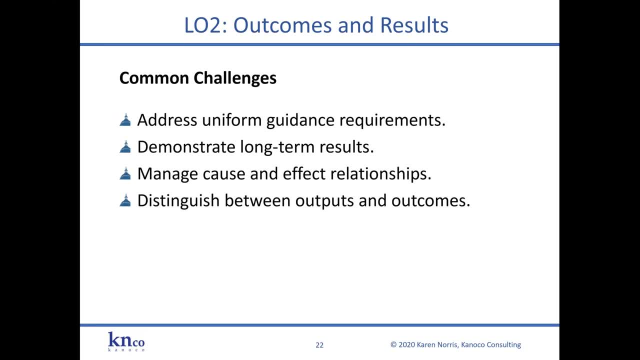 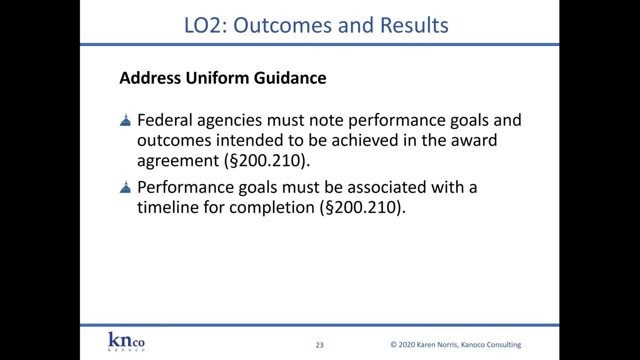 who doesn't know the difference between those two terms and cannot articulate the difference. So let's talk about the Uniform Guidance requirements first. Well, federal agencies must note performance goals and outcomes that are intended to be achieved in the award agreement, and there's that same provision 200.210,. 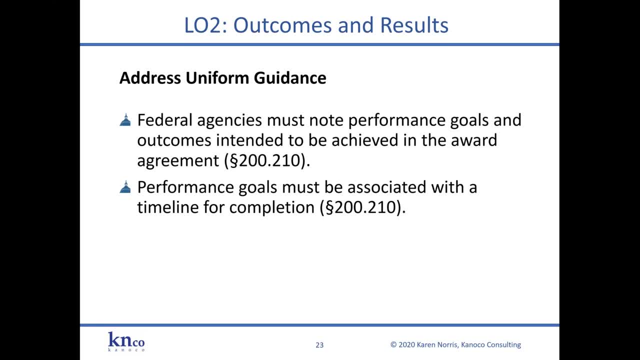 in the Uniform Guidance, in case you want to share that with your grant teams back at your organization and you want to get the source language instead of just relying on my paraphrasing. And then performance goals must be associated with a timeline for completion, and that's in the same provision. 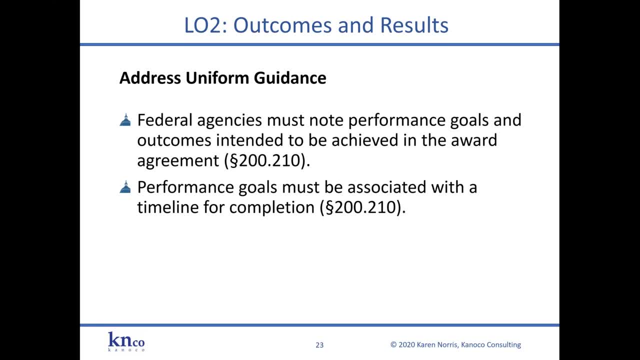 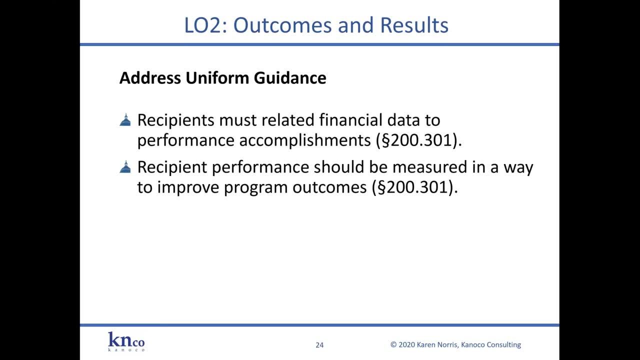 And that timeline for completion is something new under the Uniform Guidance. That focus wasn't quite there. under the old circulars Recipients must relate financial data to performance accomplishments and 200.301 is the requirement in the Uniform Guidance. that states that. 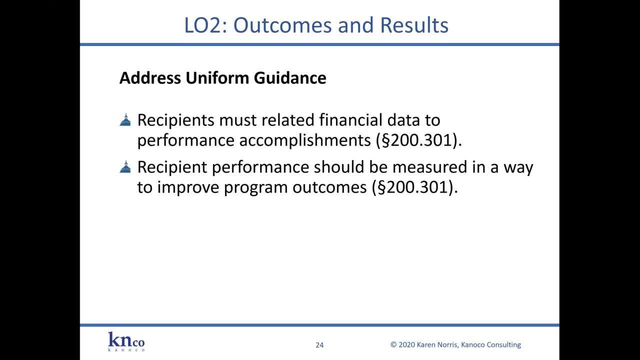 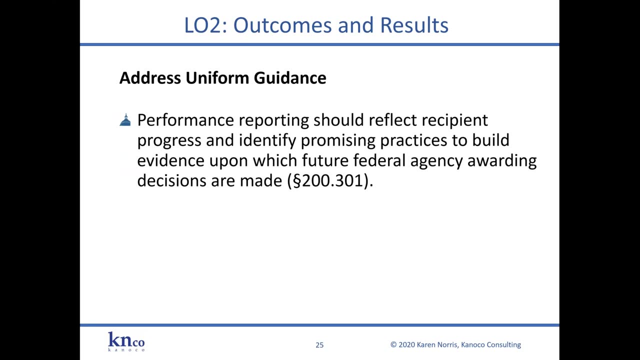 And in the same provision, recipient performance should be measured in a way to improve program outcomes, And that's again the focus on an outcome. This is an important provision. It sets the stage for several things. 200.301.. A 300 number in the Uniform Guidance. 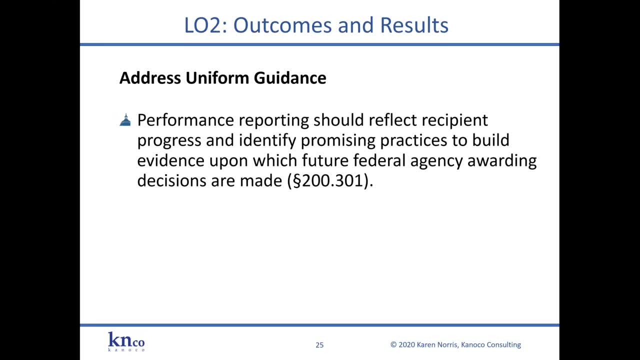 is in the post-awarding section where a 200.301 is the number in the post-awarding section, A 200 number like 200.210, that's in the pre-award section. So you see evaluation, you know. 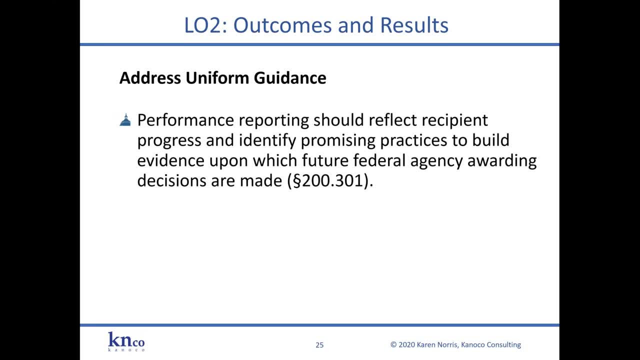 encompasses the full breadth of the grant life cycle: pre-award, post-award reporting, even audit. So performance reporting should reflect the recipient progress and identify promising practices to build evidence upon which future federal awarding decisions are made. So you know your evaluation. 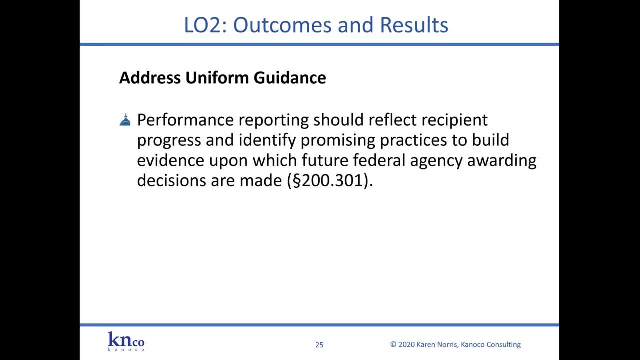 and how you articulate your results and the fact that you're able to think in terms of outcomes and you achieve your outcomes. that affects future awards. It means that your program could be replicated as a successful practice, as a best practice to use everywhere. 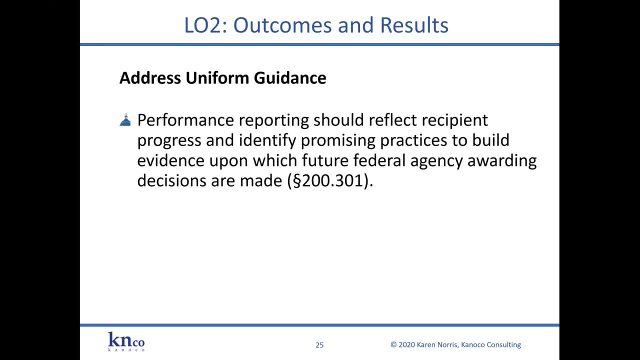 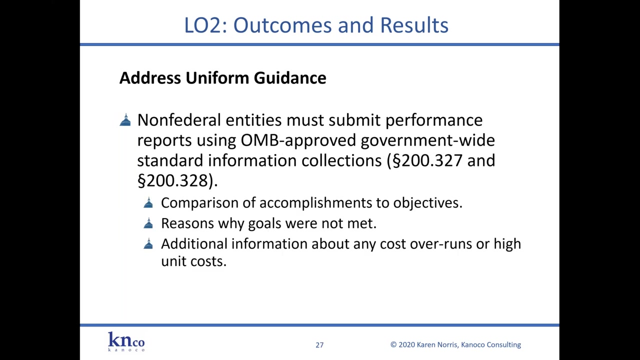 And it heightens the interest of awarding agencies in the type of work that you're doing. Non-federal entities must monitor activities under federal awards to assure compliance and performance expectations are being achieved, And that's under 200.328.. Non-federal entities must submit performance reports. 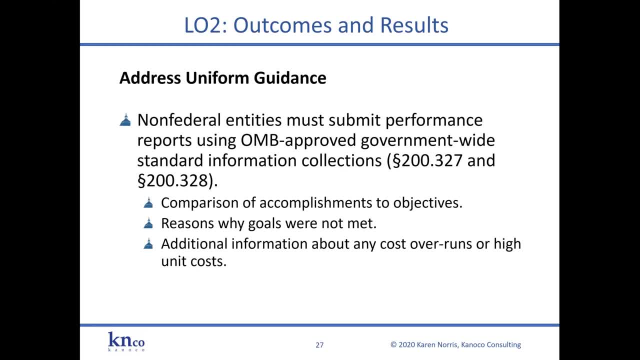 using OMB-approved government-wide standard information collections. Now that's usually standard federal forms like the RPPR. That's for the research progress report, That's reporting. my folks from the universities in class today are probably familiar with that progress report. 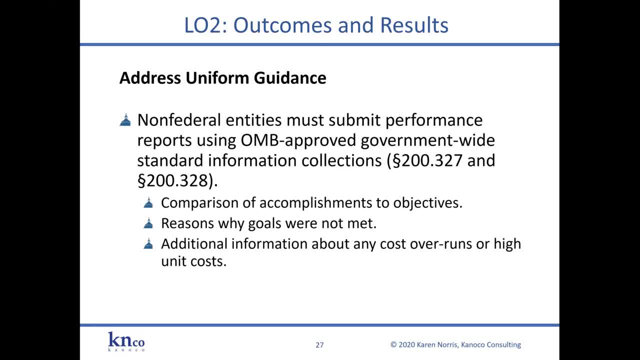 But 200.328 in the uniform guidance is the provision for progress reporting And 200.327 in the uniform guidance is the provision for financial reporting And for those of you who are working on the financial side of things, you may have filled out a standard form 425,. 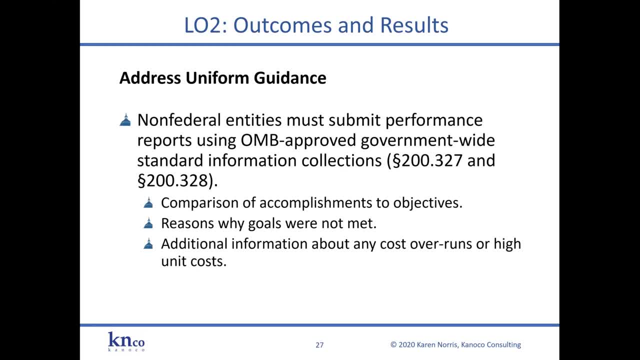 which is the federal financial report, And that's under 200.328.. And again, the logic model helps tie what you've spent to what activities, what work you've done And the types of things they're looking at and reporting is they want to compare your accomplishments. 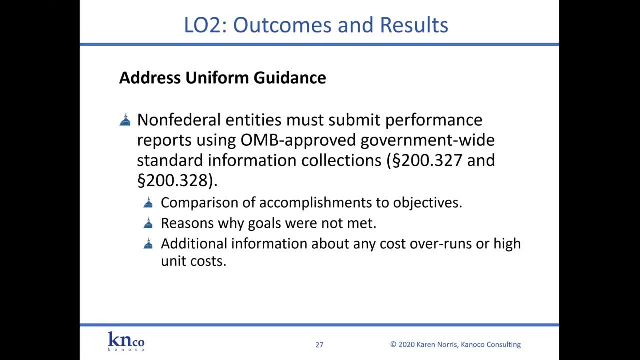 to the objectives that you promised in the proposal. If there was an issue, any reasons why your goals were not met and additional information about any cost overruns or high unit costs. I know that when I worked in the field, I was in education. 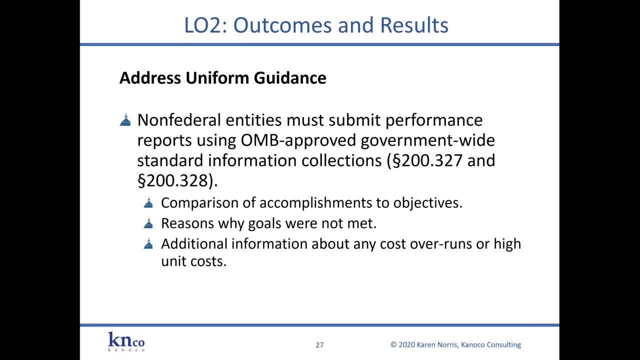 And when I worked with my institution's higher ed, my faculty members who were submitting research grants always wanted to buy some fancy schmancy piece of equipment. It cost a lot of money, You know- and they were gonna use the research grant to help them purchase that equipment. 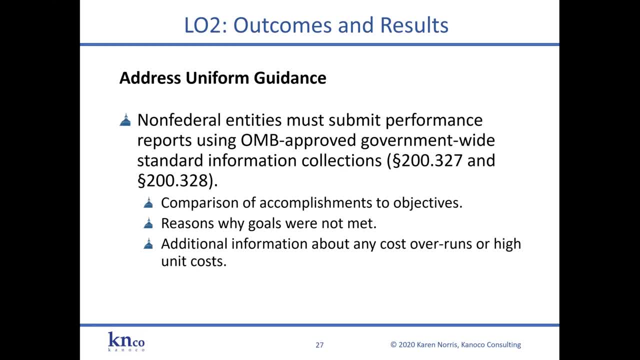 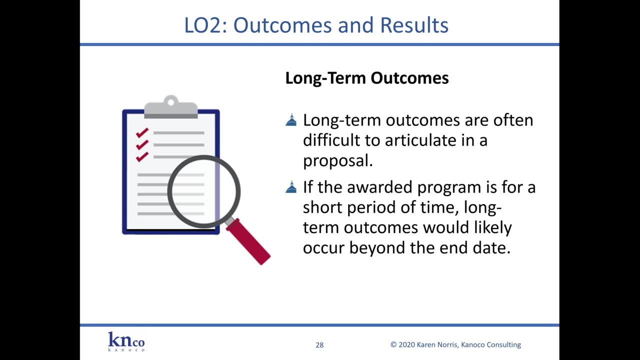 and then they could conduct research. So we would always have to explain why we had a high unit cost for that particular research item. I mean, they wanted the flux capacitor right. So long-term outcomes- those are always hard to demonstrate because they tend to happen once the program is over. 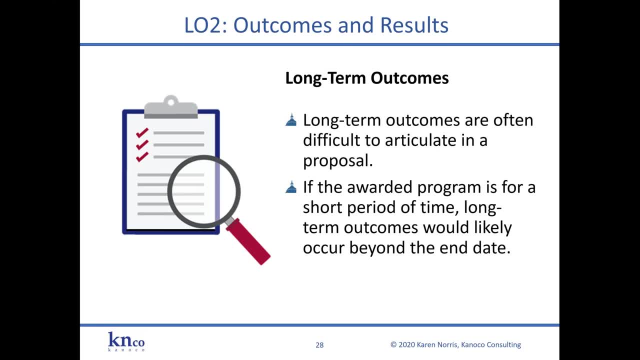 So they're difficult to articulate in a proposal, They're difficult to articulate in progress reporting, And if the awarded program is for a short period of time, the long-term outcomes would most likely occur beyond the end date. So how do you show the likelihood of continued success? 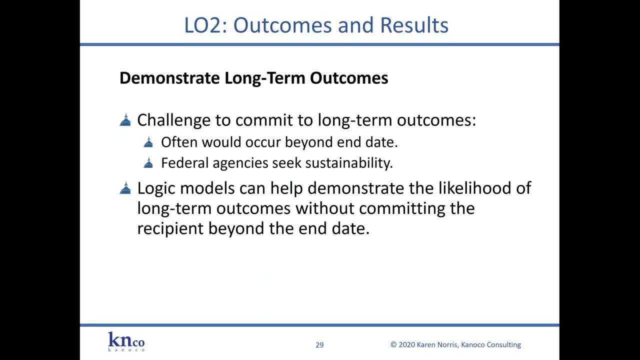 So the challenge is to commit to long-term outcomes. They often occur beyond the end date and at the means, and you can't. If you're on the recipient side of things, you can't commit your organization to anything once that grant period is over. 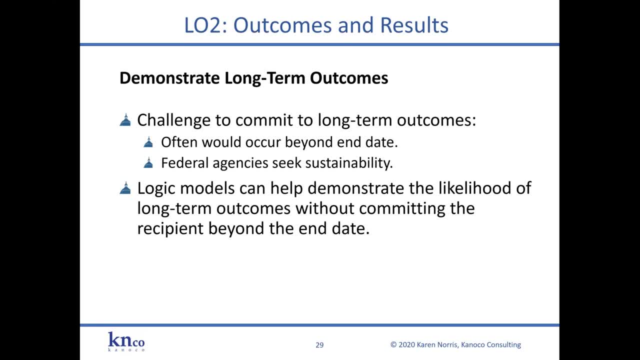 I mean it would be nice if things would continue, if things are sustainable, but you can't commit them, You know, not without institutional approval. So in the meantime, the awarding agencies, particularly federal agencies, they're looking at sustainability. 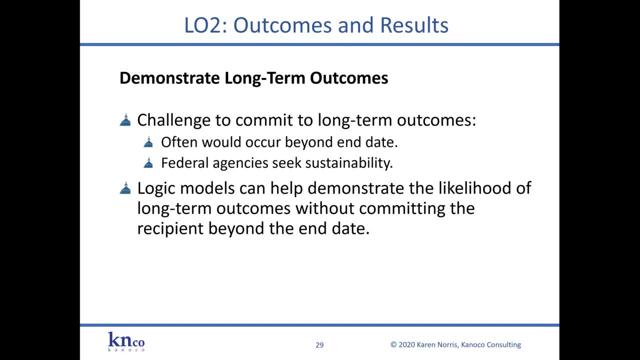 So what can be sustained? If not the entire program, what parts of it can be sustained, And how can you demonstrate a likelihood? And so a logic model really helps with that. So the word, the focus, the key word is the likelihood. 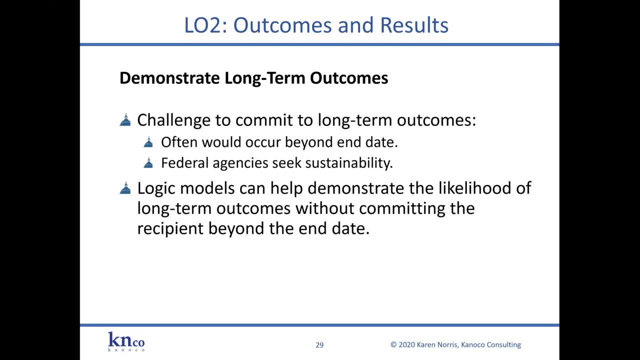 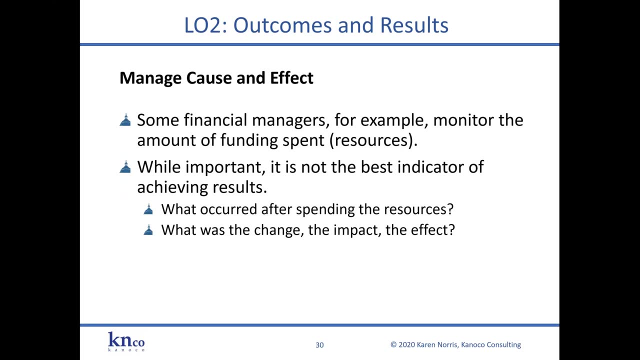 And it's the way you present your cause and effect, And if this, then this, and then the likelihood that it will continue. So some so managing cause and effect can be a bit of a challenge too. So you have financial managers and you have your program managers. 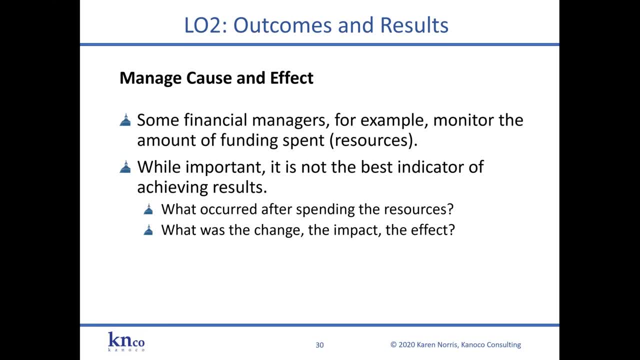 who are delivering mission And the financial managers do a really great job monitoring the expenditures, The amount of funding that was spent, which is the resource column of your logic model, And that's important. I mean, oftentimes they can tell when there's an issue. 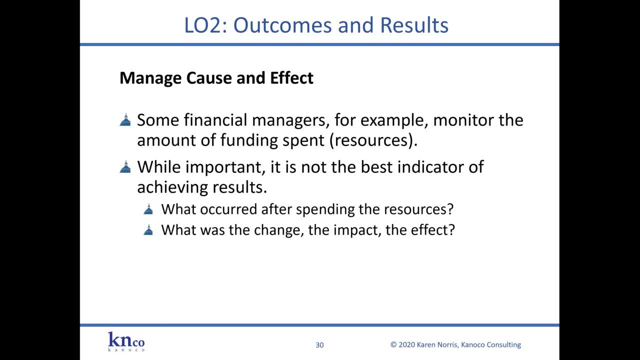 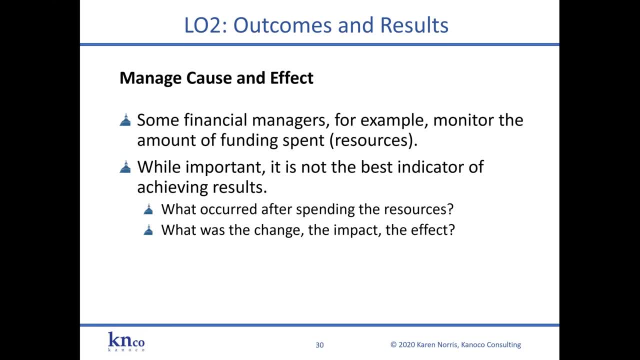 expenses. but while this is important, it is not the best indicator of achieving results, which is what you're struggling with when you submit these progress reports. So what occurred? What was the effect after spending the resources? What was the change, the impact? 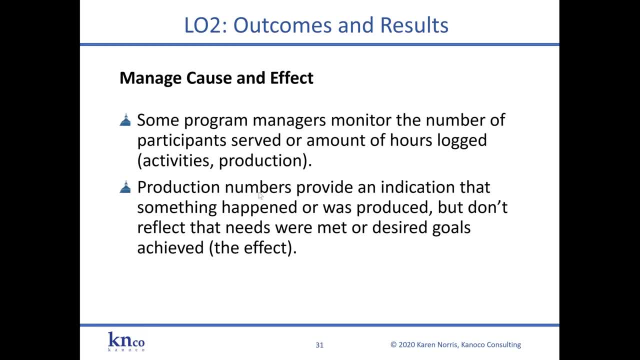 On the other hand, you have program managers and they're going to monitor their activity. They're going to monitor the number of participants who have been served or the amount of hours logged in. So again, you've got all these activities, these production numbers. 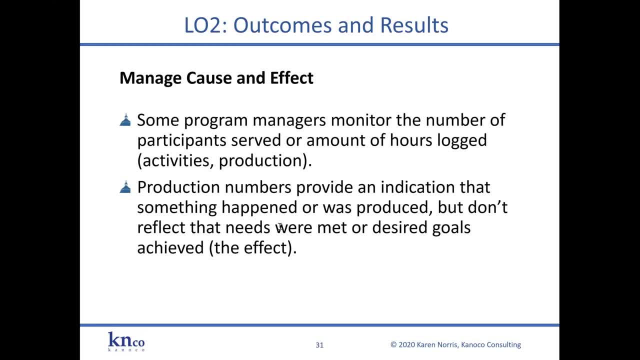 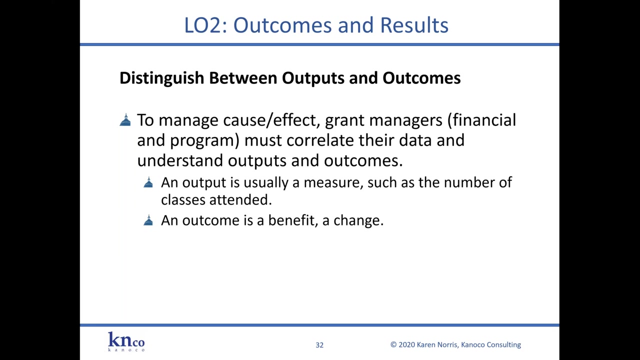 but production numbers provide an indication that something happened or was produced, but they do not reflect that needs were met or desired goals were achieved. the effect and the outcome, That's output. I'm trying to advance. There we go. Thanks, guys for your patience. So let's distinguish. 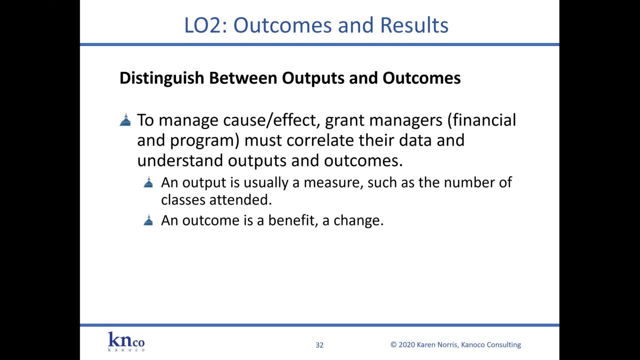 between outputs And outcomes a little bit, you know again, to kind of drive home the message: To manage, in effect, grant managers, whether you're financial or you're on the program side, you must correlate the financial data with the mission data and understand the difference. 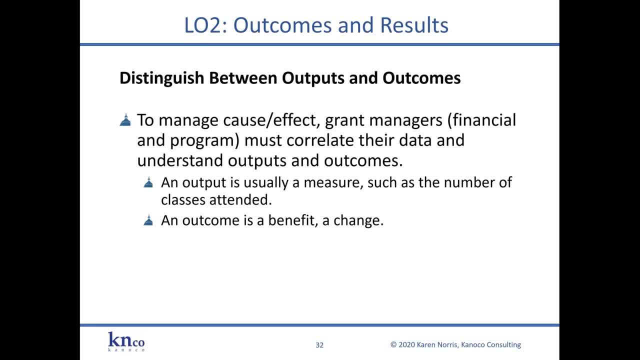 between an output and an outcome. And again, an output is usually a measure, such as the number of classes attended, The number of hours logged in- as a volunteer, you know. But an outcome, that's the gold standard And that's your benefit, or that's the change that took place as a, you know, as a result. 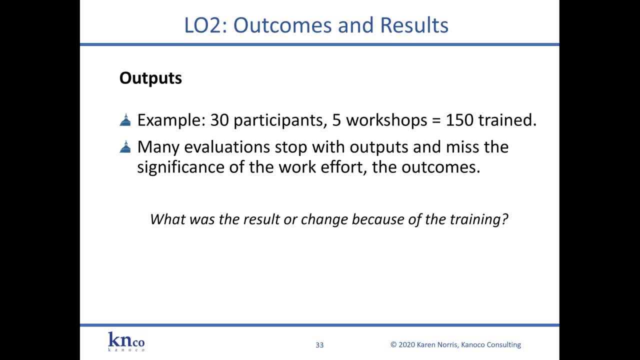 of all that productivity and that hard work. And here was the example that I cited earlier. You have 30 participants in a workshop and the grant was going to deliver five workshops And the grant was going to deliver five workshops, And the grant was going to deliver five workshops. 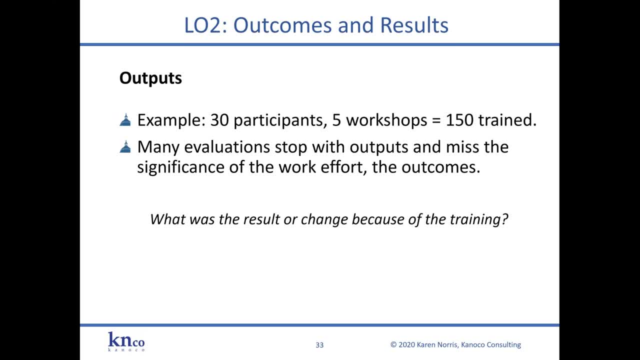 So you end up with 150 people who were trained. So here many evaluations stop with outputs and they miss the significance of the work effort, the outcome, What was the result or the change because of the training? How did these individuals who took the training, how did they change? 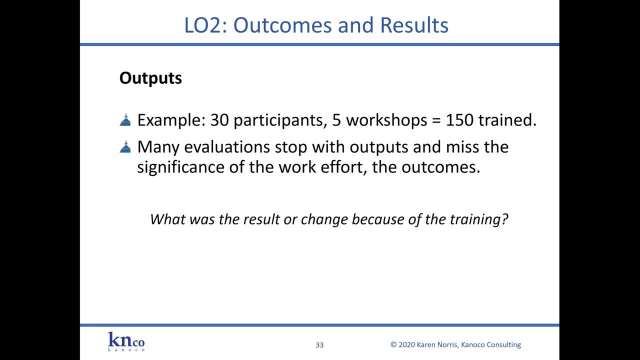 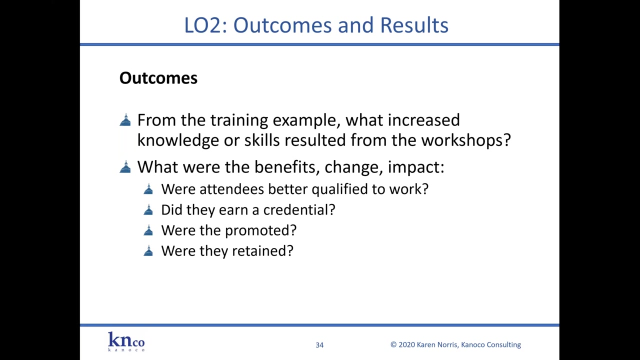 Did they earn a credential? Were they eligible for an award? Were they now skilled in a particular machine language, Were they able to present a new curriculum? And what's the positive impact of all that? And on this slide, this is exactly what we just talked about. 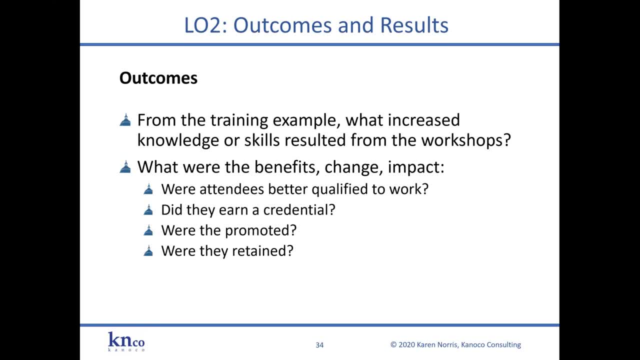 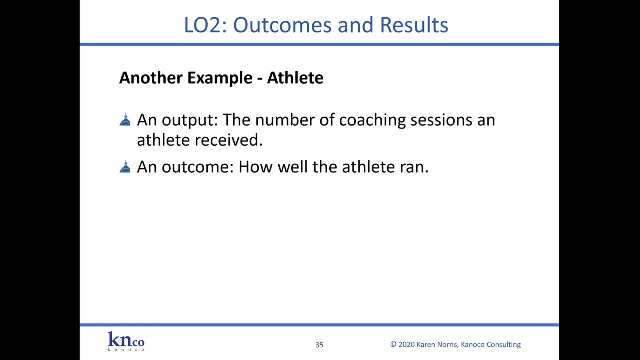 What were the benefits? What was the change? What was the impact? So here's another example. You have an athlete and an output is the athlete had took X number of coaching sessions, But what would the outcome be? The outcome is well. did those coaching sessions make a difference? 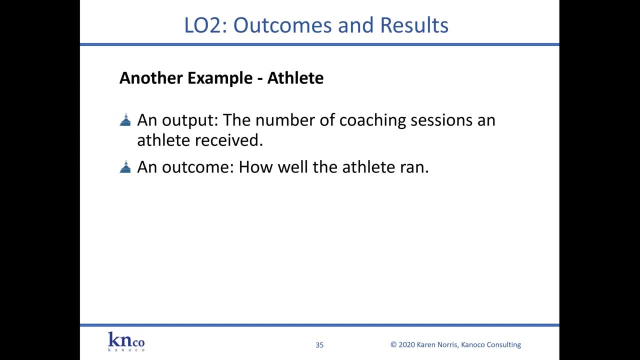 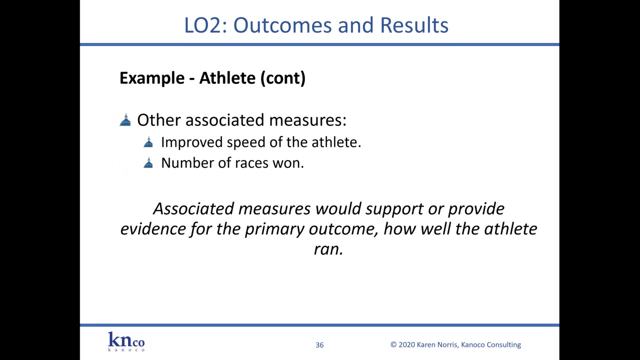 How well did the athlete run? Is the athlete now faster? Does the athlete have A better start, You know? does the athlete have more long distance, more stamina? What was the outcome of the number of training sessions? And continuing with this analogy with the example of an athlete, what are there? some other associated measures? 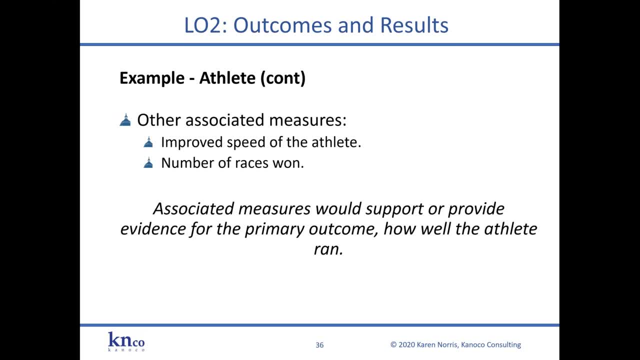 Was the athlete faster? Did the athlete win more races? That kind of demonstrates that the athlete is running not only better than he ran before, but the Because the athlete is running better than everybody else. So associated measures would support or provide additional evidence for the primary outcome. 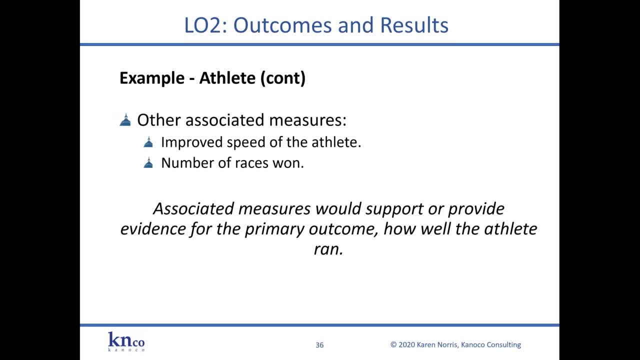 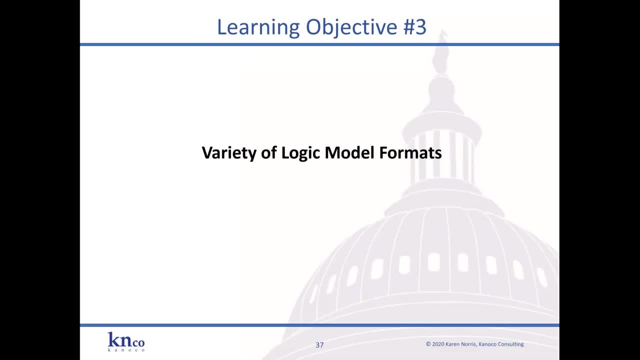 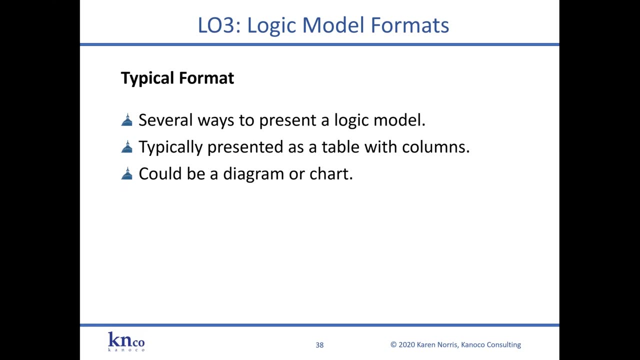 How well the athlete ran. Oh yeah, he's running. well, Look at all these medals. OK, so let's look at different logic model formats. So there are several ways to present a logic model, and it's there, It's typically present. 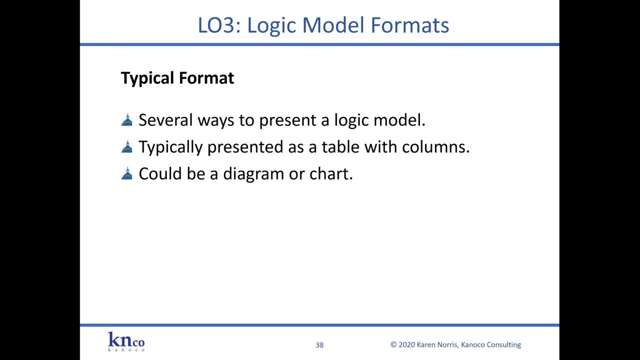 It's a visual, It's not just narrative words, It's. it's an actual design, It's a visual display and it could be a table or with columns, And I like the column view best, but the column view doesn't always work well with some research grants. 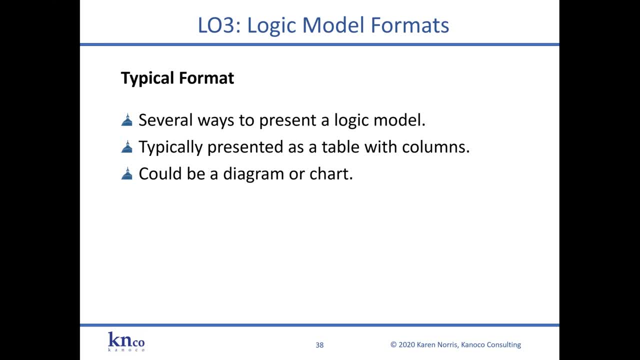 So it could be a diagram or a chart, Or a chart in those cases where the columns aren't as as practical. So again, the lot, the column format or even the chart format. the intent of whatever format you select is going to capture information as a progression from cause to effect. 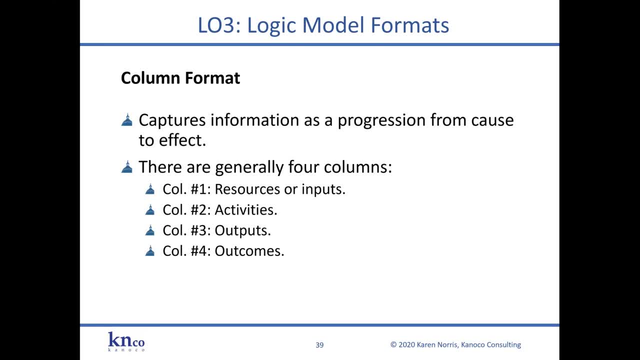 And if you're using the column format, they're generally four columns. So column number one is going to be your resources or your inputs, Column number two will be your activities, Column number three will be your outputs and column four will be your outcomes. 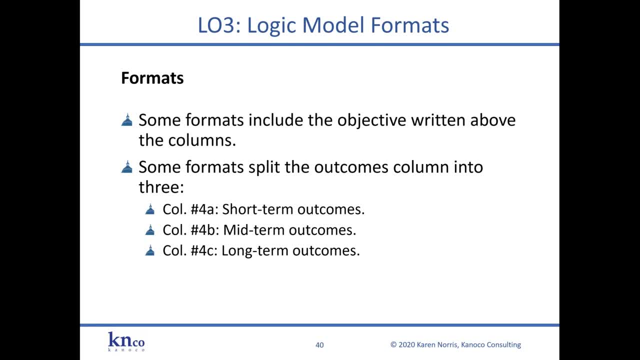 Now, and some formats include the objective written above the columns. That's the one that I happen to like the best, particularly if you have a Fairly complicated grant program with several objectives and several things happening. I find if you try to use one logic model- excuse me- to articulate progress for multiple objectives, that logic model becomes very long and a little bit unwieldy- unwielding. 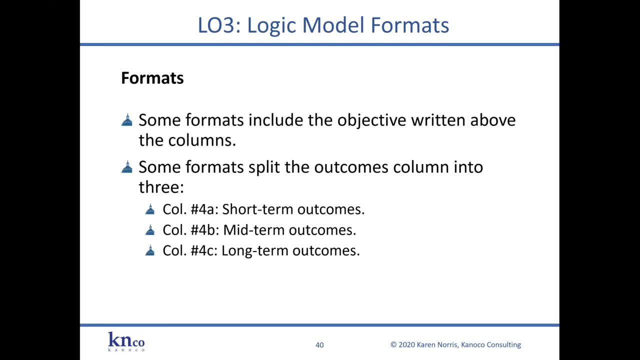 So if you divide up your logic models, So you have one logic model For each objective, then you could clearly show that the activities are for that particular objective, The money that you spent is for that particular objective, And then these are the outcomes from that, from that objective. 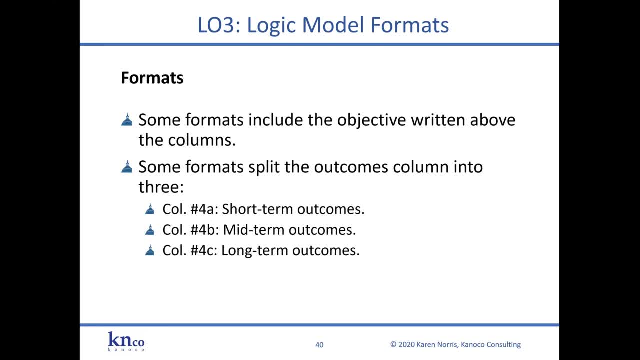 And it's just makes it very clear to demonstrate performance and results for each objective in the program. So some people Still prefer to have one logic model for the entire grant program. I'm of the school where I would prefer separate logic models, one for each objective. 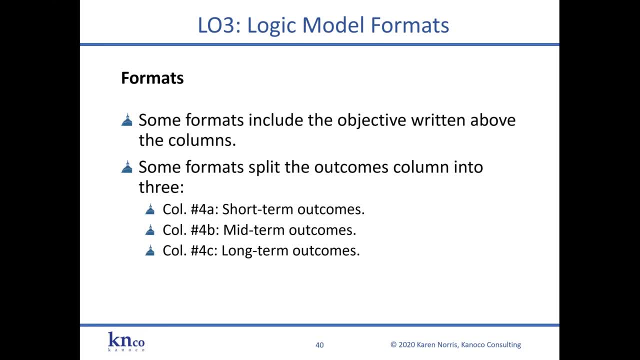 So another consideration in thinking about the format that you select is that some formats will split the outcomes column into three parts. So instead of having four columns- Reference resources or inputs, activities, outputs and outcomes- they take that outcome column, that last column, and expand it to short term outcomes, mid term outcomes and long term outcomes. 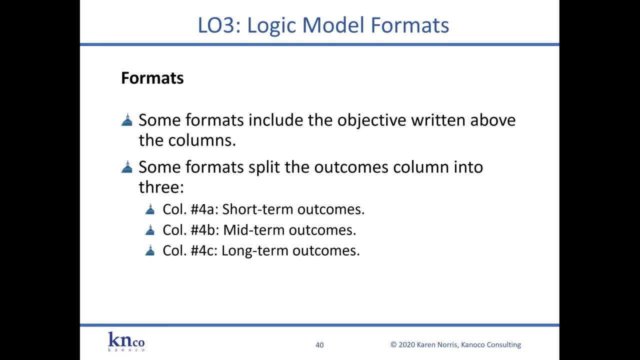 And again, if you reflect, you know I've used both ways, I've used what. it depends on how complicated the objective is, the grant is. the one column for outcomes could be sufficient. I tend to think the simpler the format, the simpler the presentation, the clearer it is to 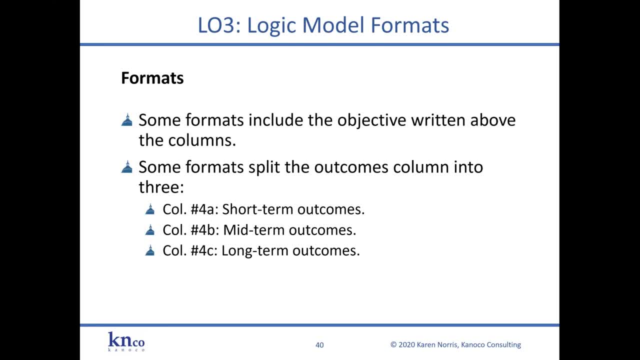 understand, but sometimes it's very appropriate to have short, mid and long term outcomes, particularly if it's a multi-year grant project and it also indicates you know it lets the federal agency know that you're thinking in in terms of long-term outcomes, you're thinking in terms of sustainability now, 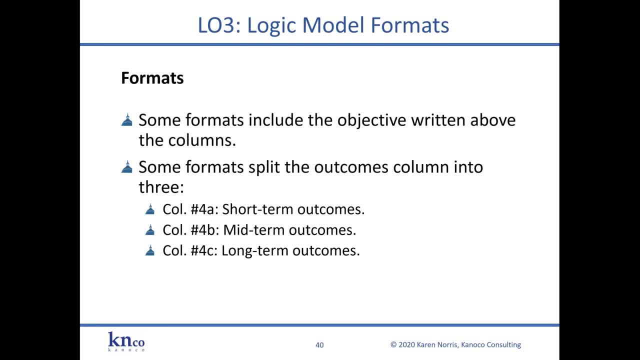 you can still articulate that with one column for outcomes, but it without a doubt it's very clear if the outcome column is split up. so some awarding agencies have their own version of a basic logic model and they're becoming popular. the EPA uses logic models, for example, and sometimes the federal awarding agency. 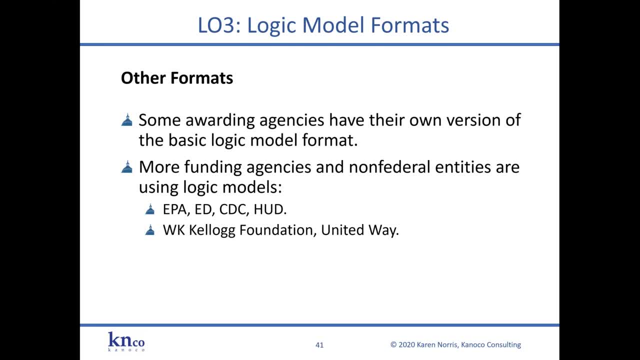 provides you with the format that they want you to use other times. they don't they're, they're silent. they don't say you can use a logic model. they don't say you can't use a logic model. they just want you to be able to articulate. 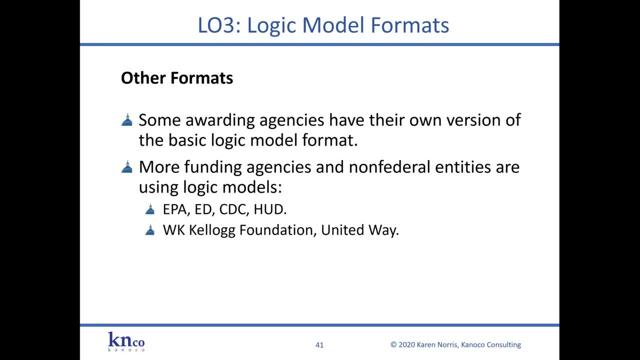 performance and results. and if that is best handled by using logic model, then great, you know, no problem there. There's no prohibition, in other words, of using a logic model, even if it's not mentioned in the grant solicitation guidelines or your award. 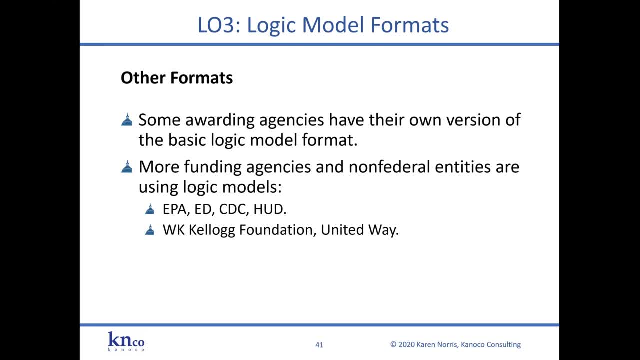 agreement. I think what's interesting is the uniform guidance is currently under revision And in January of this year the Office of Management and Budget, OMB, published a federal register notice and they released the proposed changes to the uniform guidance. At the same time, the president's management agenda on performancegov under Cap Goal 8 for 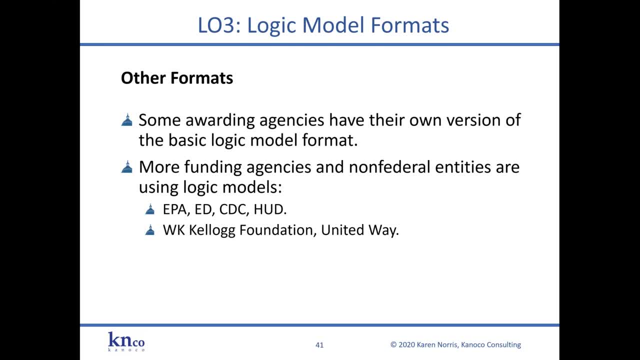 grants has published what they call a redline version Of the proposed changes. So they have produced, they have put a copy of the current version of the uniform guidance online with track changes on. I think that was very clever. I found that tool. 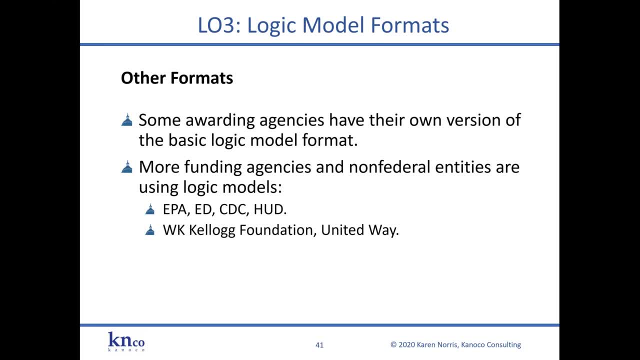 to be very, very helpful. And then with the track changes, with the redline version, you can see where the revisions are for each provision number And you can get a copy of that online. And then with the track changes, you can get a copy of that online. 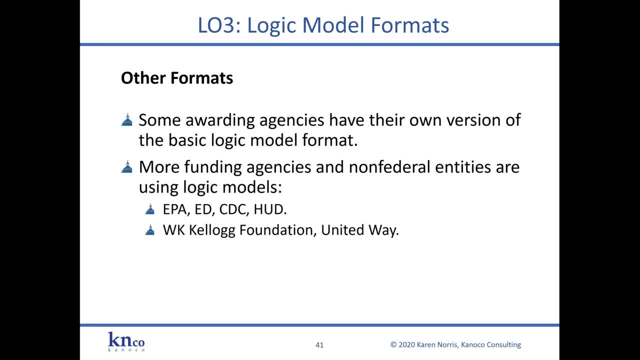 So one of the changes, one of the proposed revisions in the uniform guidance is the uniform guidance is now actually mentioning logic models and that they are appropriate for grantees to use when reporting performance and results in their evaluations. So what's the schedule for that? Well, in January of this year, the Office of Management and Budget OMB published a federal register notice. In January of this year, the Office of Management and Budget OMB published a federal register notice. In January of this year, the Office of Management and Budget OMB published a federal register notice. 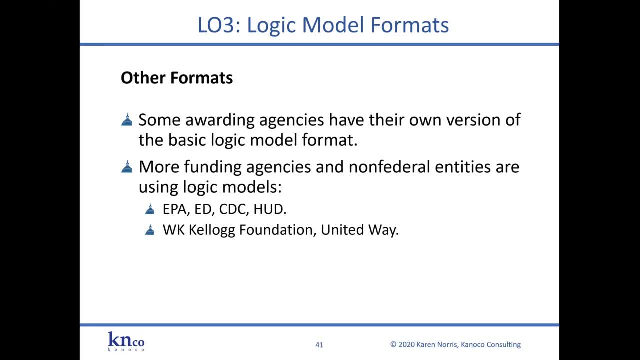 The proposed revisions were released And then there was a public comment period that closed March 23rd And OMB received 200 and some comments. Now they are in the process of reviewing all the public comments on the proposed revisions And they're going to make determinations. Well, no, that revision doesn't help. That's not helpful. That comment is not helpful. 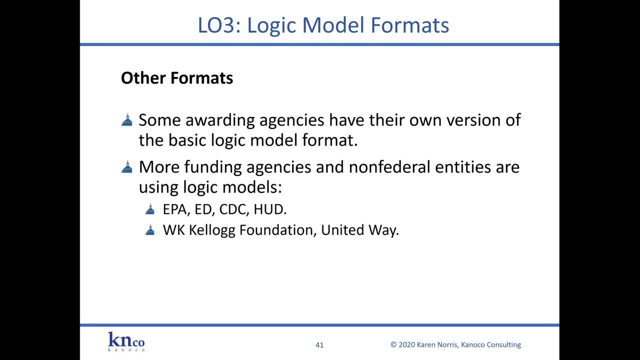 we'll ignore that one, and we'll ignore that one. oh, but this comment has a good, good idea. let's let's further refine the revisions. so they are in the process now of reviewing all the public comments that they received to determine whether they're going to revise the guidance further, and sometime this year, we expect. 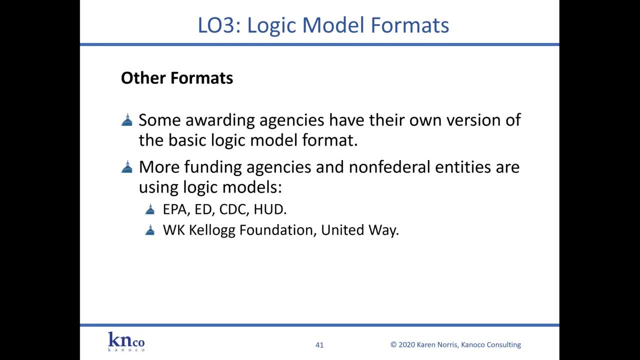 them to publish a final rule in the Federal Register where the revisions will go live with the uniform guidance. now I have heard rumors that that's going to happen in August, but I will be happy if it happens by by the end of December. you know when they when they release the uniform guidance initially. 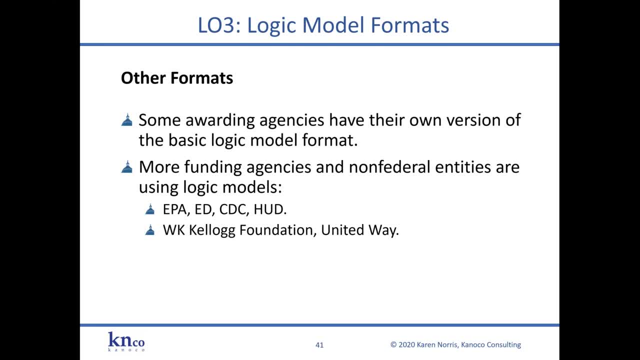 you know, we were waiting and waiting and waiting for it and one day was saying, oh, we'll have it out before the end of December, but it's going to happen. I'll go through moreardare fits now. if I recommendplate dishes today, I can do it once. maybe I'll try to did. we were waiting and waiting and waiting for it and be saying, oh well, have it out before the end. 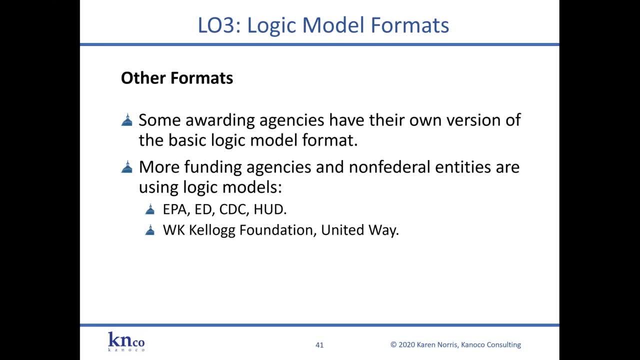 of the year. We'll have it out before the end of the year And you know September, October, November. at what point is it going to come out before the end of the year? So they actually released it on December 26.. Now that's the day after Christmas, like nobody's around. This was 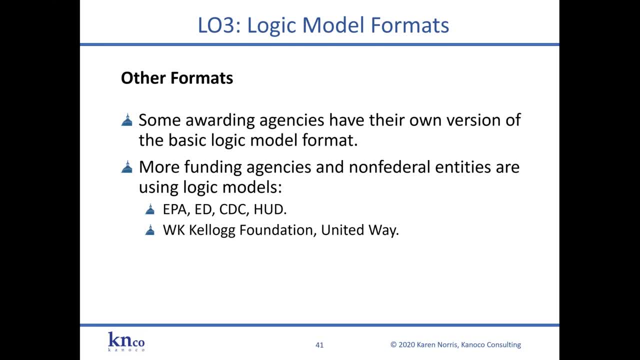 the biggest thing to come down the pike in the grant world for the in 30 years, And it was finally released December 26.. So if we get the final rule in August, that will be great, But I'm betting on December 26 of 2020.. So we'll see. So some other? so, in addition to having some federal awarding, 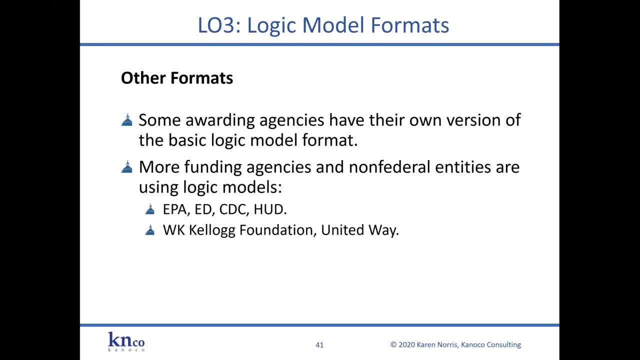 agencies that may have their own version of the basic logic model format. there are more and more funding agencies and non-federal entities that are using logic models And the EPA refers to them, the Education Department refers to them, the CDC and HUD has. 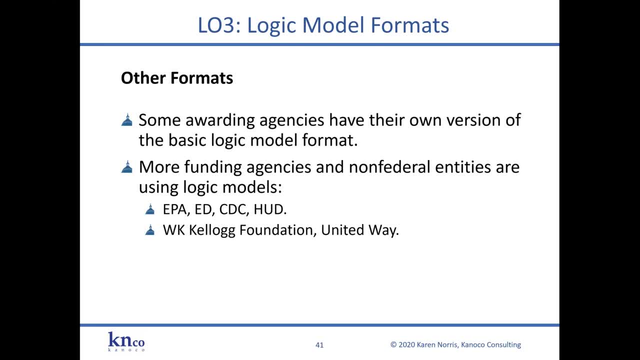 referred to them, And in the private sector. the Kellogg Foundation and the United Way support and are proponents of logic models And they have some interesting explanations and resources on their website. So it is becoming more and more popular of a tool, And if you were just 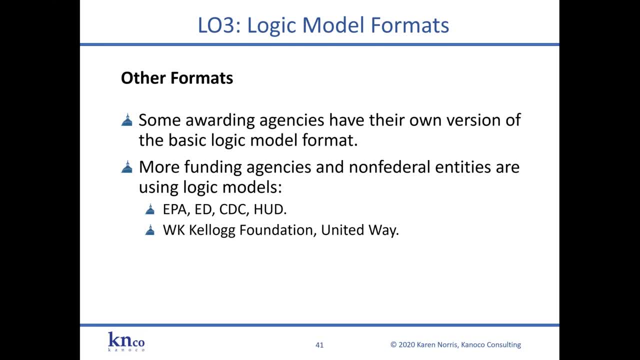 to go after it. you would be able to find it on the website. So if you were just to go after it, this webinar is over. if you were just to go and Google the term logic model, you would find a whole bunch of information about it. But hopefully you know I've provided for you here a good 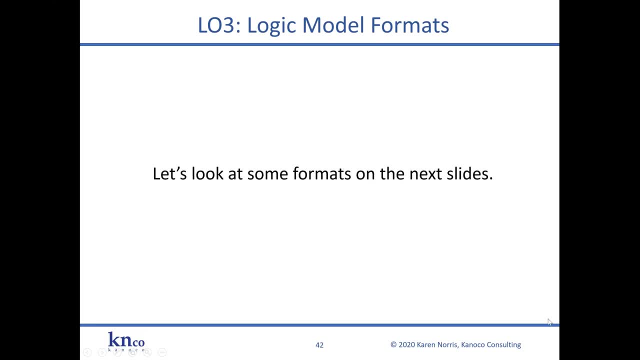 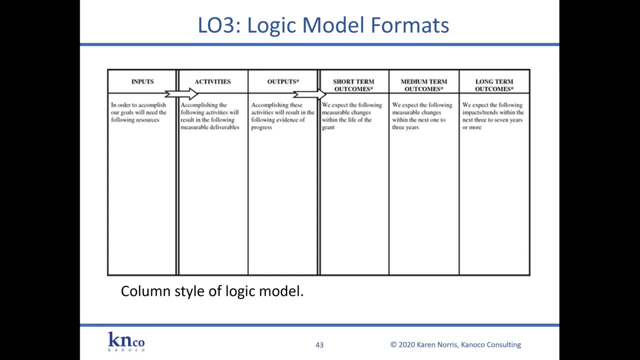 sampling of what you would find if you go research it on your own. So let's look at some of these different formats on the next few slides. So here is a format and you've got your basic columns, your inputs, and then your activities and your outputs, And here this one has taken the outcomes. 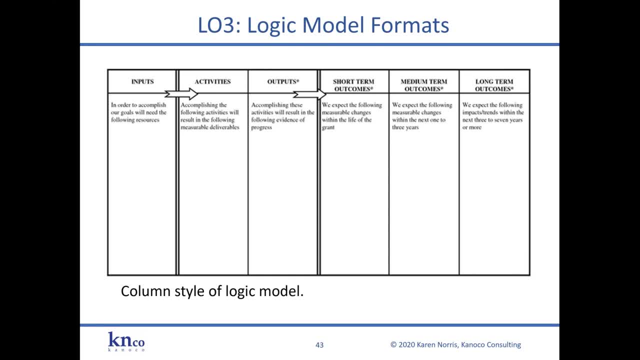 column and they split it up into short, medium and long-term outcomes And they further defined it. a short-term outcome is going to take place within the life of the grant, usually 12 months. A medium-term outcome is: we expect the following measurable changes within the next one to three. 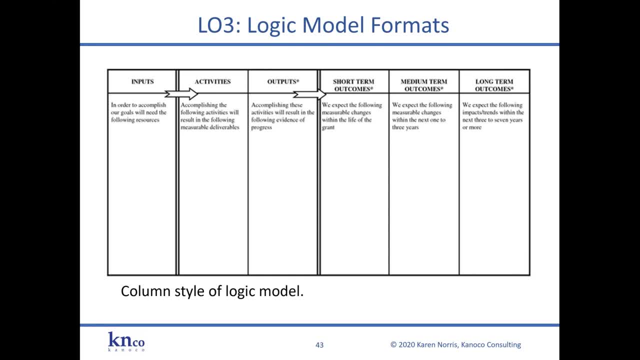 years And long-term. we expect the following: measurable changes within the next one to three years, And long-term is defined as within the next three to seven years or more. That's how they defined it. So you can write the logic model. Let's say you have a five-year grant, So you would 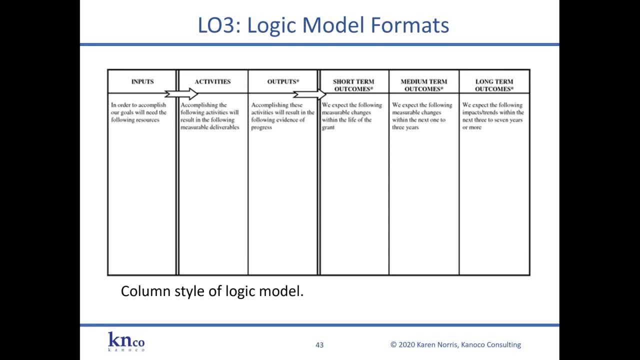 have short-term outcomes for maybe year one, two and three, And then medium-term would be year three. Oh, someone is asking Amy, is that anything that you need to address? No, sorry, That was the notification. No worries, Keep going. 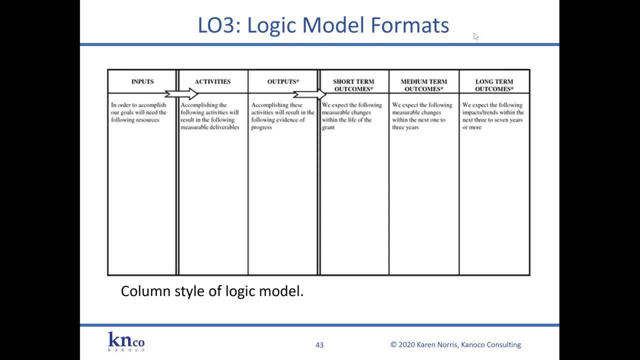 Okay, All right, I'm on the East Coast, So it's like, uh-oh, my poor people in California, Yeah, You know. so, all right, So great. So here I think, what's interesting. so, oh, my goodness. 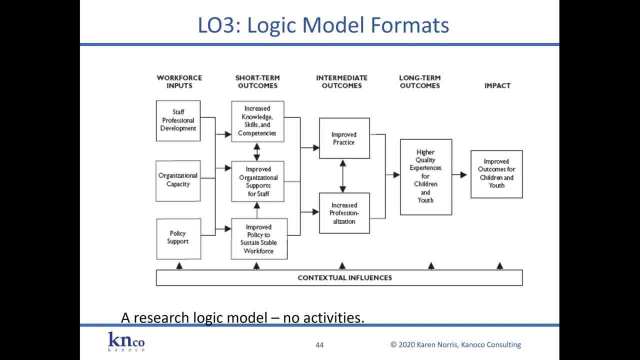 So well, let's hope it was something simple. Okay, So, Amy, you can go ahead and join us. Okay So, Amy, if you feel that you have to leave the webinar, Amy do so. You know, if you feel that you have to leave us, go ahead, And Amy will post this webinar up on the website, And I think she has a YouTube channel that she can explain about you know later. So you have access to the webinar. Yeah, Apologies everyone for these notifications If you're getting an earthquake as well. I haven't felt anything here, But it sounds like some places in California are getting hit by the earthquake. Yeah, Okay, Oh, my goodness. 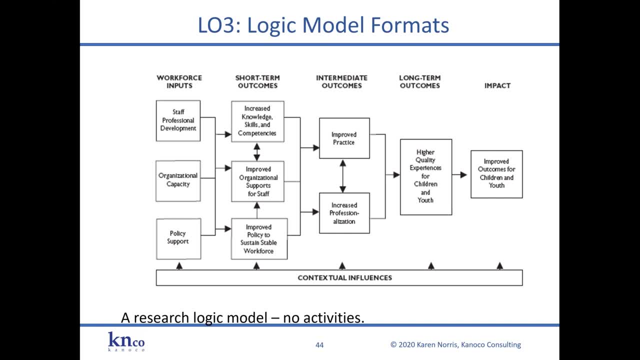 But yeah, if people do need to log off, we will have this presentation up on the OPR website, the Federal Grant Resources page, and also on the OPR YouTube page, which you'll be getting a link to tomorrow in the follow-up email. 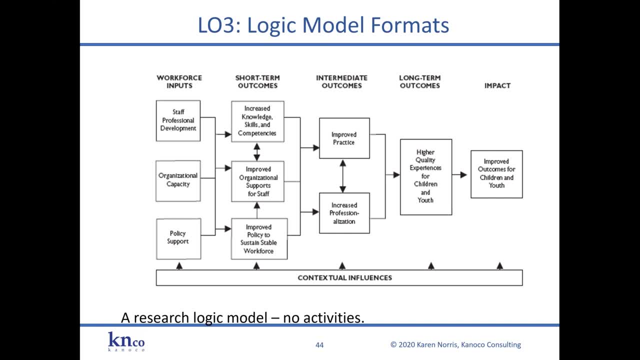 So it might take a couple days for us to get everything. Okay, Great. Thank you so much, Amy. So good teamwork. This is a format that is often very useful for research projects. There are no activities. That's the biggest difference between this model. 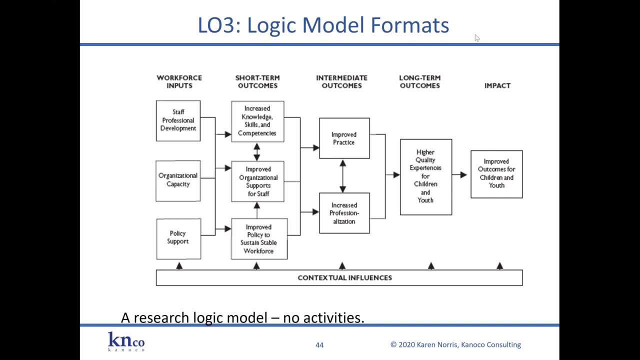 Not just the fact that this one is little boxes with arrows and not columns, but the biggest difference, difference between this version and the prior ones that we've been talking about- is that this one has no activities, so you have what's called workforce input, so there's going to be staff. 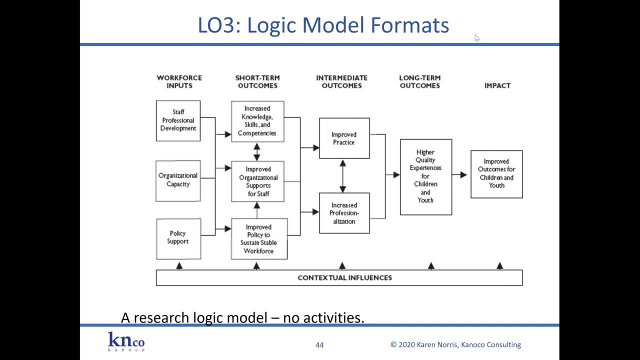 professional development. You're going to try to increase organizational capacity. You're going to support a policy, possibly that to constantly, you know, seek out new knowledge. It could be policy support. I think that is a really good, no matter what logic model you're working with, the fact. 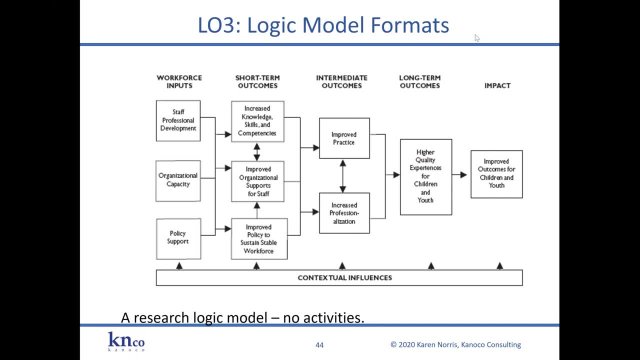 if you can say that your grant project is supporting a mission, your mission and here's the policy, if you you know every federal agency has Government Performance Results Act goals and the GUPRA goals and it or a strategic plan, and if you can say, oh yes, it's also supporting the federal agency's. 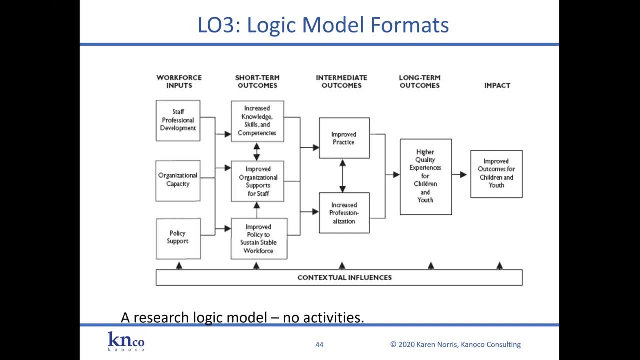 strategic plan- any type of language like that, I think, is always valuable to put in a progress report- And then, of course, you have your short-term outcomes, your intermediate outcomes and your long-term outcomes, and then they have the ultimate impact. that's that's being shown. 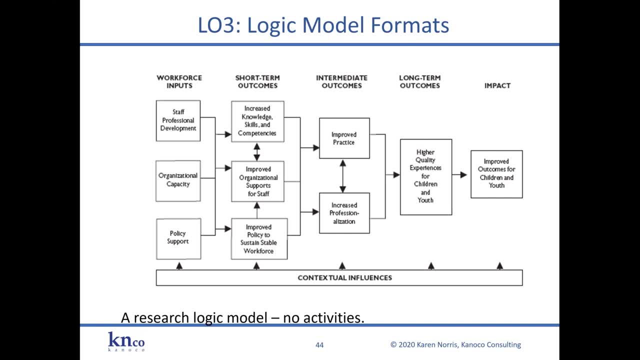 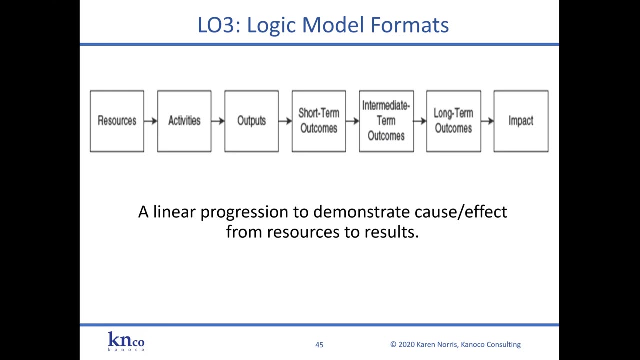 shown in this, in this version. I think it's interesting. they kind of reflect these different formats, kind of reflect how people's minds work and how they're thinking and the progression of the cause and effect relationship and what is the right progression for your particular agency and for your particular project. So here's. 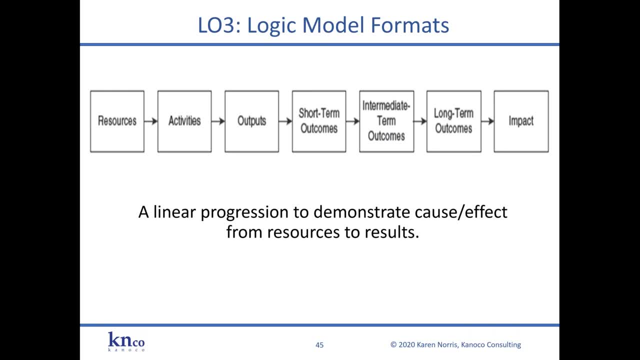 one that just boxes without the question. you get the beginning. That's what we're talking about here: the columns, it's resources, activities, outputs, and now you have short-term outcomes, intermediate, long-term and then the ultimate impact. 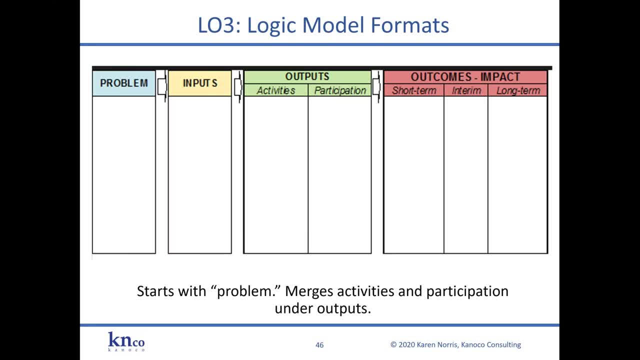 Here's a colorful model. This one's interesting because it starts with the problem and that's similar to the one that I use, but I like having an objective. but what's the objective? Because you've promised these objectives in the proposal. but I think this is very interesting and to say, well, this is the. 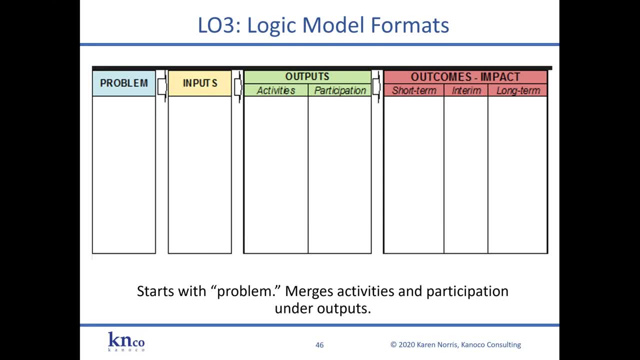 problem. This is why we submitted the grant to begin with, and to restate the problem there in the logic model. and then you have your inputs- They have activities and participation underneath outputs, and then you have your outcomes or your impact, and that column is split between short-term, interim and long-term. 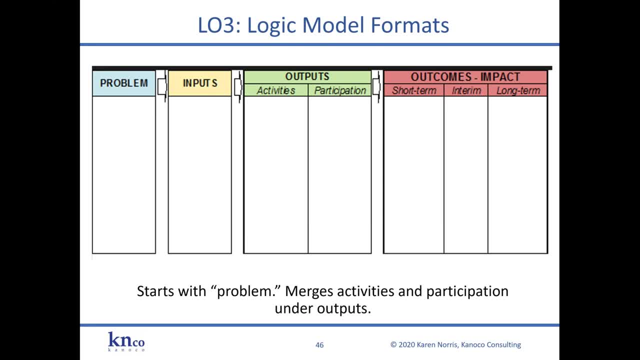 So you can see that there are key words that are, you know, key concepts that are being used in each of these logic model formats. but there are this variety of formats. You're able to pick the format that would work best for your project. This is: 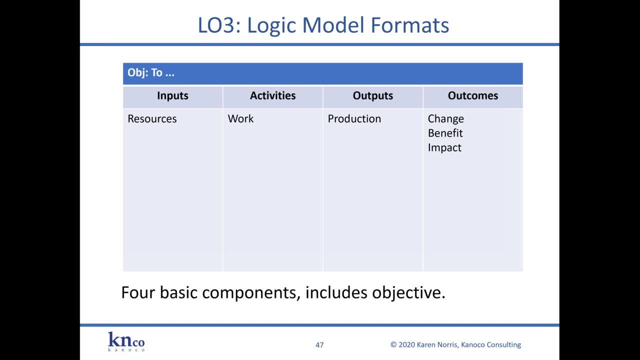 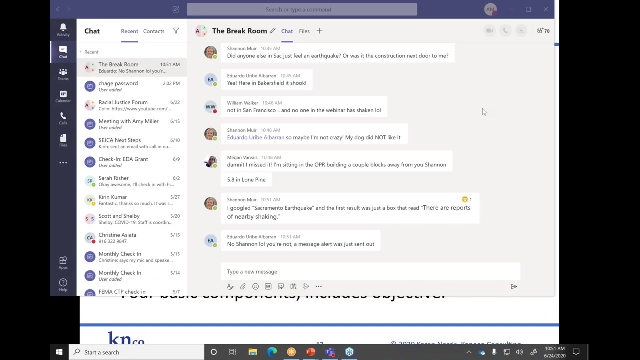 the one that I like to use, where you have your objective across the top and then you have your basic four columns: your inputs, your activities, your outputs and your outcomes, And that's where you can see where we need to go from here. 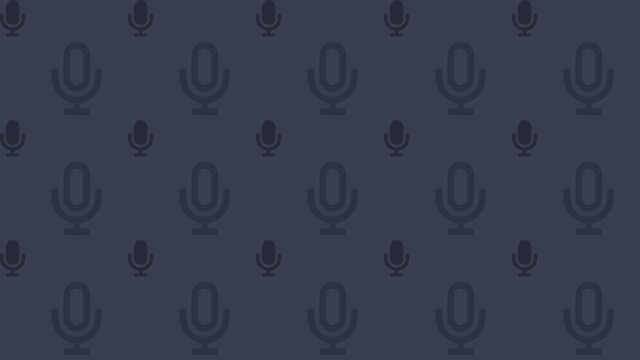 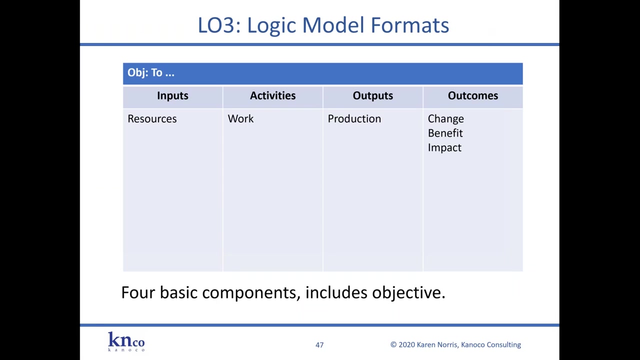 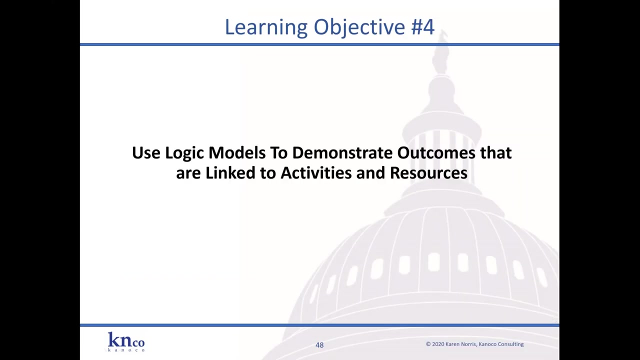 It's interesting, I don't know how many people who want to say: well, there's this very, very complicated approach And if you look at what I do and I can just kind of make the description more simple and easy to get on and I'll give you a little bit of presentation. 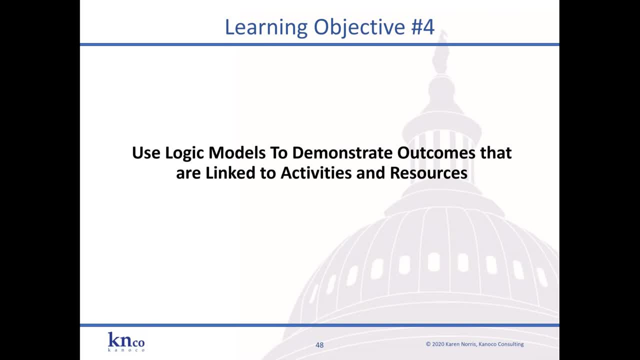 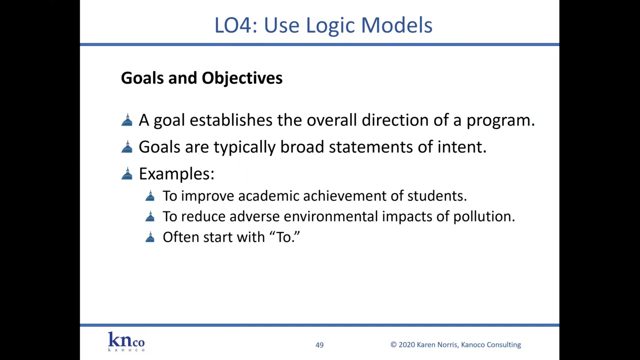 here work A logic model, having a really nice format for your logic model is great, but if you do not know how to write measurable objectives, the logic model is not going to be as effective as you would hope it would be. We're going to start off by talking about goals and objectives. A goal would 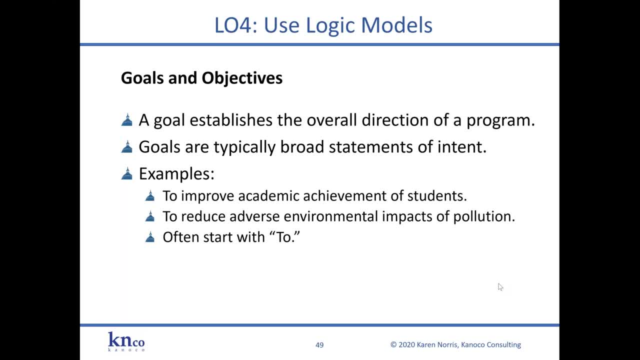 be something broad, lofty goals, lofty language, broad language. that's going to establish the overall direction of a program, For example, for health and human services, federal HHS, the federal department of HHS. they would have a goal to decrease health disparities nationally. So there's a very lofty 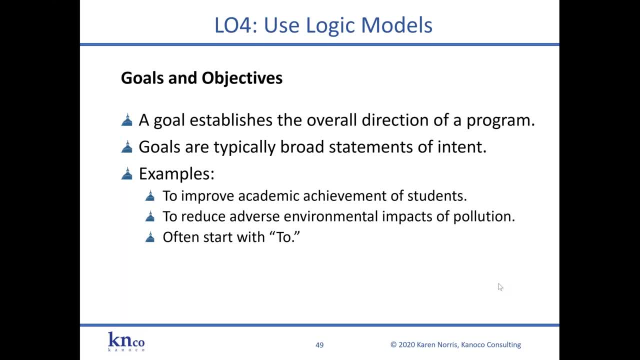 goal: Broad language. that's the overall direction of that particular program. A goal is typically said broad statements of intent. So examples would be to improve academic achievement of students. Of course that's what all educational agencies want to do To reduce adverse environmental. 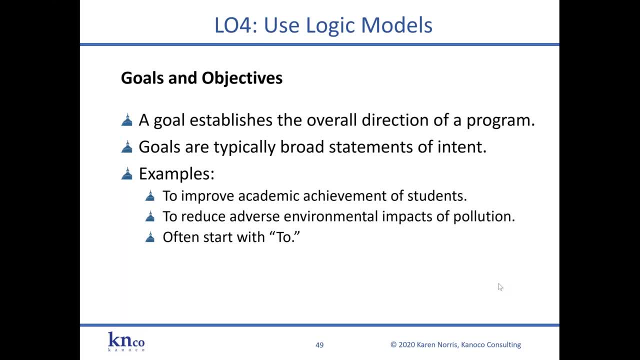 impacts of pollution. To reduce environmental impacts of pollution. To reduce environmental pollution Again, to reduce health disparities in the United States. To reduce the number of deaths on the highway by mandating the use of seat belts, you know, for the front seats. So very lofty goals. 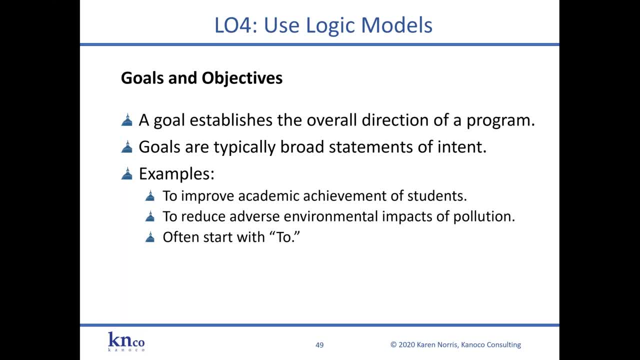 the intent. We're going to save lives, reduce deaths, reduce disparities, improve achievement, reduce adverse impacts. Very lofty statements, broad statements of intent, And they're usually two statements. They usually start with the word two: Now an objective is going to be more detailed. It's going to define the steps to achieve the goal, And objectives need to be more specific and they need to be measurable. You need to be able to measure your progress. 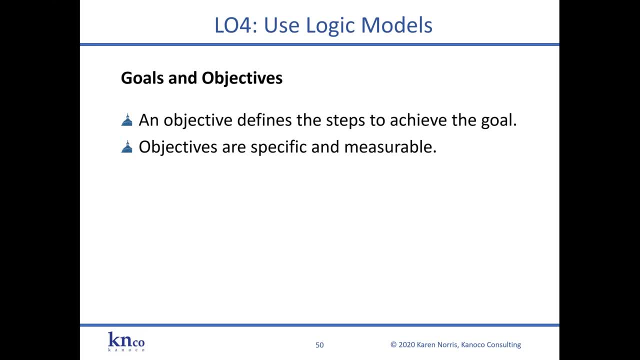 And objectives need to be more specific and they need to be measurable. You need to be able to measure your progress, And objectives need to be more specific and they need to be measurable. You need to be able to measure your progress And to demonstrate your performance, And so there's a way to write objectives that is better than other ways. There are a few ways to write objectives that are better than other ways of writing objectives, So I'm going to give you some examples. So let's talk about a well-written objectives. Here's in a poll, another poll. So, Amy, can you put up the next poll? 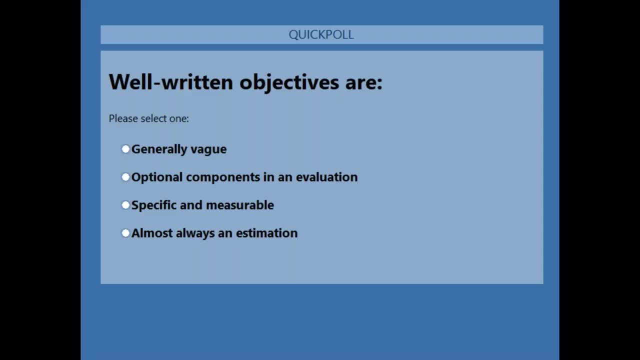 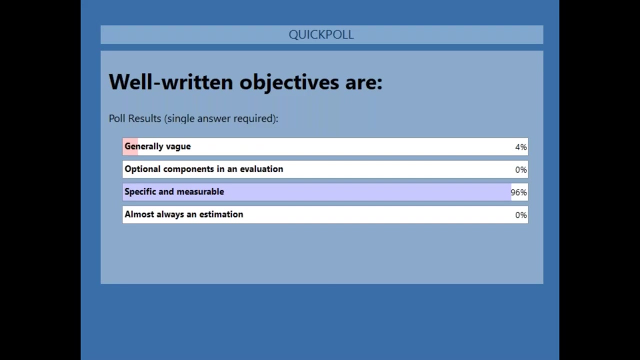 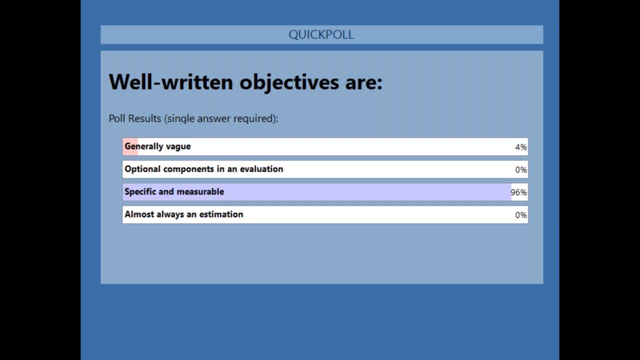 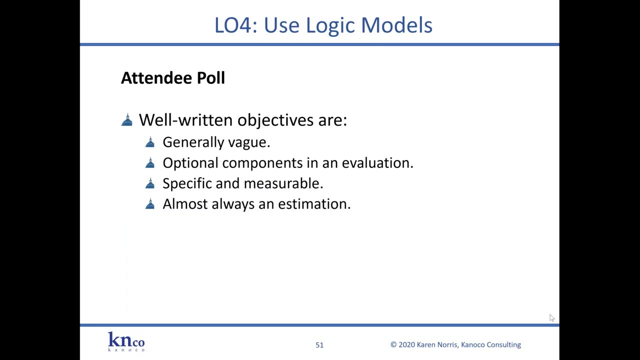 objectives are going to be specific and measurable. So good job everybody. So there are several kinds of objectives. There's something called a SMART objective and a lot of federal agencies refer to these SMART objectives- That's an acronym- them. They're process objectives and they're outcome objectives. So just looking at these, 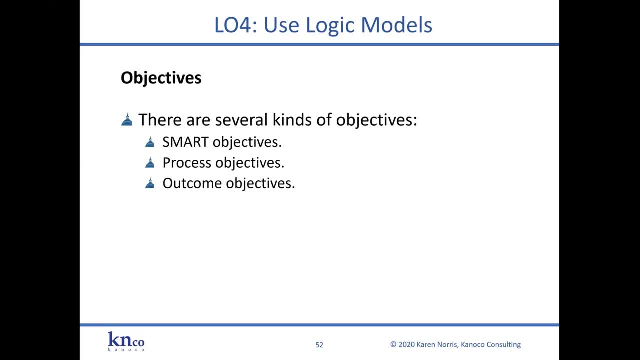 words. you know this is the SMART objective. You want to make sure, whatever objective format you use, you want to produce an outcome And the logic model is going to reflect that you've got your outcome. So think in terms of outcomes. So here's a SMART objective and it follows a little formula. 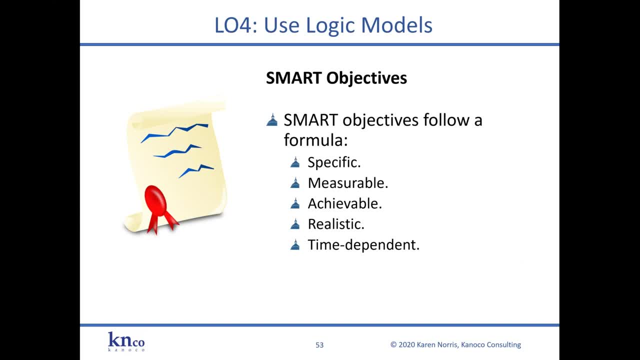 and there it is: S-M-A-R-T. So specific. the goal has to be more specific, written more specifically than a goal. The objective needs to be more specific. It has to be measurable, like a before and an after. It can't be so aggressive that there's no way you're going. 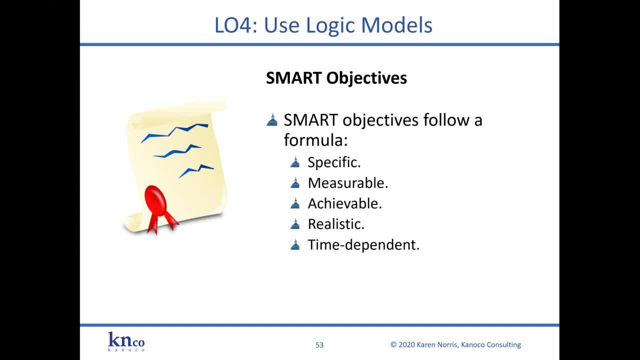 to be able to achieve it. So it has to be thought out so that it's achievable. it's realistic. To me, achievable and realistic are pretty much the same. And then time dependent, which goes in hand with the uniform guidance requirements for a timeline for completion. 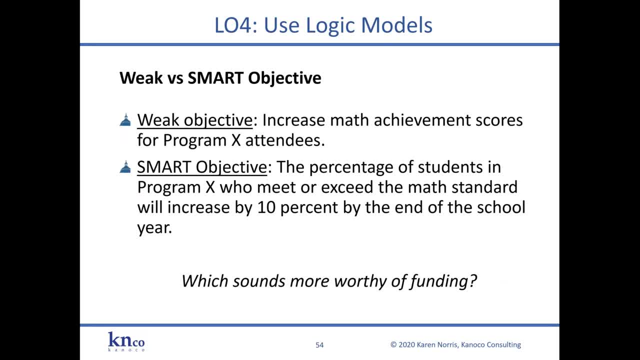 So here's a weak objective versus a SMART objective. So the weak objective is we're going to increase the math achievement scores for program X attendees. Okay, so that shows the basic intent of what you would intend to do, but how are you going to measure how? 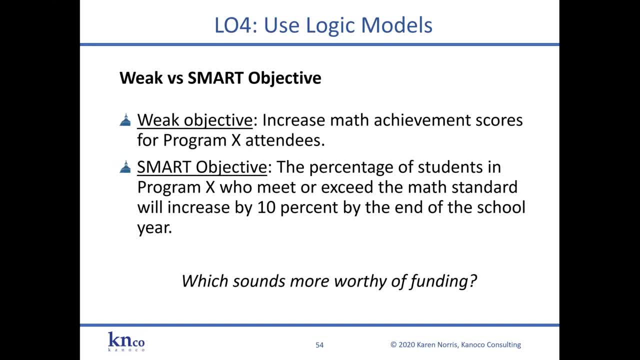 are you going to know that you've improved the achievement scores? So the smart objective would say: well, the percentage of students in program X who meet or exceed the math standard will increase by 10 percent by the end of the school year. So it's a little wordy, but you have your students in the same program. they're going. 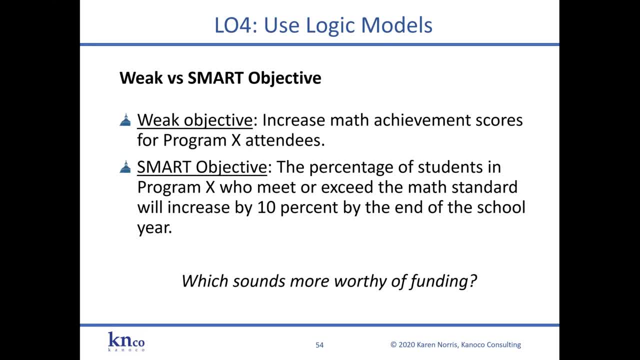 to exceed. It's referring to a local standard- that they have to at least meet the standard or exceed it, and they're going to at least make sure. it's going to increase by 10%. and there's your timeline, by the end of the school year. So between those two objectives, which one sounds more worthy? 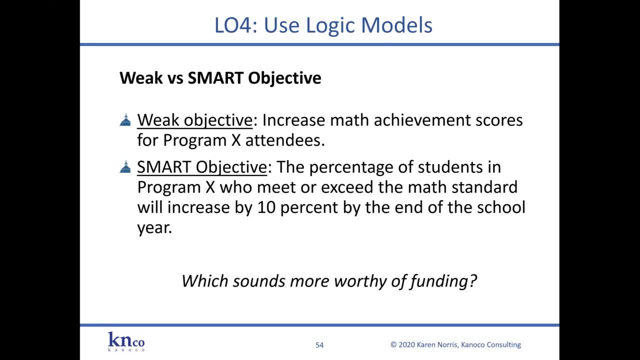 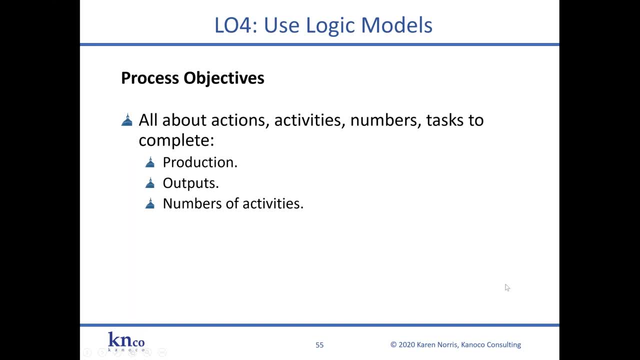 of funding. Obviously, the SMART objective. You know these people are focused, They know exactly what they're doing. Let's talk about process objectives. So a process objective is all about actions and activities, numbers, tasks to complete. So a process objective is better at demonstrating. 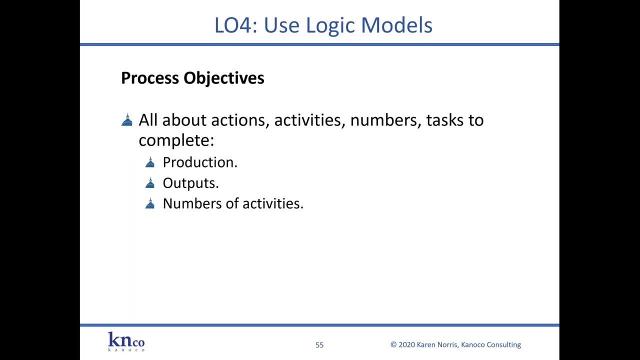 production and outputs, and numbers rather than outcomes. So let's look at some examples of process and outcome objectives and of course, we're going to compare and match them. So let's look at some examples of process and outcome objectives and of course, we're going to compare and match them. 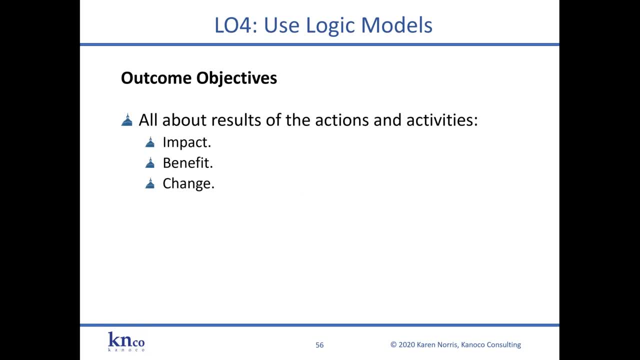 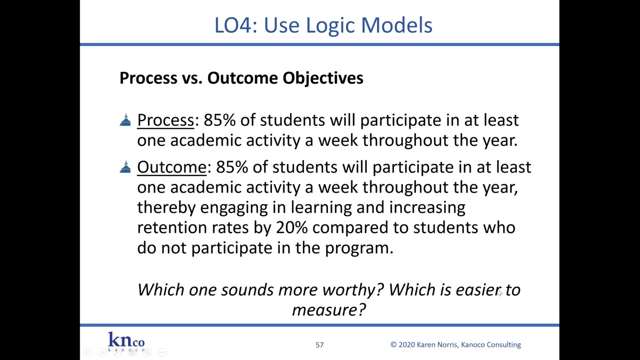 the process objective to the outcome objective. the outcome objective is all about the results of the actions and activities. what's the impact, what's the benefit, what's the change? please forgive the delay. here we go. so here are some examples of a process objective versus an outcome objective. the process objective would say 85% of 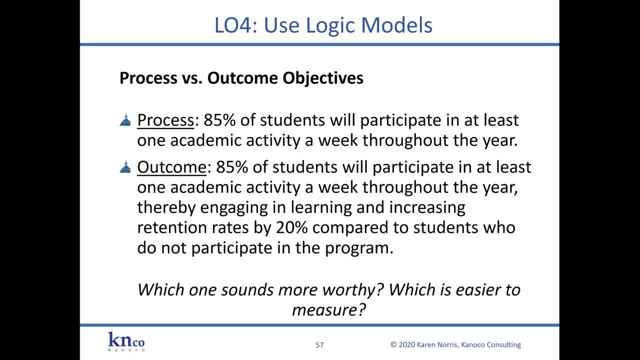 students and right away start. hmm, that's a, that's a specific number. that sounds pretty specific to me. you know, 85% of students will participate in at least one act at one academic activity week. well, that that's something you can measure, right. they're participating in one activity a week throughout the year. 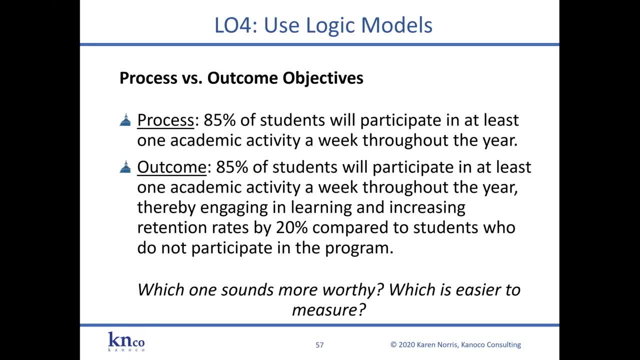 and there's your timeline. what's so bad about you that that one's pretty good. but it's going to measure the the out, the outputs. now let's look at the outcome objective. it starts the same: 85% of students will participate in at least one academic activity a week throughout the year. 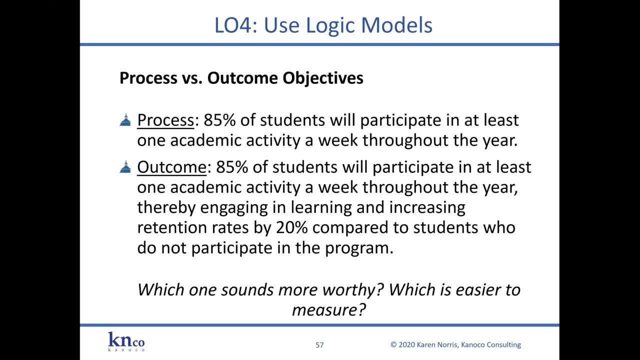 thereby engaging in learning and increasing retention rates by 20%, compared to students who do not participate in the program. so again, which one sounds more worthy and which one is easier to measure? you know, they're both kind of easy to measure because you've got 85%. 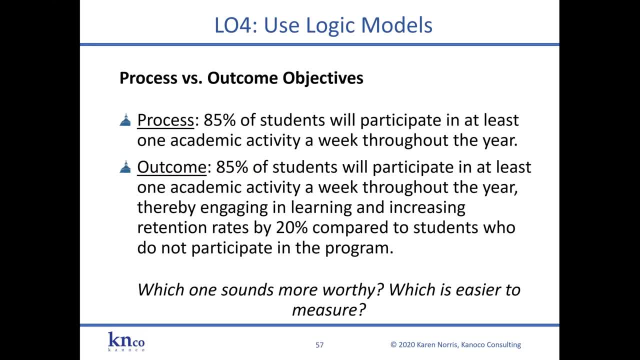 of students participating and they either are or they aren't participating in a weekly activity and it's going to be measured throughout the school year. but the difference is you, what's the What's the whole reason behind them participating in those academic activities? Why do you want them to participate in the academic activities? 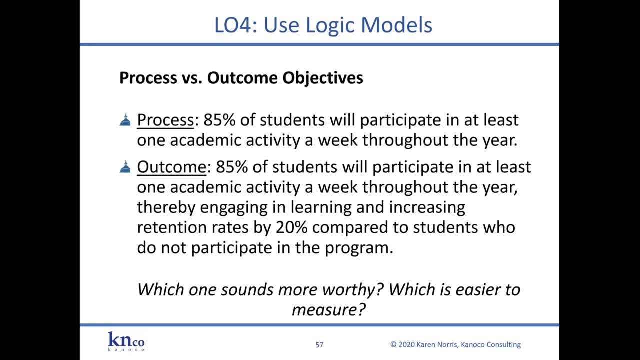 Well, we want them engaged in learning and we want to increase retention rates. We don't want them to drop by 20%. So now we have some data that we can measure and we're going to have comparative data: Students who are in the program compared to students who did not participate in the program. 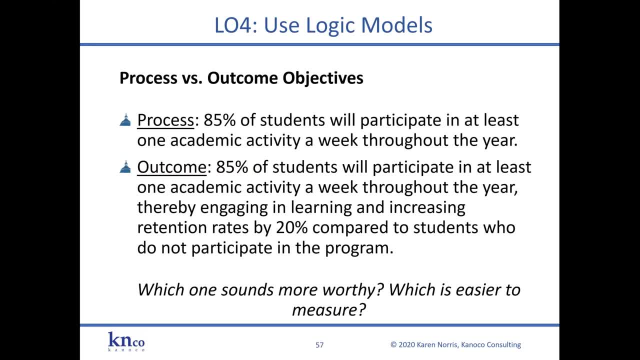 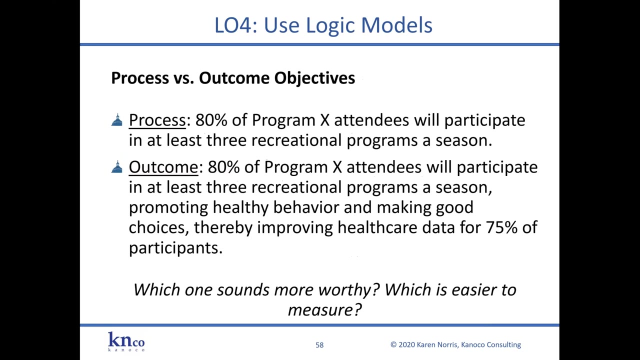 And where's the difference? So the second one is obviously a lot more easier to measure and it shows a reason for having them participate in the academic activity each week throughout the year. Why are they doing that? Here's another one: 80% of Program X attendees will participate in at least three recreational programs a season. 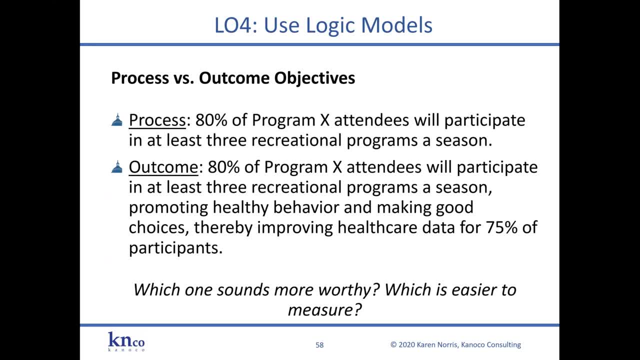 So, again, not bad. You know there are activities there, You've got a percentage of attendees, You've got – you're focused on recreational programs rather than academic programs and you're doing it in a – per season. So you know a lot of good – a lot of good information is included in that objective. 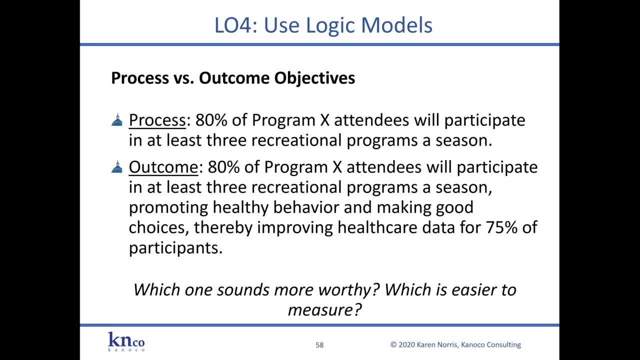 but let's look at the outcome. objective Starts the same but adds a few more – adds a punch to it. So 80% of Program X attendees will participate in at least three recreational programs a season, promoting healthy behavior and making good choices, thereby improving health. 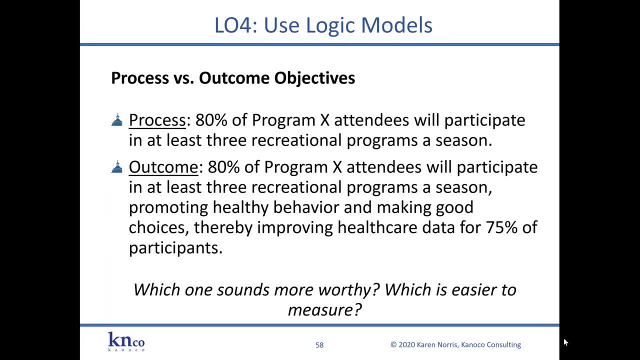 So again, not bad Health care data for 75% of participants. Yeah, we want them to lose weight. We want them to have healthy activities that they're engaged in during personal time. We want to see improved health care data. 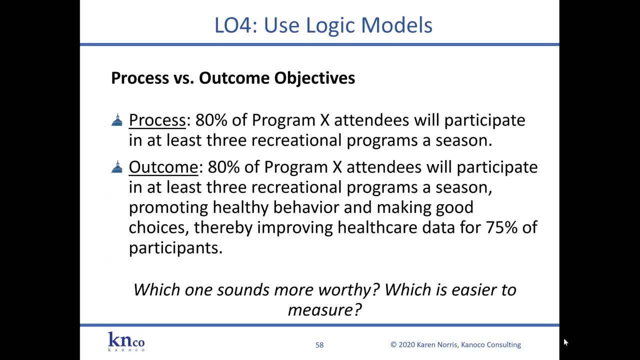 Maybe diabetes has reduced, Maybe weight has reduced, Maybe good eating habits have increased, Maybe you know the body weight mass – whatever it is that second – that second objective, the outcome objective, lets the reviewer know immediately, from the very beginning: this proposal these – this project is thinking in terms of healthy. 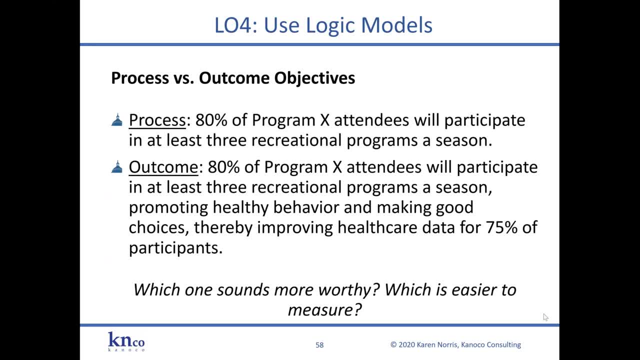 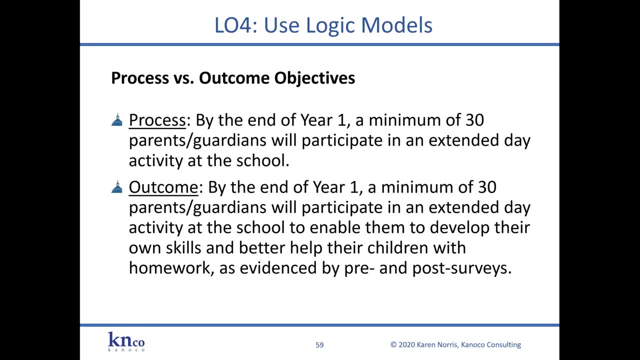 and good benefits from the very beginning, much more worthy of funding and easier to measure and makes for better valuations. Here's another one By – here's your process objective By the end of year one – so they're – they're your timeline for complete – completion. 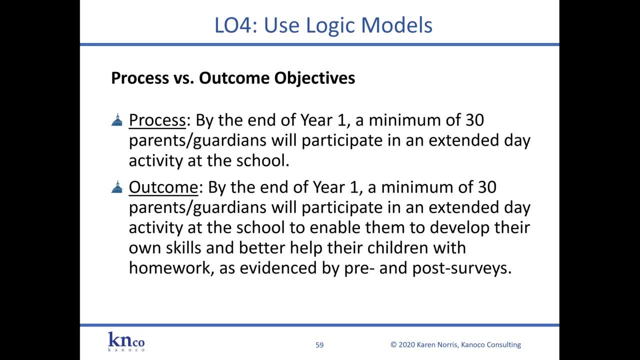 and this one is at the beginning – by the end of year one, a minimum of 30 parents or guardians will participate in an extended day activity at the school. Okay, that's pretty good, but their outputs, its activities, its numbers. 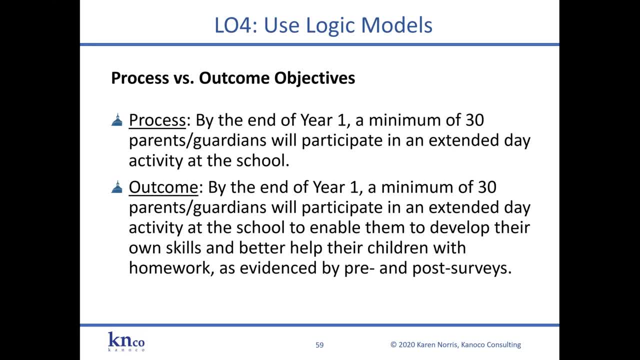 it's 30 parents and guardians and they're going to participate in an extended day activity at the school. The outcome objective would say, by the end of year one, a minimum of 30 parents or guardians will participate in an extended day activity at the school. 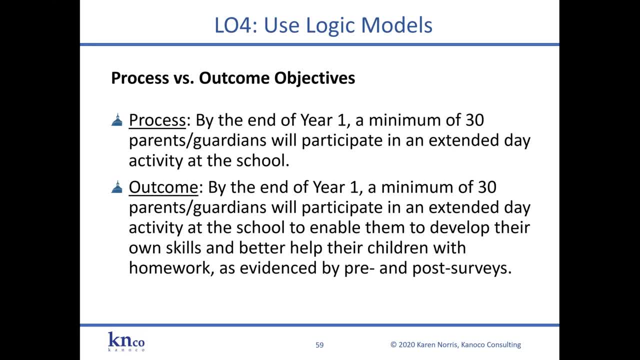 Why? To enable them to develop their own skills and better help their children with homework, as ever. So that's a good one, Okay. so the next slide is evidence by pre- and post-surveys. So there we have it. You're going to ask them how they feel about being able to help their students. 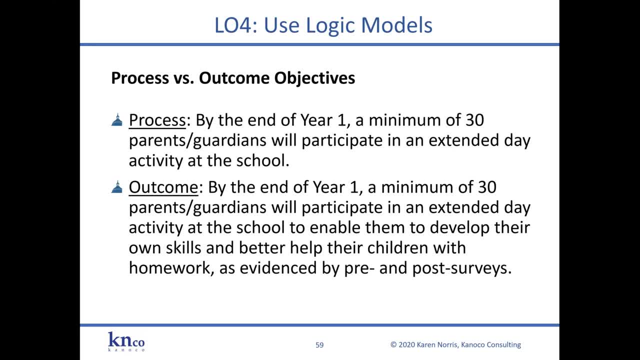 and do they understand the math? do they understand the – the language? maybe they're – they're immigrants. You know you're going to give them a pre- and a post-survey and by looking at the pre-survey you would better know what kind of activities to pre – present to them. 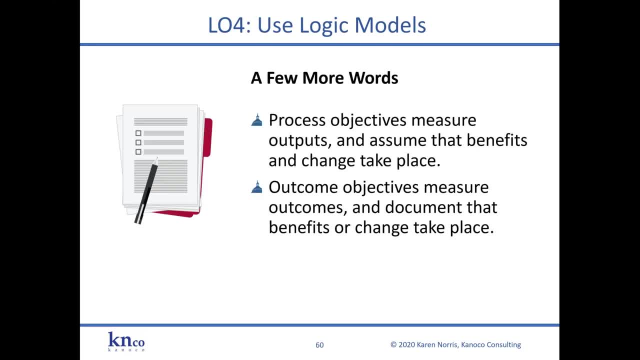 can address where the parent feels they're weakened. So process objectives: measure outputs and assume that benefits and change will take place. Not bad, but you can do better. Outcome objectives: measure outcomes, which is in the name of the objective, and they actually document that the benefits. 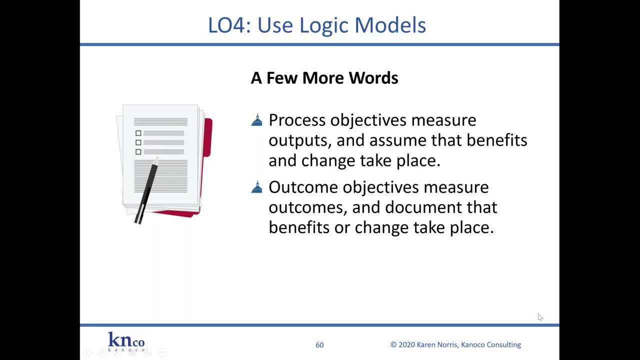 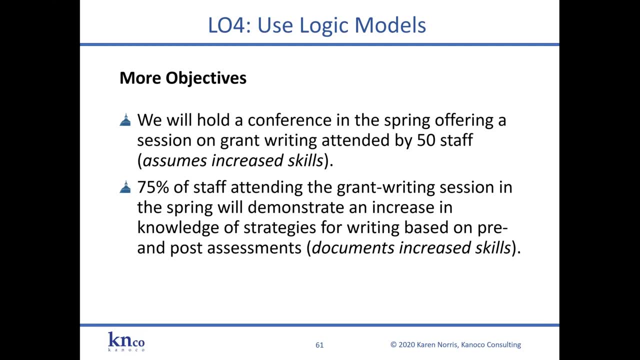 or change will take place. So here's some more examples. With that thought in mind, here's number one: your process objective. We will hold a conference in the spring offering a session on grant writing attended by 50 staff. Okay, great. 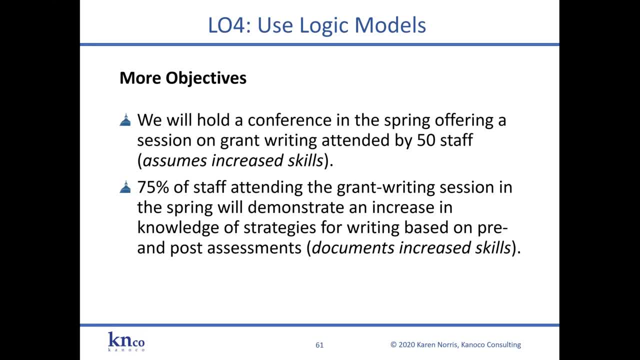 So you're assuming that staff needs to have increased skills, that they are interested in grant writing and they want to pursue grants to support their programs, and if they take this workshop, you're going to assume that they're going to learn something. 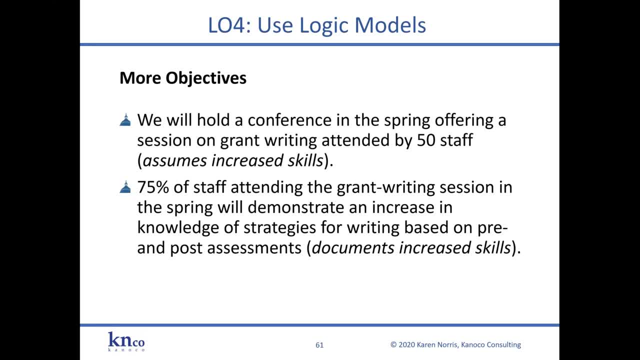 So here the second one says: 75 percent of staff attending the grant writing session in the spring will demonstrate an increase in knowledge of strategies for writing based on pre- and post-assessments. So now you know how many are actually attending. 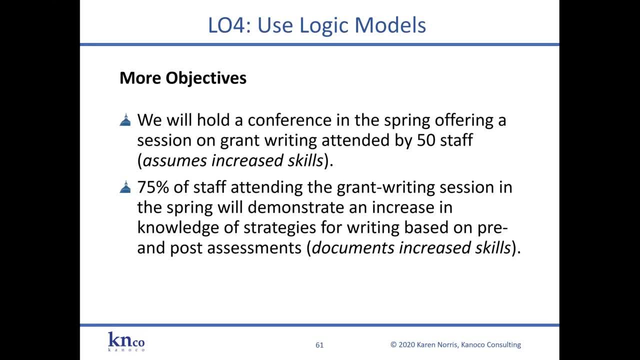 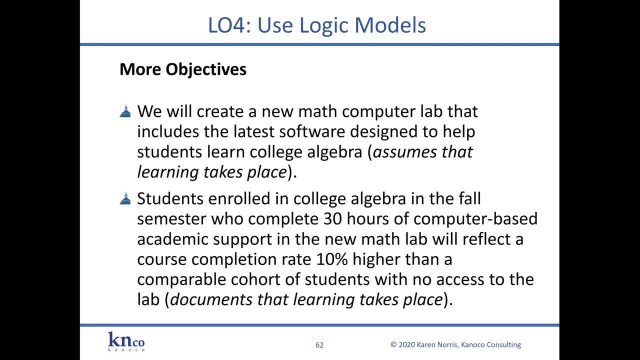 and you've got the timeline, but you're actually going to be able to document increased skills and increased learning. All right, so the first thing I want to do, I want to show you how to do this. So you're starting out just with an article. 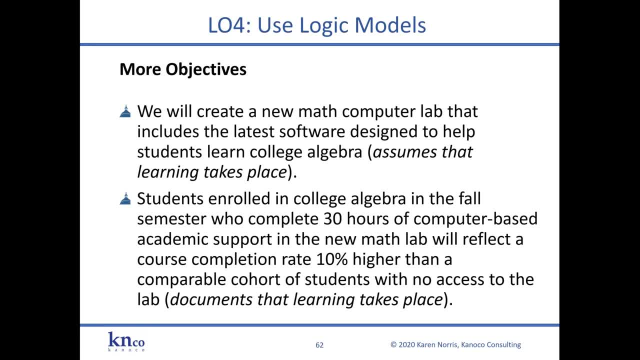 and I'm going to show you how to do it. So you'll see, here I'm going to go ahead and say I'm going to do this Now. I'm going to go ahead and continue on with my students until I'm going to get into the course. 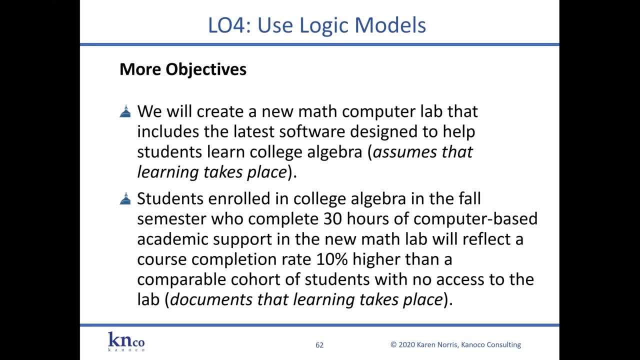 So I'm going to get into the course and I'm going to start with my students to see what they're going to do in the first. So I'm going to go ahead and do this to ponder. we will create a new math computer lab that includes the latest software designed to help. 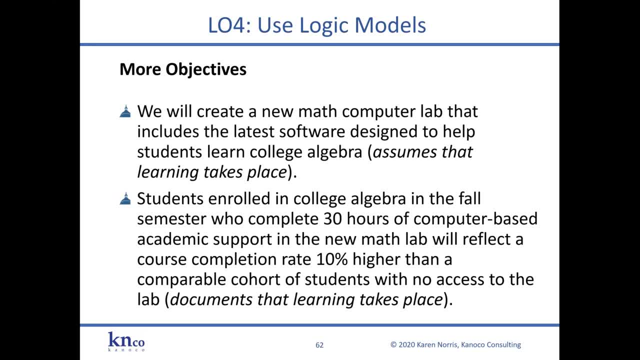 students learn college algebra. Again, this is assuming that the learning takes place. if they go to the math computer lab and if they use this software, you're going to assume that they're going to learn college algebra, but you don't really have a way to measure it, not, by the way. 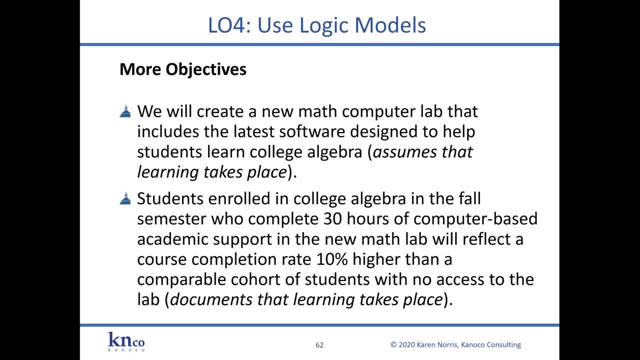 the objective is written. The second objective, on the other hand, says students enrolled in college algebra in the fall semester who complete 30 hours of computer-based academic support in the new math lab will reflect a course completion rate 10% higher than a comparable cohort of students with. 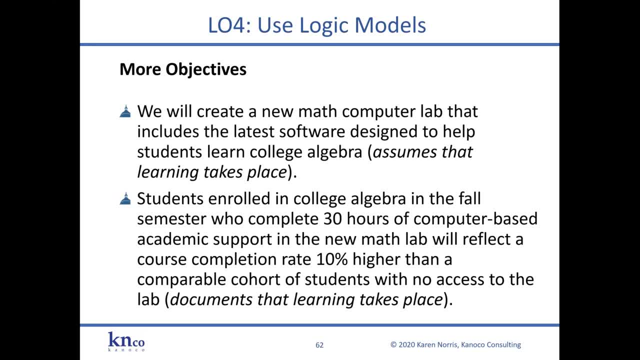 no access to the lab. So this way, you're actually documenting that learning takes place and if you exceed the 10% percent, well then wow, you're excelling, you know you're. you're not only meeting, you're exceeding expectations. that would make for a really nice progress report. 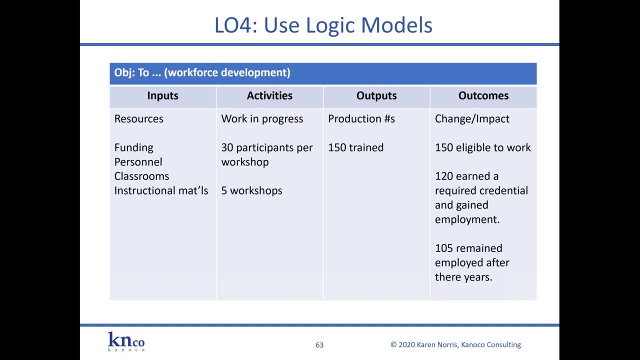 don't you think so? here let's use the logic model format and try to put some of this into giving you example based on the format. so here, if we would have the objective across the top, this would be an example for something to do with workforce development. so quickly skip over to the outcome column, which would 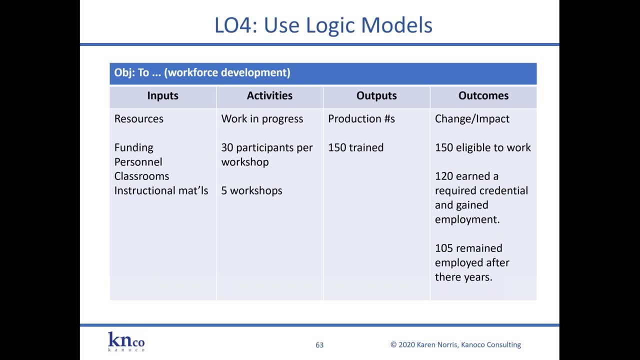 be your change of impact and you would look at some of the the possibilities that I put in the outcome column. you would write that objective that would lead you to whichever one of those outcomes you write, or maybe, according to your workforce development grant your you would have other outcomes that you're looking for, but you want to make sure that the objective 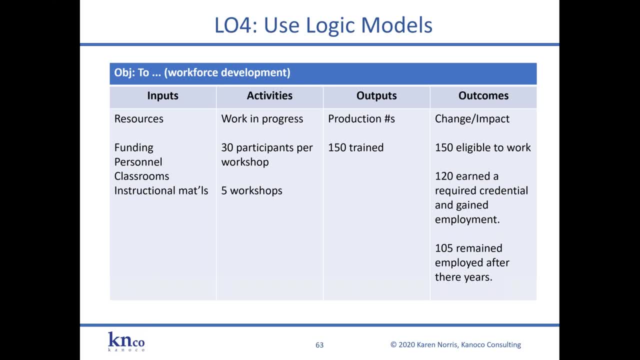 is going to lead you to the outcome column. so now the input column would be the funding, your personnel. who's involved? how many classrooms? if it's workforce development, there's probably some training. what types of instruction materials are you using? 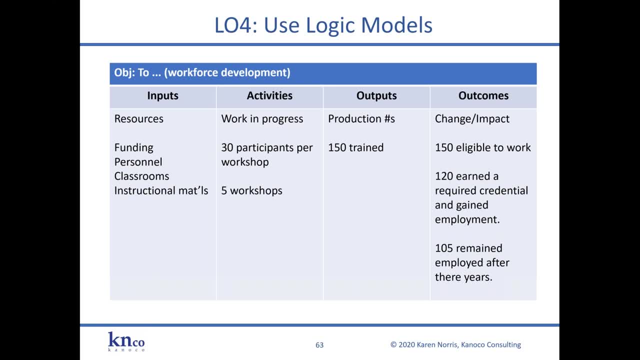 and then your activities are going to be: well, you're going to have workshops, and you're going to have five workshops and there are going to be 30 people in each workshop. so your production numbers, well, you're going to end up with 150 trained. okay, That's good, That's a lot of work. 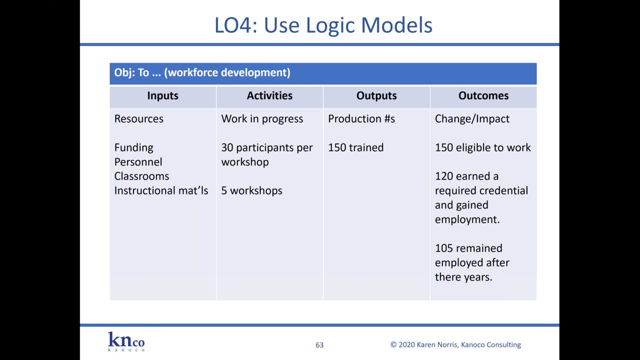 that's taken place. but what's the point? You know what is the point of their being trained So they're eligible to work, or they've earned a required credential and they gained employment, or 105 remained employed after. that should be three years. 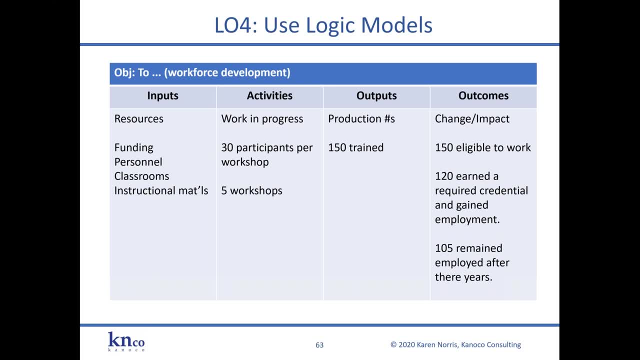 There's a typo there, sorry after three years- and you can get as evidence through HR records or something you know. Here's another example. so this has to do with parenting skills. so your resources would be your funding, your staff. you might have partners in this case. 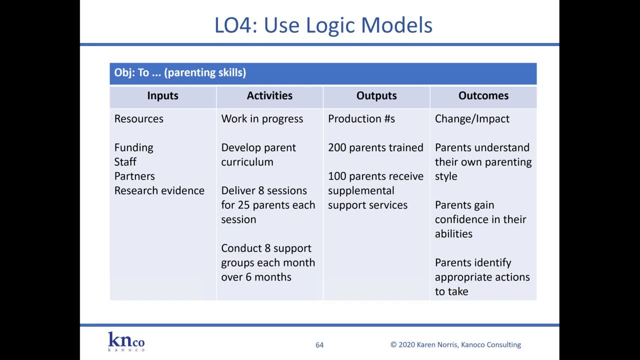 you might be basing the program on some evidence, some research evidence, and there would be literature citations. You know you're not just making up an idea, you're actually. you've done a literature search and you've identified some best practices that 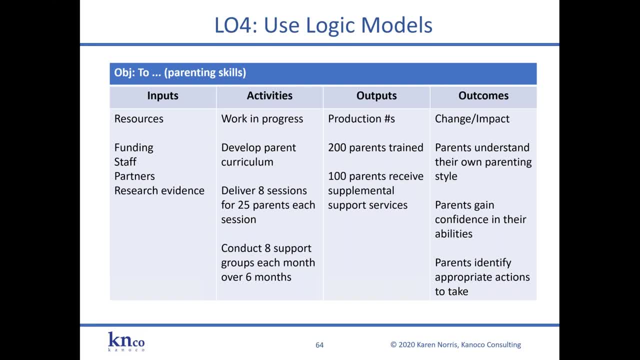 have shown to have good results nationally: Federal agencies, like programs and, I should say, pass-through entities also. everyone has pressure to perform, And what's the likelihood of successful performance? Well, if you've done your homework and you're designing a program based on a best practice or 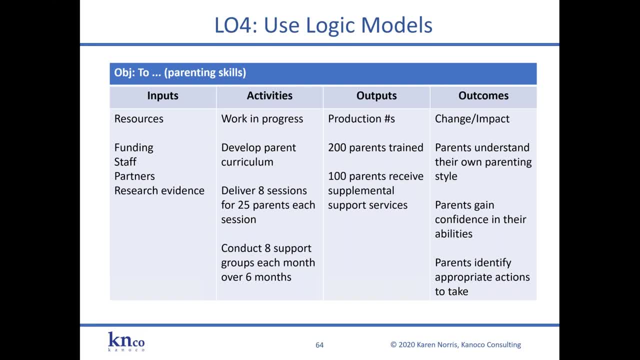 evidence and you have some citations. again, that raises the level of your project above other people who don't take the time to include that information. so that's a great input, that's a great resource. is to include something that's evidence-based, some literature citations and then the activities you're going to develop: a parent curriculum. 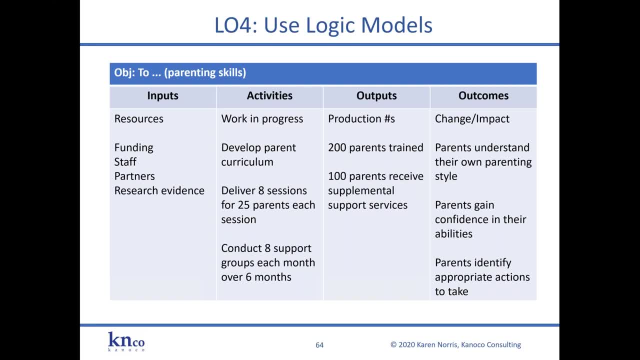 you're going to deliver eight sessions for 25 parents each session and, in addition, you're going to conduct eight support groups each month over six months. so these parents will be able to meet and and talk to each other about their experiences and, um again, and to share, to share. 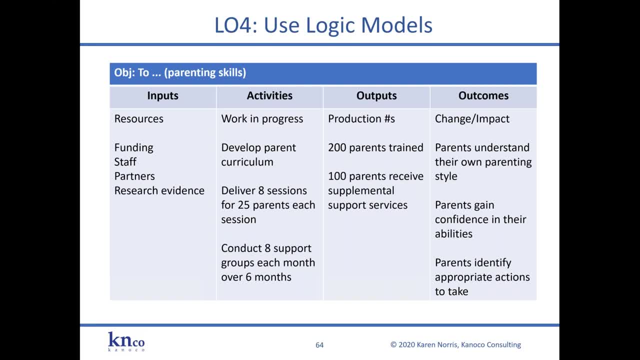 stories, so your outputs are well. you're going to have 200 and 200 parents trained, and that's a lot. 100 parents receive supplemental support services through these support groups. and what's the change or the impact? will parents understand their own parenting style? parents gain confidence. 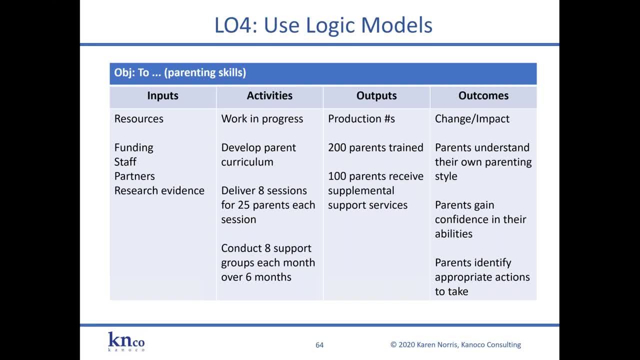 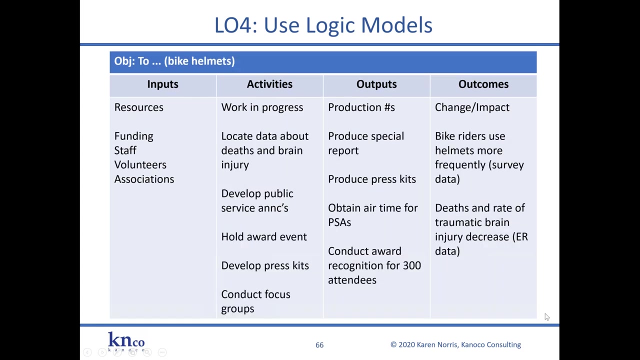 in their abilities and are therefore better able to help their children. parents identify appropriate actions to take, which is important- instead of just punitive actions. so this one gives you a lot of options for some very positive impacts and good coaching sessions throughout. so here's one that's: oh, we went forward, let's see if we can go backwards. 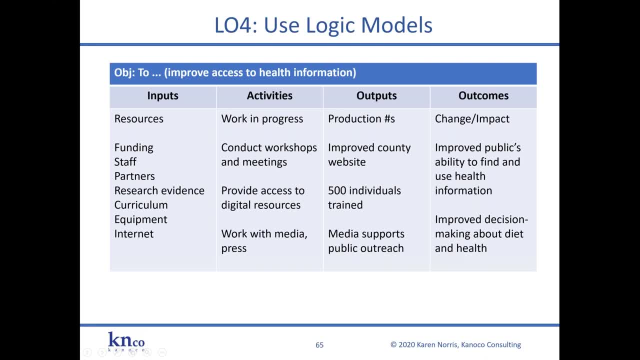 yay. so here's one about access to health information. so it's access to information, informational services. we're dealing with maybe the internet, a website, brochures. so the resources would be funding and staff. you might have expert partners, you might again, here's your research evidence. you want to make sure that the 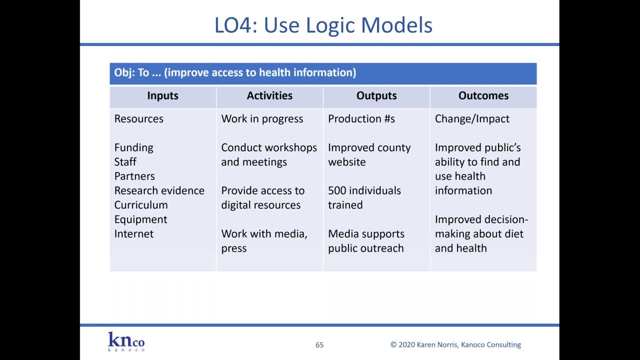 information you're going to communicate is based on sound practice. you'll have a curriculum, you're going to have equipment and you're going to need the internet, and then your activities are what you're going to conduct: workshops and meetings to come up with the appropriate, the best messages. you're 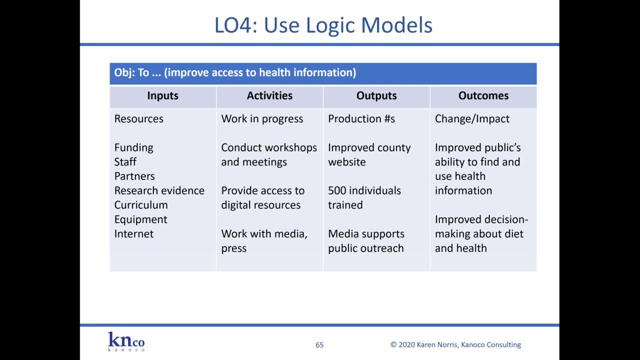 going to provide access to digital resources. and then you're going to work with the media and the press to let get to do, to perform public outreach, so people know, oh, there's a new website that I can go to for good information. and then your production numbers, your outputs, you're going to have an improved 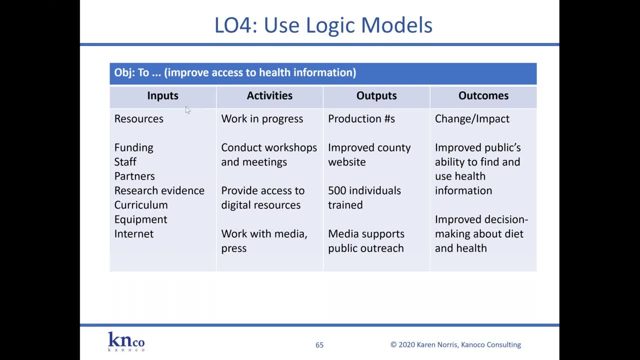 the county's website is going to be improved. you're going to have 500 individuals trained and then you're going to have the media: a media campaign which supports your public outreach and the change or the impact your outcome is going to be improved: public's ability to find and use health information. improve decision-making. 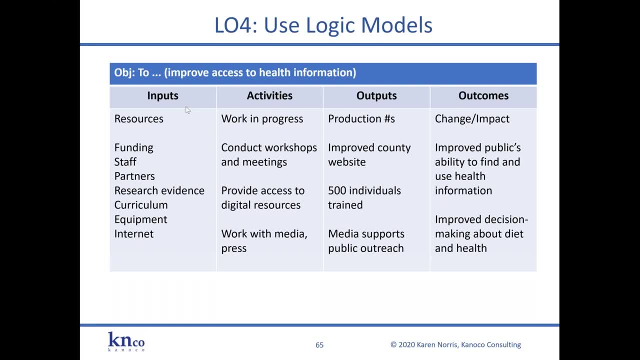 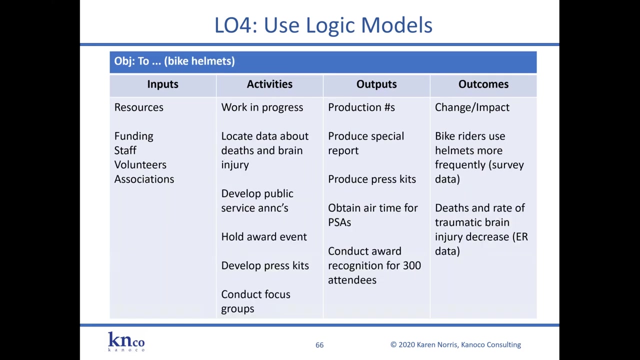 about diet and health, or safety, or COVID-19, you know, social distancing, whatever it is. this, this type of a logic model, this type of information or could, could, objective, could work well in a number of different grants. yay, so here's one for bike helmet safety and you've got funding and staff. maybe. 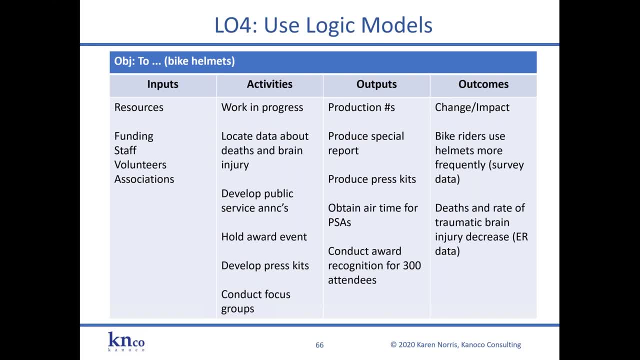 oh, you've got some volunteers here to help and maybe you're involving some health associations, some bike riding associations and safety safety associations, National Safety Council, the Red Cross, you know any number. the county, the county's recommended recommended County Department of Recreation, might have some recommended resources. so you're going to locate data about deaths and brain injury and that's. 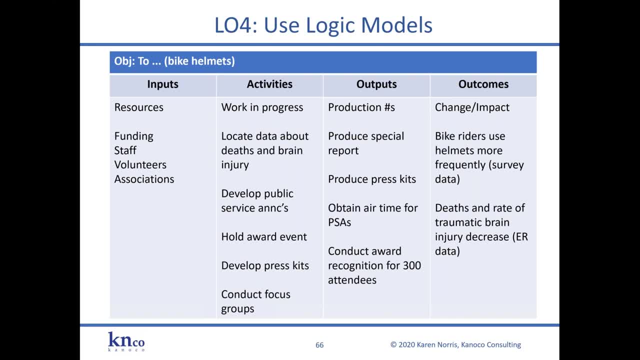 going to be part of the work in progress in order to have the best message as possible and to see how big is the extent of the problem. is there one area, area of the county, where it's worse than other areas? you know, now you're going to develop your 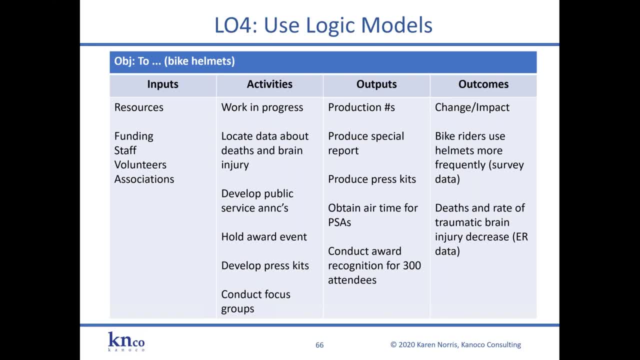 public service announcements based on this data and you're going to want to hold an award event for the volunteers and the associations who are get helping to get the work out and they're improving. you know they're getting more people to use spike helmets. you're going to develop press. 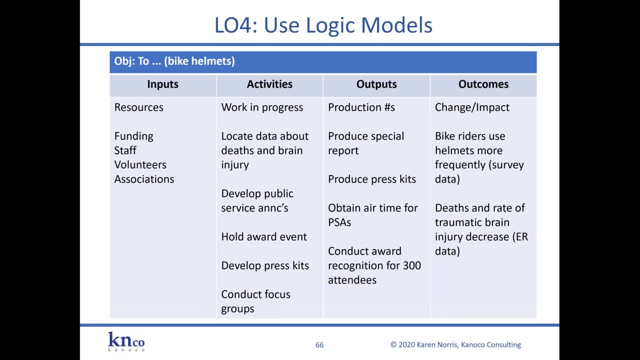 kits and you're going to conduct focus groups to help again with those messages and the outputs would be well, you're going to produce a special report, you're going to produce the press kit, you're going to obtain air time for the public service announcements and you're going to conduct 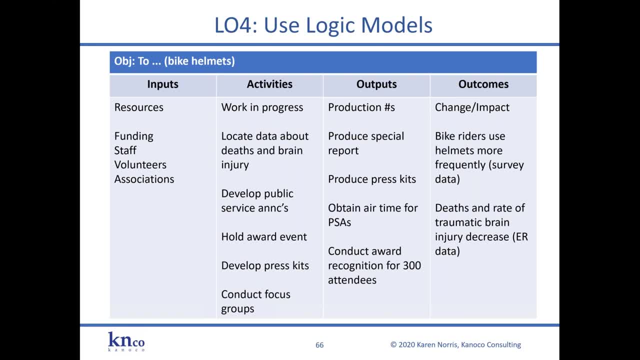 an award recognition ceremony for 300 attendees. you know providing, you know positive feedback for people who are, who are, who are taking steps for health and for safety, for for safe usage, parents encouraging their children, or any number of examples. and then the the outcomes, the positive change in the impact: bike riders use helmets more. 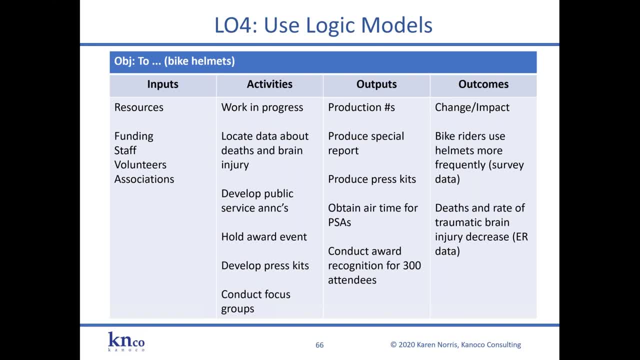 frequently and you can use survey data. the death rate, the deaths and the rate of traumatic brain injury decrease, and you could use emergency room data to to reflect that. so just think of the conversation and the thought processes that can happen when you have a well-written objective and you have a very organized method of presenting what's. 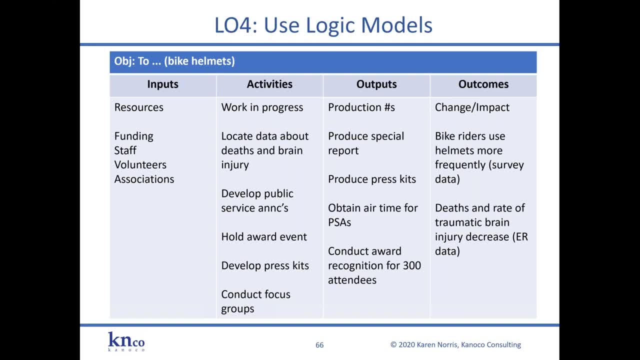 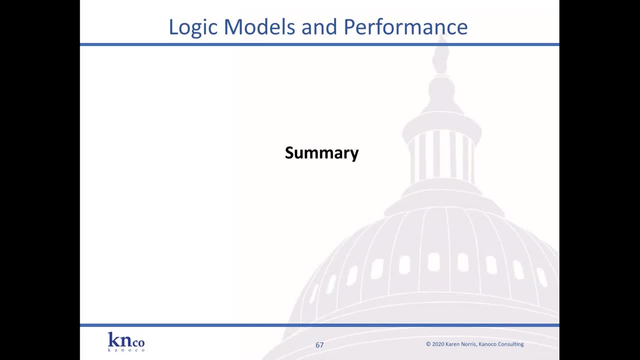 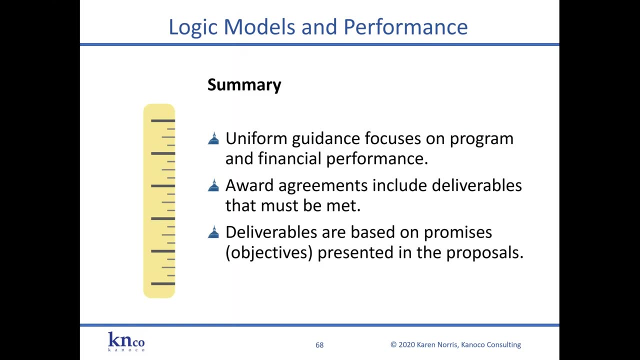 happening in your grant program. great, so let's let's recap. the uniform guidance focuses, excuse me, on program and financial performance, without a doubt, and the revisions of the uniform guidance are going to increase that language. they're going to have even more language about performance and results and the president's management agenda, as evidenced. 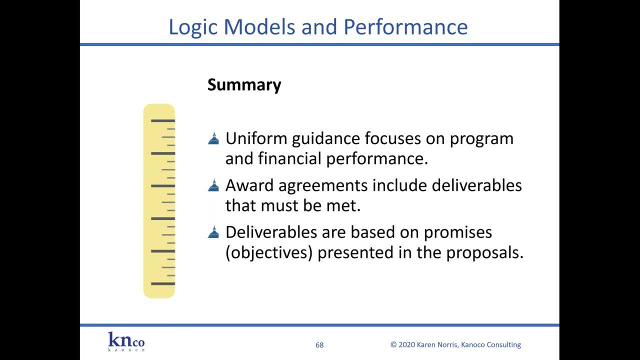 by its most recent report. is is very much focused on on management of performance and results, and everyone needs to comply with federal regulations, but they're raising the bar. not only must you comply, you also must perform and award. agreements must include deliverables that must be met, and those deliverables are usually drawn from the proposal that was. 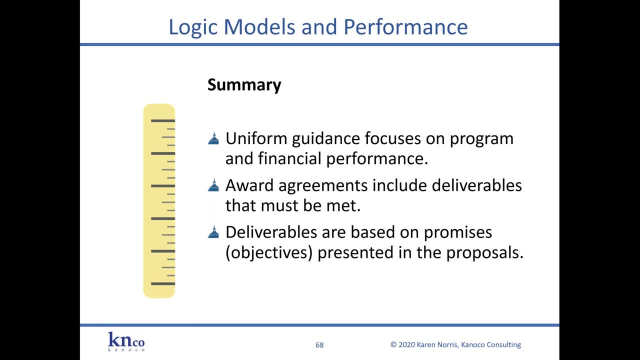 submitted and awarded and the stated objectives, the promised objectives that were in that proposal, become the deliverables in the award agreement. and again the deliverables are based on the objectives that were presented in the proposals and that award agreement is a legal document, so it does it, that award. 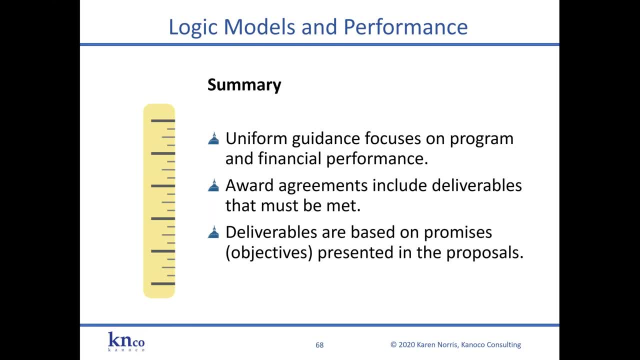 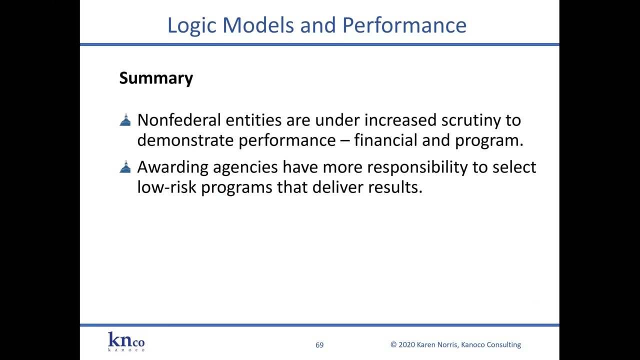 agreement is a is not a controversial to us and this is not having any impact on difficulty. the policies that we act as planning or the policies that the homage from the work that we hide of the relevant involves should be covered, and and all of these types of activities are still. 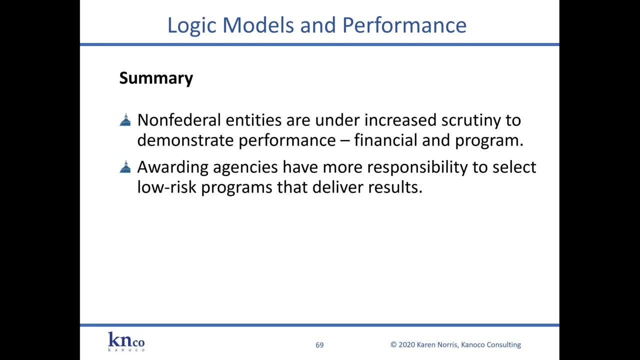 horizontal and that's because there are no diagrams in the channels that go to these. your performance and that logic model gives you a tool to present your performance. you know information, the cause-effect relationships. Awarding agencies have more responsibility to select low-risk programs that deliver results. so if your objectives 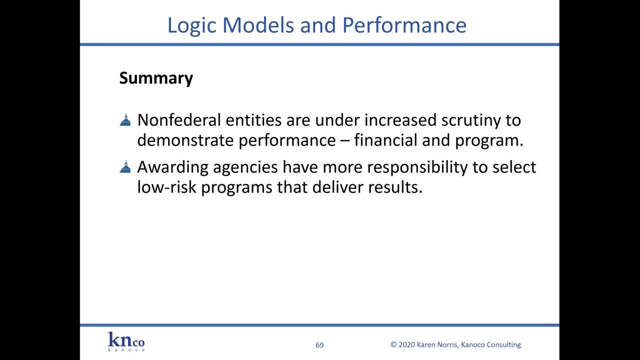 are well written in the proposal. number one: that increases your likelihood of receiving an award if you have a very worthy objective. that's measurable and it leads to an outcome that they know what they're doing. so not only does the objective help the proposal, but once you 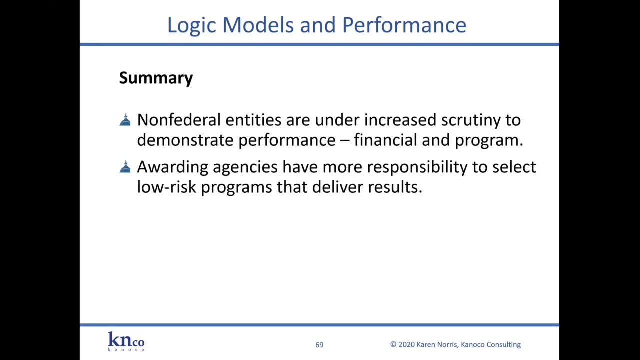 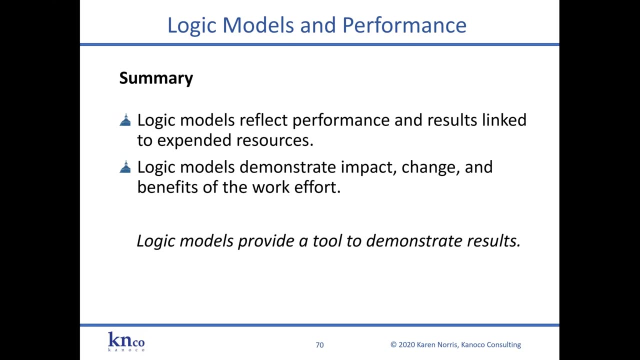 are awarded. that well-written objective is going to make your evaluation easy and it's going to make your evaluation easier to conduct. so logic models reflect performance and results that are linked to expended resources, and they demonstrate impact change and benefits of the work effort. so the logic model provides really just an excellent tool to demonstrate. 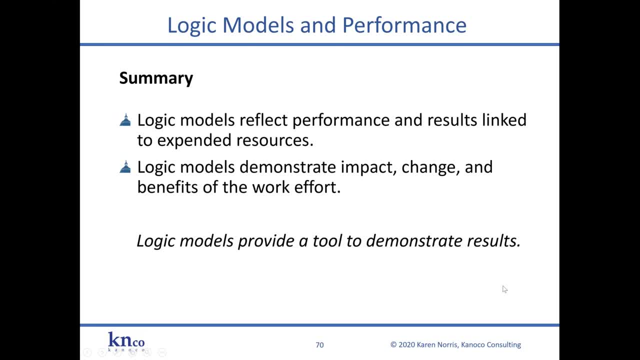 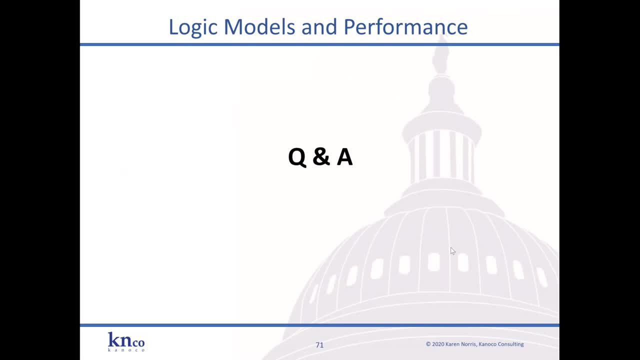 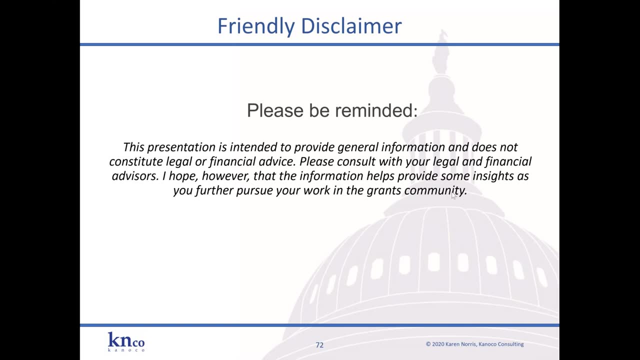 results. Any questions? Hey, yes, we do have a few unanswered questions here, so, and you might have touched on some of these in the presentation, but, sorry, let me just go back. so here it says outcomes such as reduced 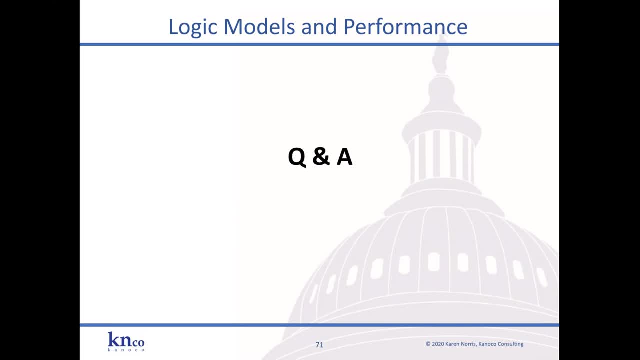 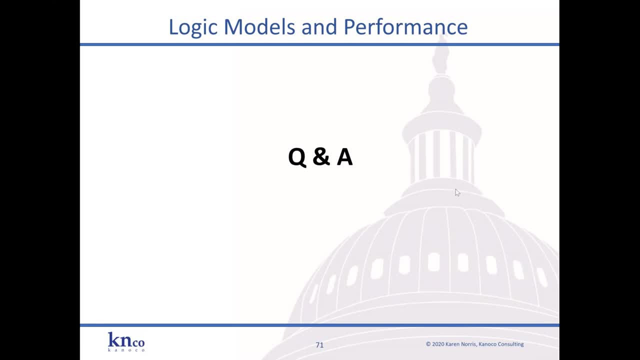 your objectives. choose your objectives wisely and you might have, let's say, an overall goal to reduce pedestrian deaths and under that goal of reducing pedestrian deaths, you have three different objectives: Pedestrians that don't cross at the corners they're crossing from. 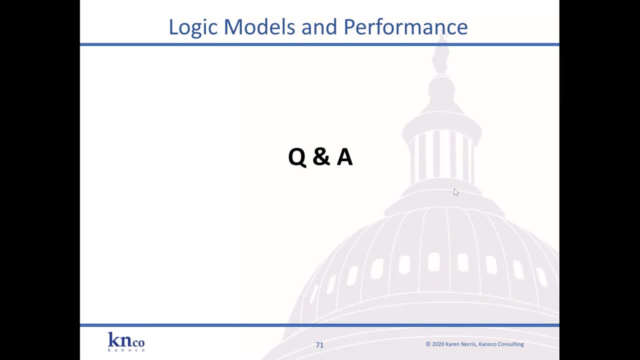 you know, mid, you know, outside of the crosswalk Pedestrians that motorists who don't attend to right away, or who run red lights, or you know you would divide it up for your multiple reasons and make each objective clean. so you're, you are addressing one piece of 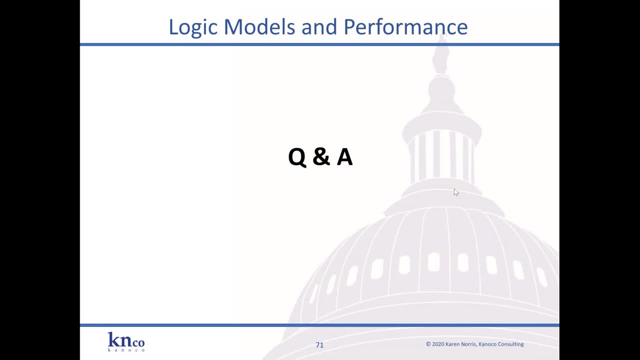 the puzzle at a time, and then what you want to do is you want to work toward an outcome, to change human behavior, which is really hard to do. but if you can get some of that articulated in that logic model, then you would have your short-term goals and then you could anticipate. 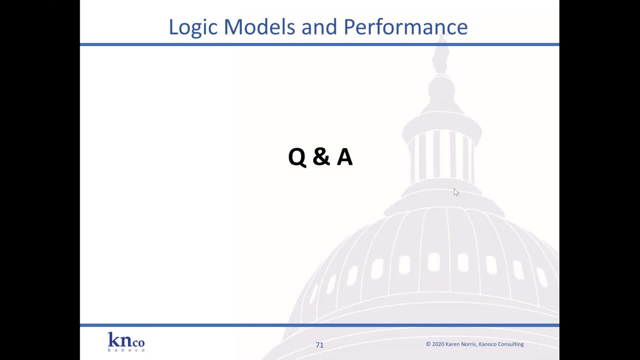 we will continue to the website. we will prove messages on the website and those will. the website will continue beyond termination of the grant period. We're going to. we have partnerships with the media outlets for free public service announcements and they will continue to to. 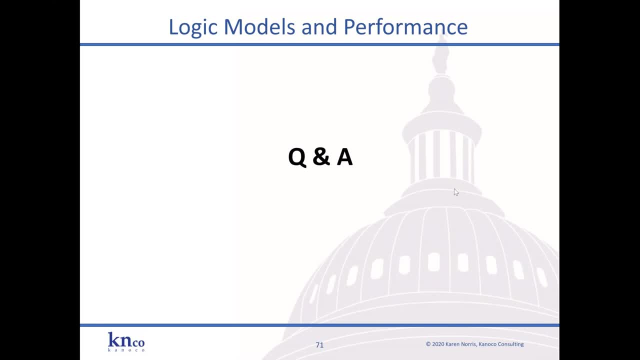 do to publish these public service announcements beyond termination of the grant period. So those are ways and you could have a partner. you know they're partners with us and we have a partner agreement where they will agree to do this, this and this. So hopefully that. 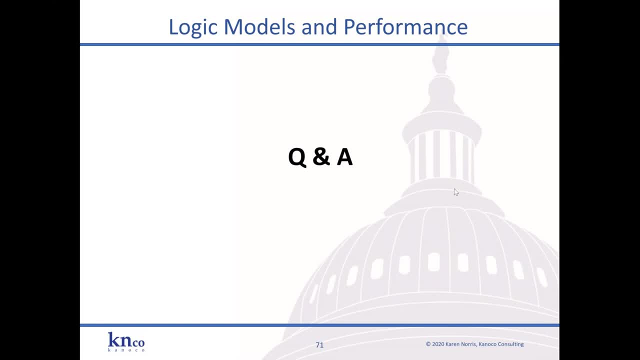 gives you some some thoughts. Is there another? Here's another. yeah, here's another great question. Is it ever required that a single activity is linked to outputs slash outcomes specific to that activity, Yeah. or is it okay where multiple activities yield multiple outputs and outcomes? 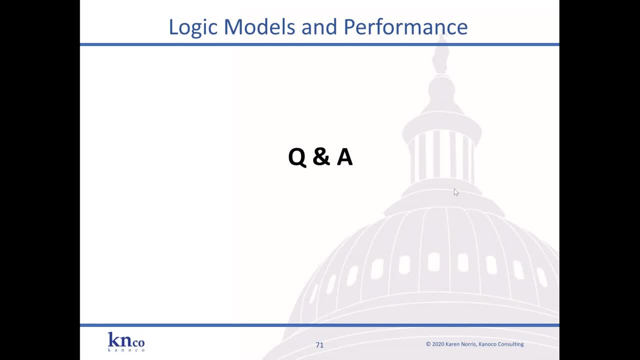 under a single objective. either one will work and either one can be presented in the logic model. just present them on different lines, but either one will work. okay, great. and if there's any other questions, people can fill those in in our the questions tab and we can answer those. but I think that looks like all of. 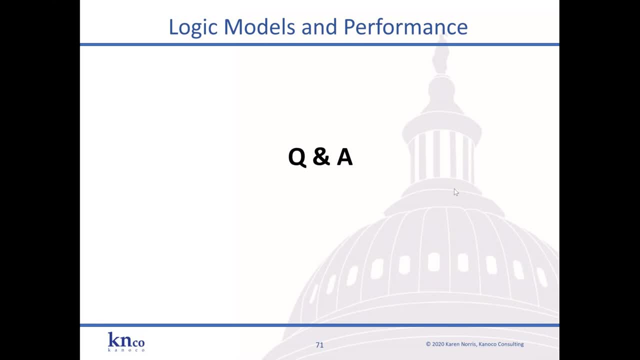 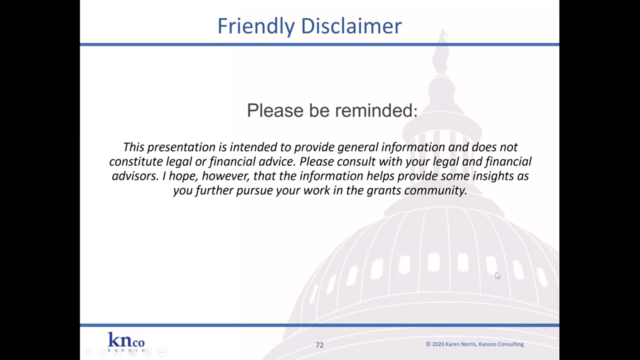 the questions for now, great, so let's continue. the view on my, let's see. so I would just like to remind you that this presentation is intended to provide general information, and I'm not. it doesn't constitute legal or financial advice, you know. in those cases, consult with your legal. 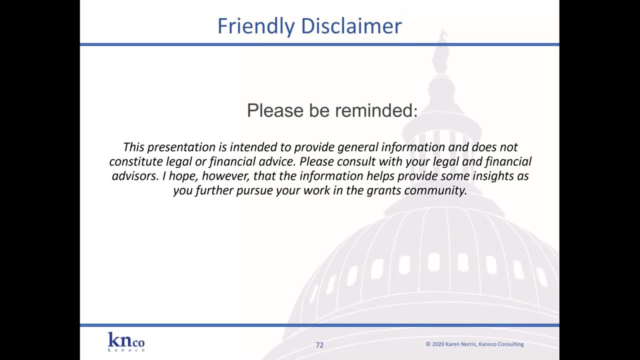 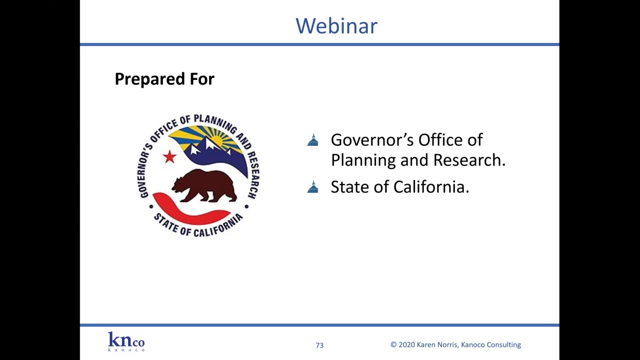 information- and I'm not- it doesn't constitute legal or financial advice, you know, in those cases, consult with your legal information financial advisors. however, I sincerely and truly hope that the information helps provide some insights as you further pursue, pursue your work in the grants community. and this was webinar, was prepared, prepared for the 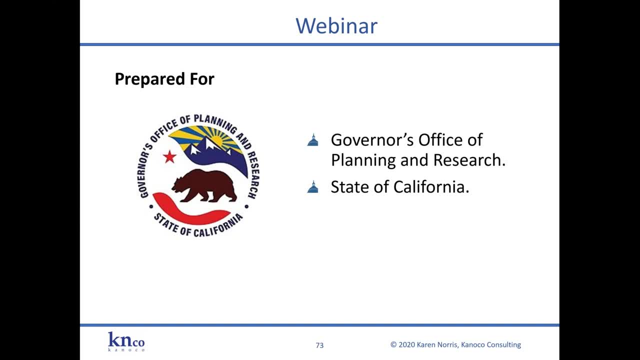 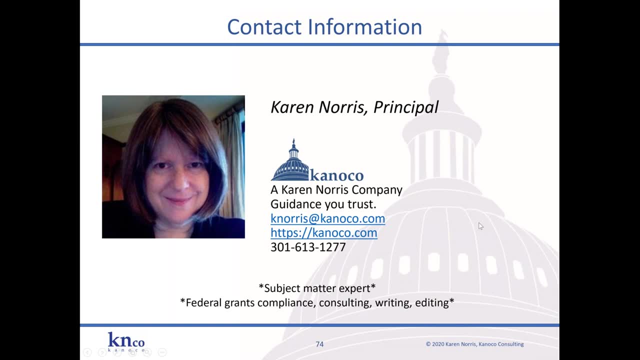 governor's office of planning and research for the state of California and it was prepared by me, Karen Norris, and there is my contact information so that if you go back and you review it and you have another question that comes to mind after the fact, you have a way you can email me and 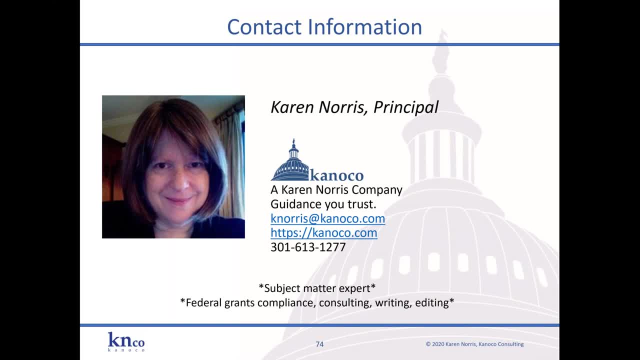 I will make sure that any questions that I receive will be shared with Amy and she can post them for everybody to read you know in in her website. and I think with that that'll conclude our presentation against a positive feedback from the board and I'll see you next time. 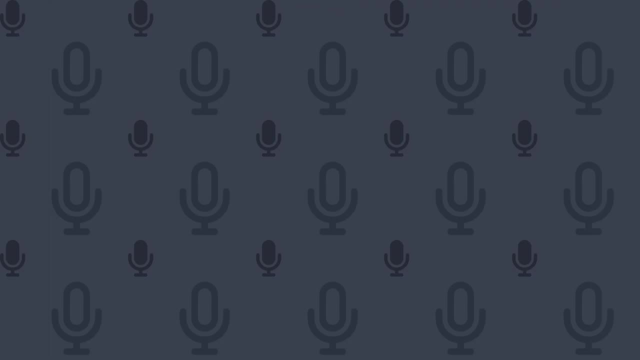 Amy, thank you for being so kind and giving us a lot of tiredness. Thanks everyone for the interruptions there. apparently, the teams App does not follow the other notifications being turned off, but so thanks Karen for forging through with that. I hope everyone survive the earthquake healthy, and so, again, we'll be sending an email tomorrow, please. 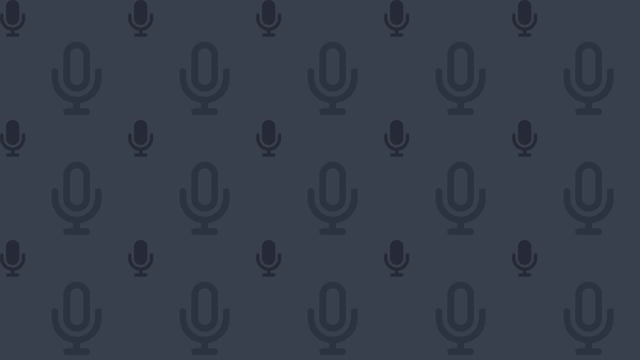 look out for that. it will include a link to a survey that we hope everyone can take, as well as the link to the YouTube page, and then the slides will be on the federal grant resources page. Thank you for joining us. So, again, please feel free to respond with any other comments or questions, and look forward. to seeing you at our next webinar in August. Thanks,